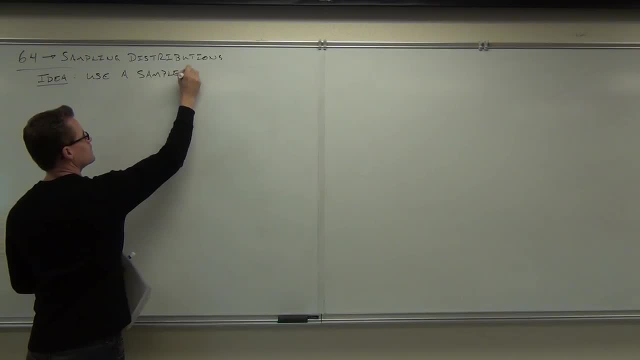 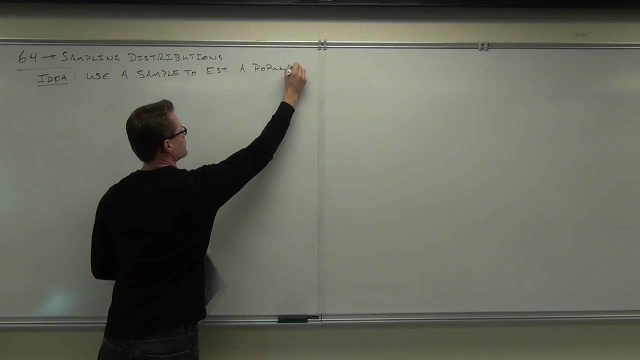 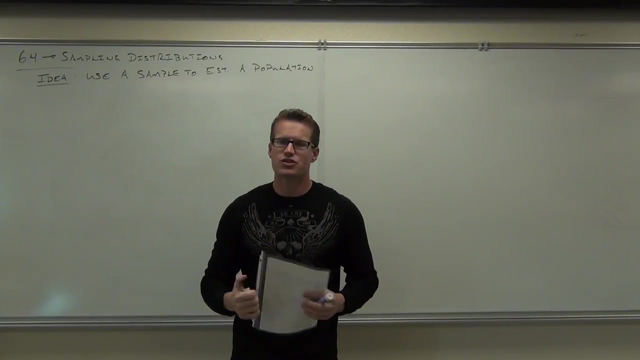 use a sample to estimate a population, And of course we're talking about specific characteristics of those things. You see, it's not just good enough to say, oh, I'm pretty sure this sample is going to represent this population, Yeah, let's go for it. You can't do that without a whole lot of legwork, And this is 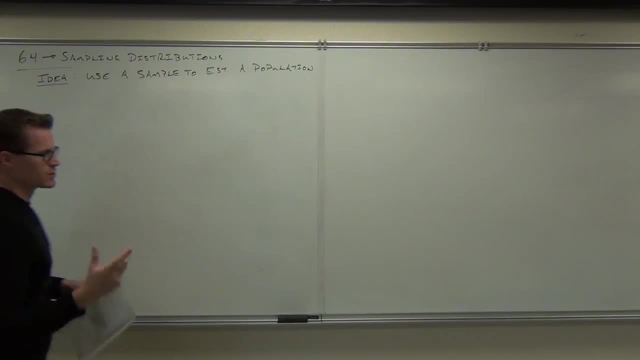 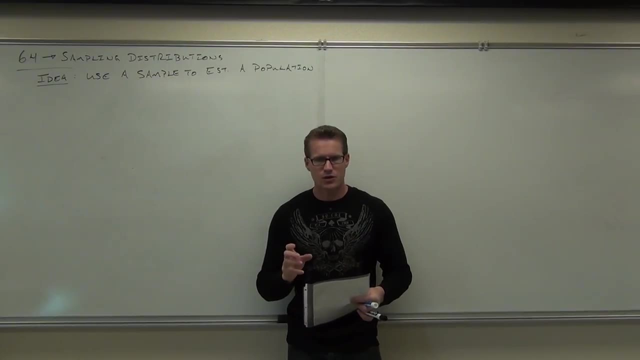 the legwork for that. So the first thing I need to notice is that if we're dealing with a population of people or population of anything, then if we're going to take a sample, we're going to have to do something about it. If we're going to take a sample from that, there's a whole lot of possible. 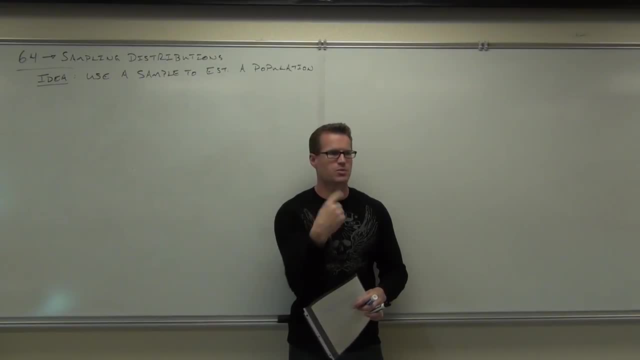 samples we could take, right. Right, Let's say: this is your population. This classroom is all the people that exist in the world. That'd be freaky. We don't know each other really well, I'm sure. But let's say that this was the population. OK, And I said I want to pick. 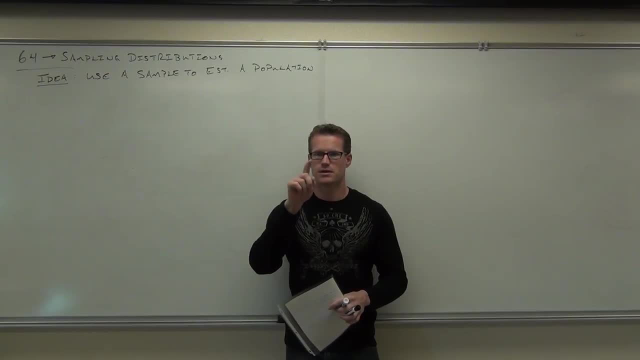 out a sample of five people. How many people? It's 1,, 2,, 3,, 4,, 5,, 6,, 7,, 8,, 9,, 10.. There's 27 of you. Let's see, I'm wondering if I'm right. I just randomly guessed that. So there's 27 of you. 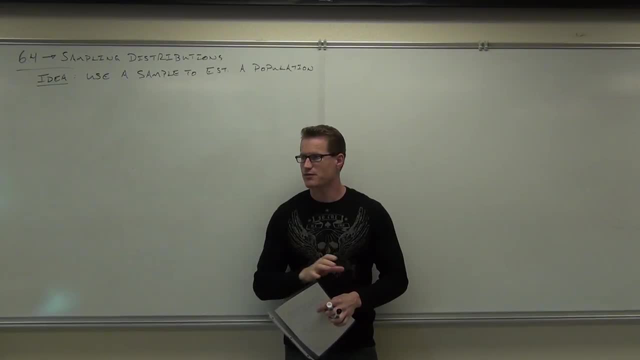 Let's pretend that there's only 27 people in the whole world. You, 27 people, you're the chosen ones, right, And I'm going to pick out samples of five, because I don't want to deal with all 27 of you. 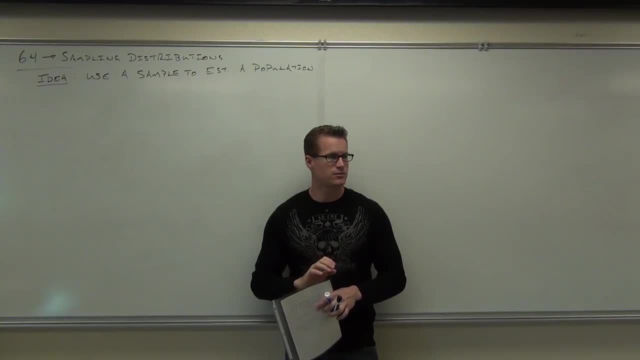 samples of five. Is there more than one possible sample of five? Well, I could pick you five. I could pick you five. That's two different samples. right, I could pick you five. I could pick all four of you, and then her instead of you at the very end. That's a different sample. 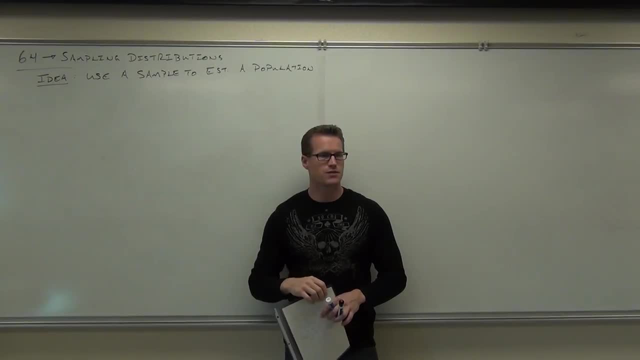 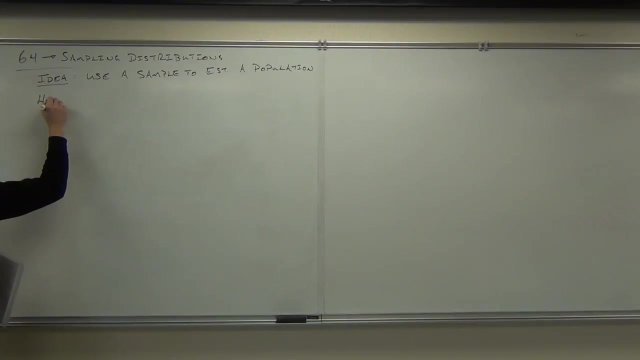 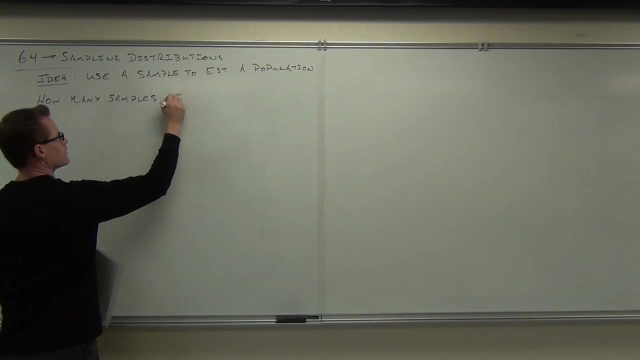 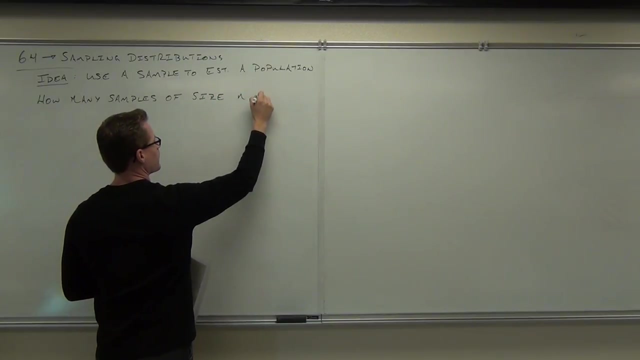 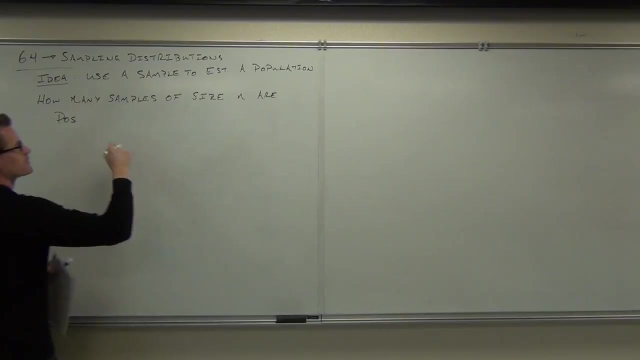 of five, isn't it? Even though those four are the same, that one's the same, Different. Are there lots of different samples in this classroom of five people? Yes, How many? A lot. Specifically how many. I'm going to change this, I'll leave it Sorry. 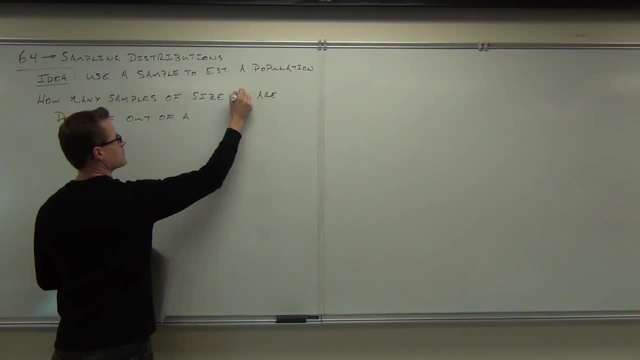 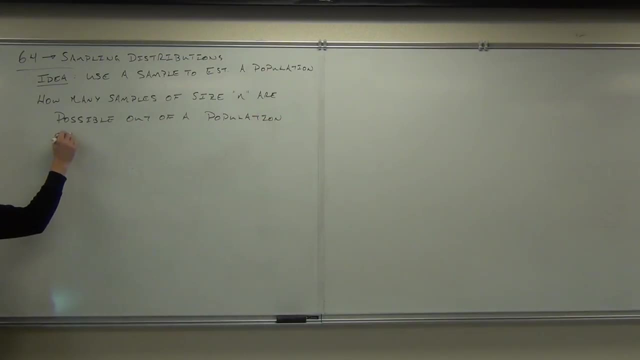 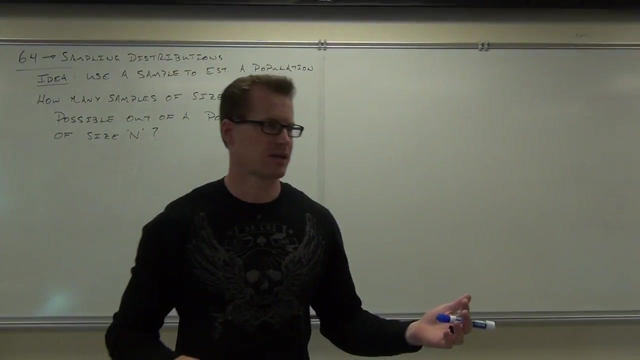 Notice how I used low, low Lowercase letter N for a sample, uppercase letter N for a population. Hopefully you remember that from like our first couple days of class. Do you remember that from our first couple days of class? 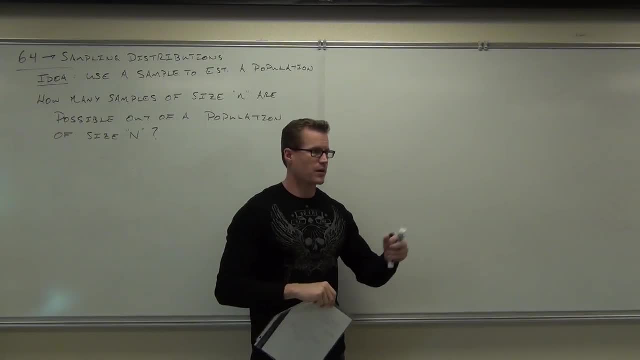 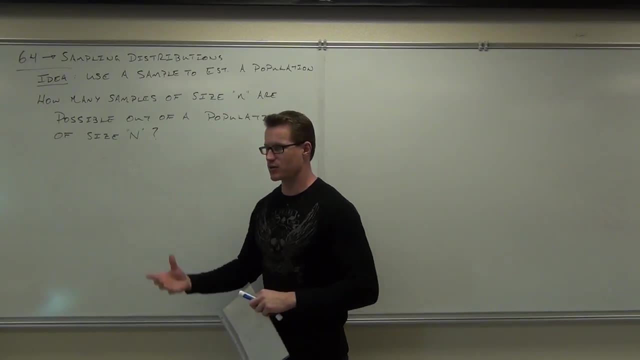 Good. How many samples of size N are there possible out of a population of size N? And I just said N twice, So if you're not reading it, you're not gonna know what I'm talking about. So how many of this size N samples? 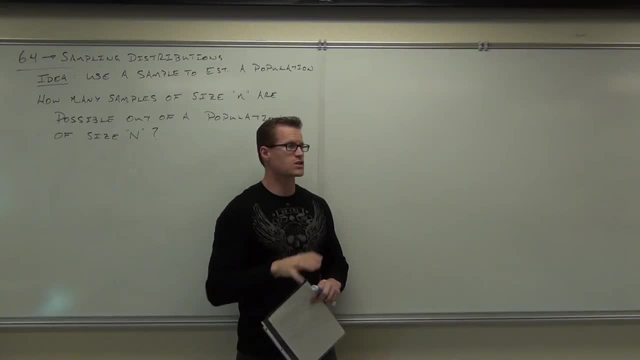 are there out of size N Shall we count. I just used this example. There's 27 people in the class. There's probably a little more now since we had some late people coming in, But let's say there's 27 people. 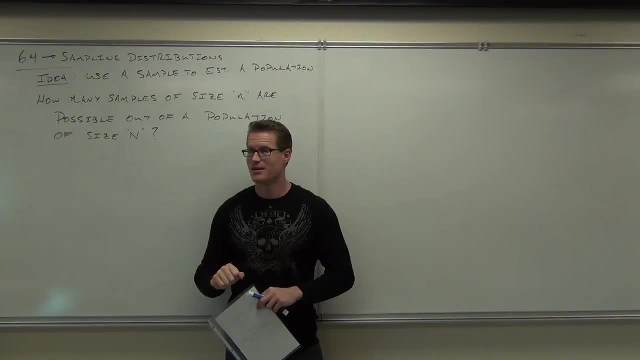 and I'm picking samples of size five. Shall we count them. Let's try it. Otherwise you need a better way to do it. So you stop me until you figure out a better way. Here's one. You five, that's one. 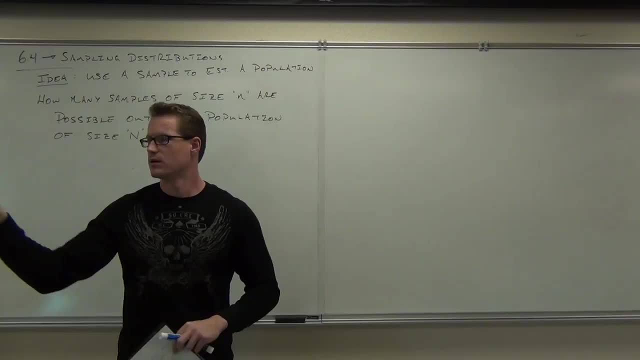 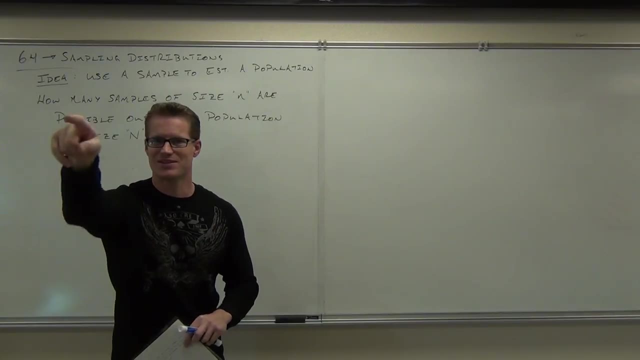 There's two, There's three, There's four, There's five, There's six, There's seven, Just let me keep going. There's eight, There's these four, and there's nine, These four and there's 10.. 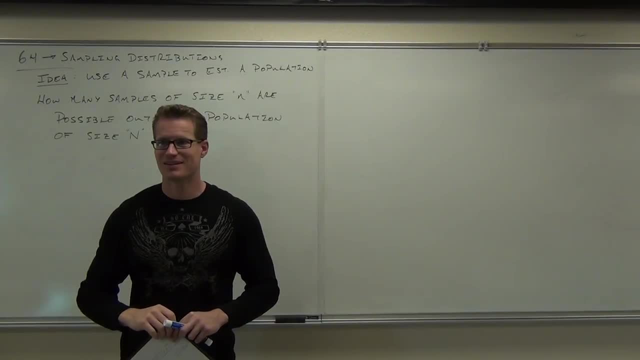 I'm gonna make you do it in a minute. Okay, Do you wanna do that? You'll be here for the rest of your life. There's like 80,000, 780,000.. You just did that that quick. That's amazing. 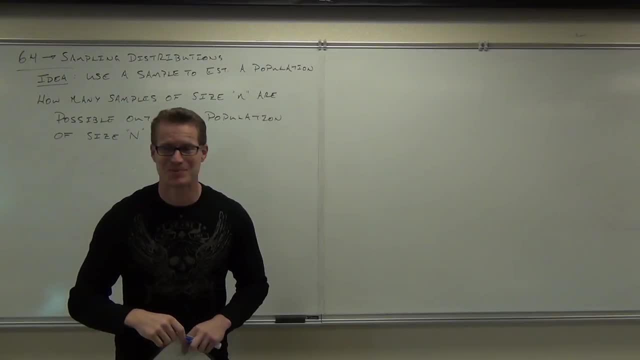 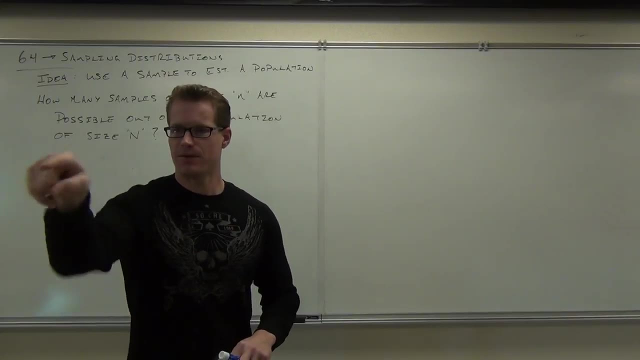 You fast counted. That's pretty good. One more question. Let's say that this is my sample of five people. Let's say I picked her out, then her out, then him out, then her out, then her out. Would it be different if I picked him out first? 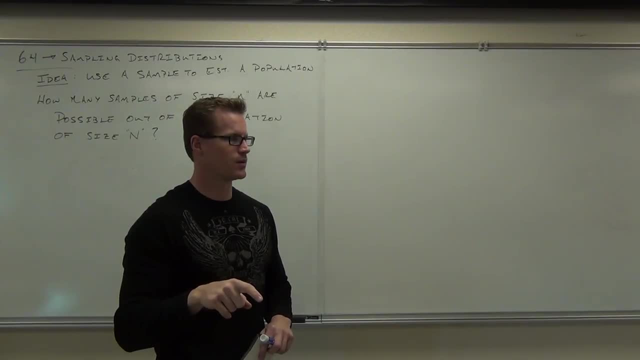 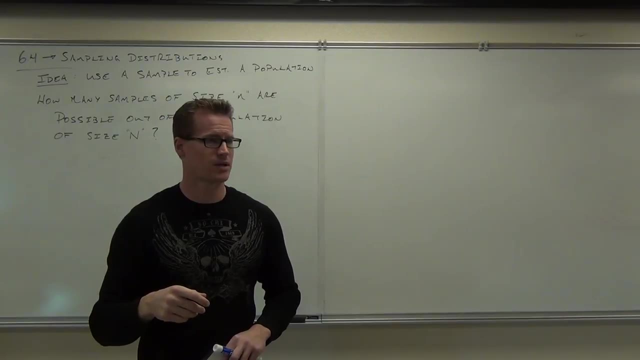 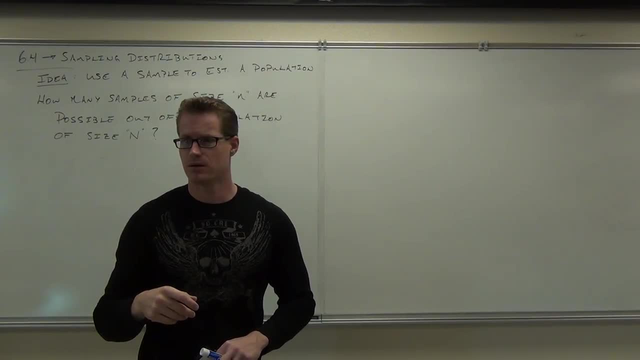 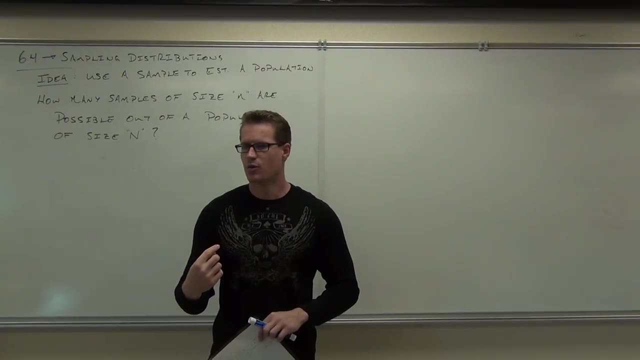 No, Does order matter or does order not matter? Order doesn't matter. Do you see where I'm going with this? How many people are in your class for this experiment? 27.. We're picking out samples of size five, right? 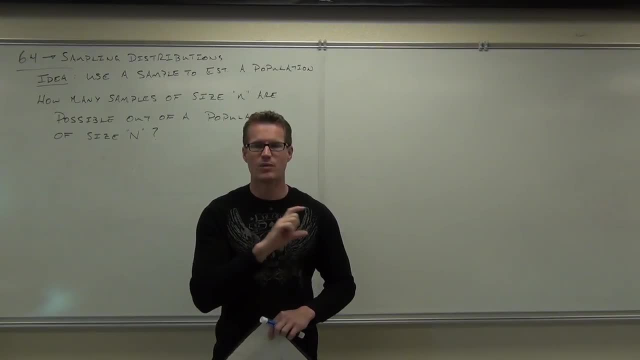 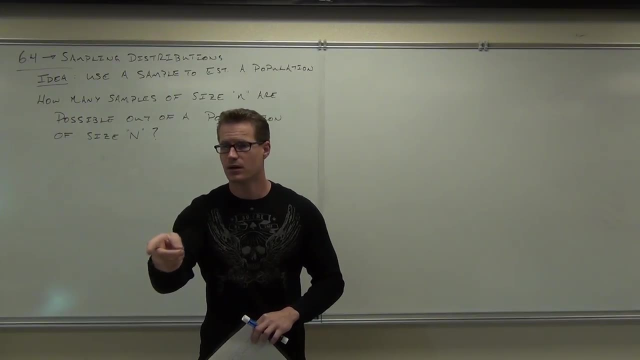 We want. there's 27 people. let's have a size five. How many possible ways can you do that where the order doesn't matter? What are we talking about? A combination, Say it louder: A combination, Why not a permutation? 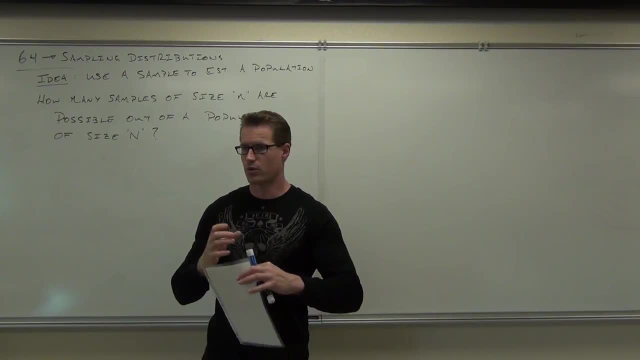 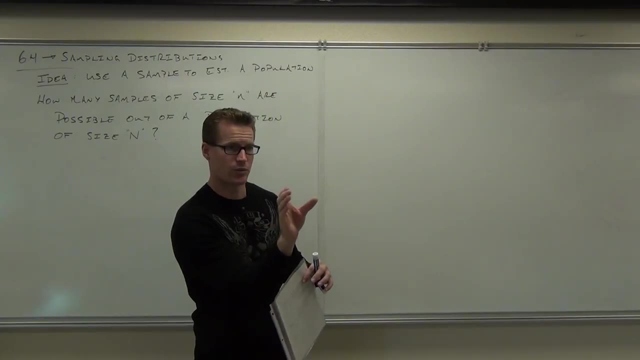 A permutation, Every one of them. that would be exact. That would be the order would matter then. However, for a sample, the order in which you pick it out doesn't matter, as long as you get the same quantity or the same exact people, no matter which way. 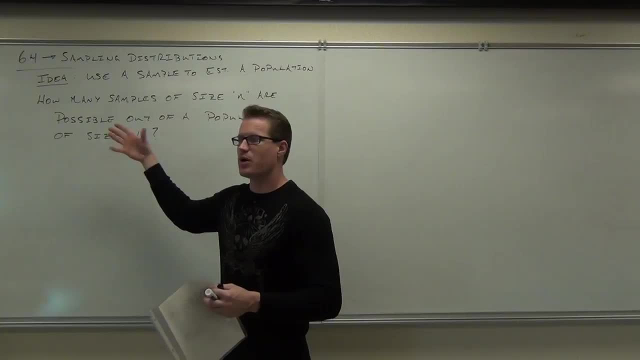 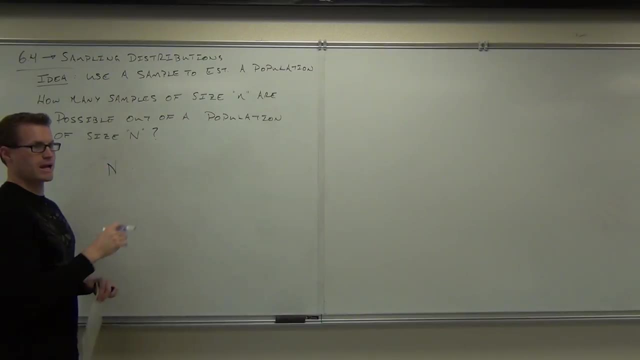 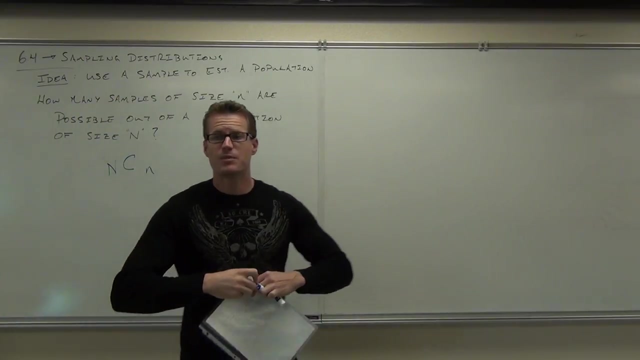 You with me on that. So we're dealing with a combination. So how many possible samples are there? if you have N people or N items in a population and you want N of them, It's a combination. It's a combination. That's how many possible samples there are. 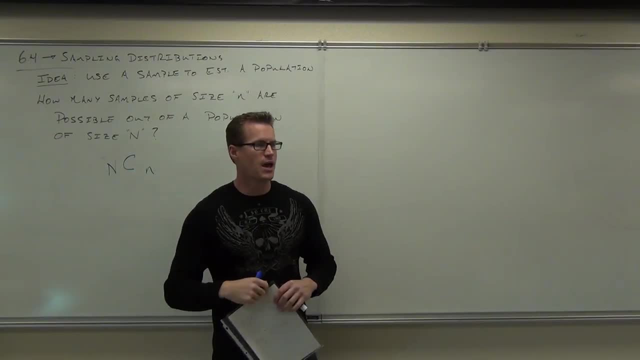 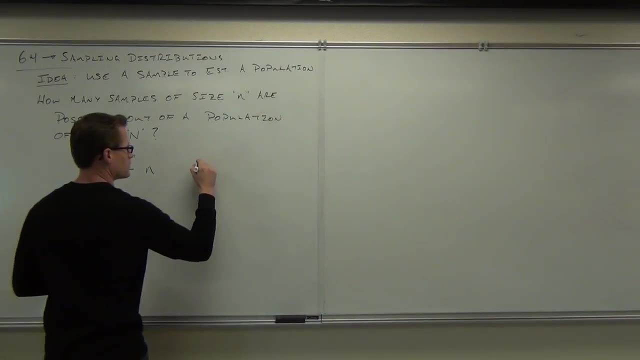 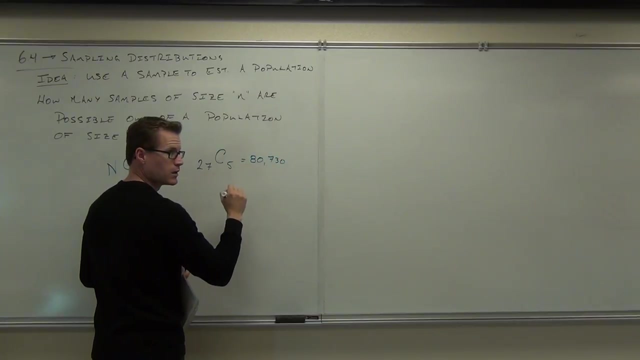 If we have 27 people in the classroom and we want samples of size five, say that again. How much was it? 80,730.. Like that. That's what you did If we did this in this classroom and I picked out samples. 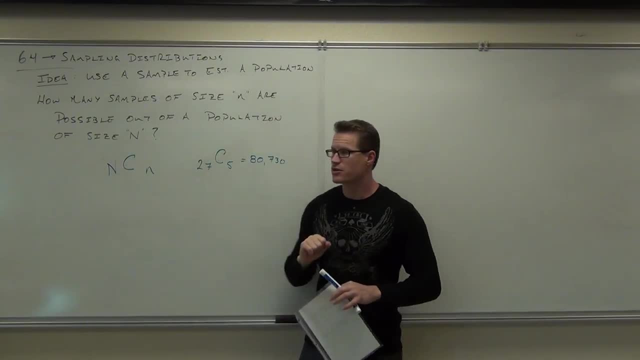 of size five. there would be 80,000.. That's what you would do: You would take all of them, you would put them in a collection: 730 different samples of size five, with just this class. How many of you want to show that? 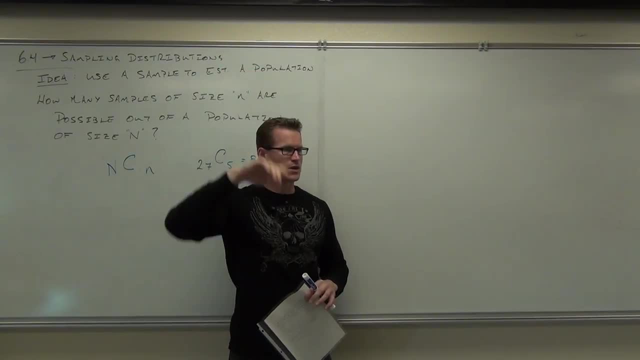 Do you want to take all of them? Do you want to actually do that? Because to accurately represent a population, you either have to take every possible sample or you'd have to use this theory stuff that I'm about to show you. Are you ready to learn it? 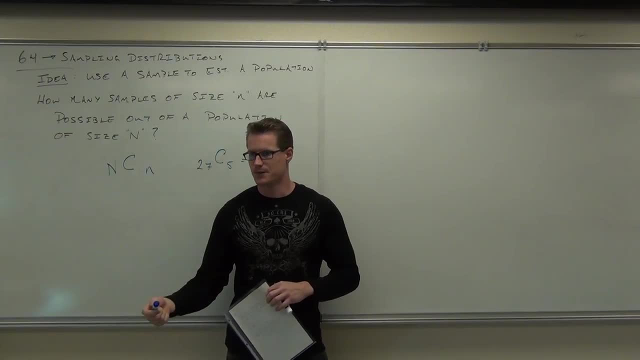 Trust me, you're going to want to learn this, Otherwise you can't make the next step, Otherwise you'd be forced to take all of them. You're going to have to take all of them. You're going to have to take all of them. 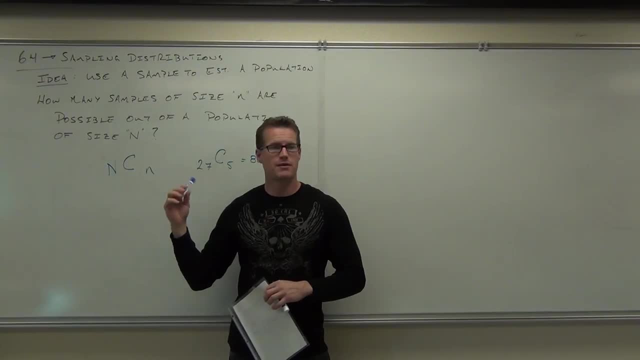 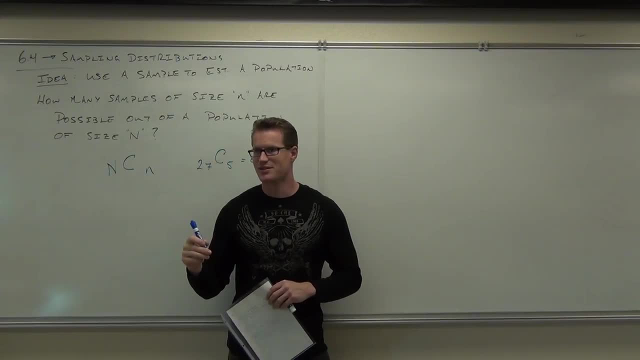 that I'm about to show you. Are you ready to learn it? Trust me, you're going to want to learn this. Otherwise, you can't make the next step. Otherwise you'd be forced to take all 80,730 of these samples. 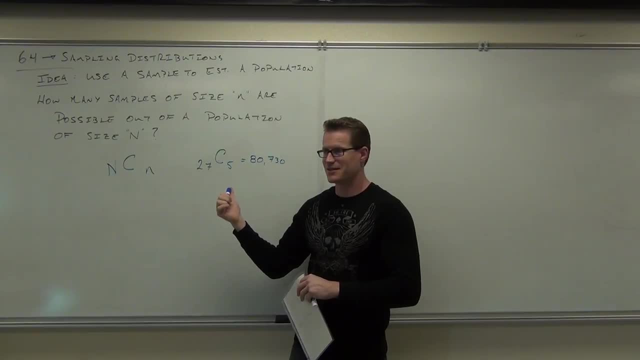 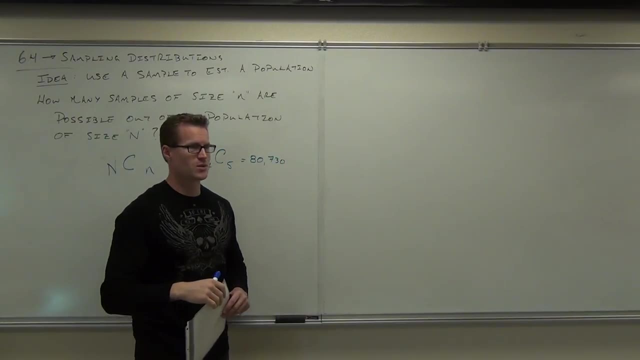 Don't you do that? That's a lot- 80,000,. I'd have to be counted. I counted up to five or eight or something like that. There'd be 80,722 of those remaining for me to go through before I exhausted all possibilities. 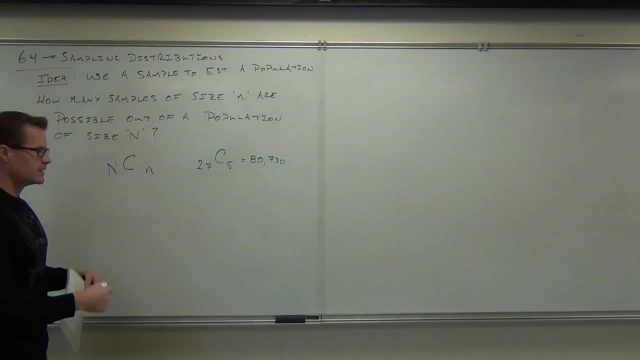 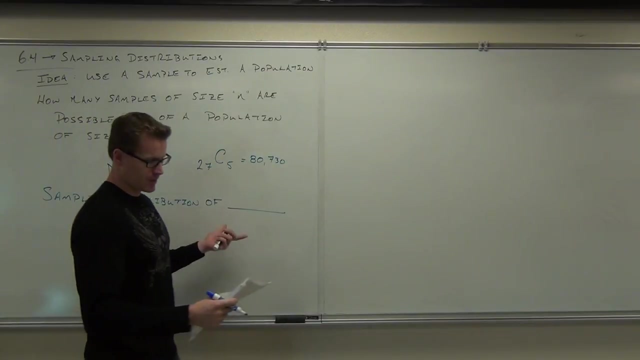 Okay, Now to go any further, I need to tell you what a sampling distribution actually means. A sampling distribution is a sampling distribution of blank. We can have one of three words here. We can have the mean, the proportion. well, one of many words actually. 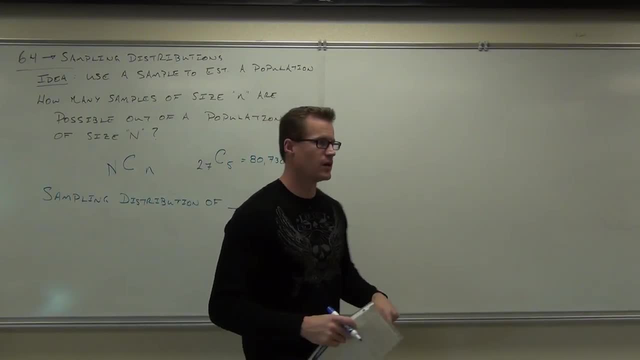 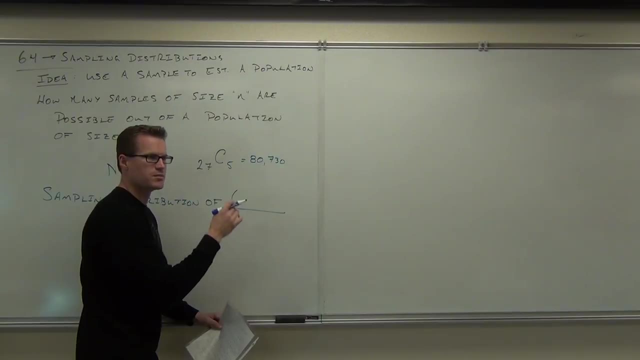 The mean, the proportion, the variance or the standard deviation, Sampling, distribution of. and then we're gonna have some sort of a- I'm gonna put it in parentheses, so you know it's some sort of a statistic like the mean or the proportion of data. 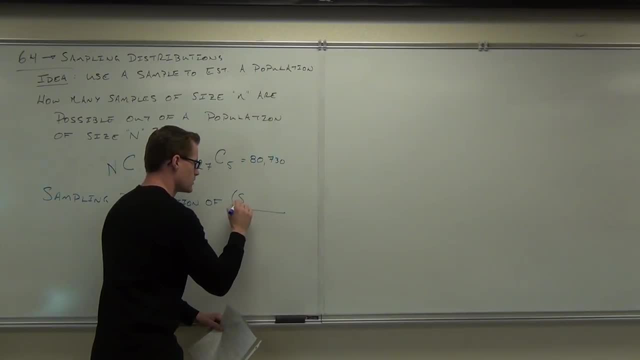 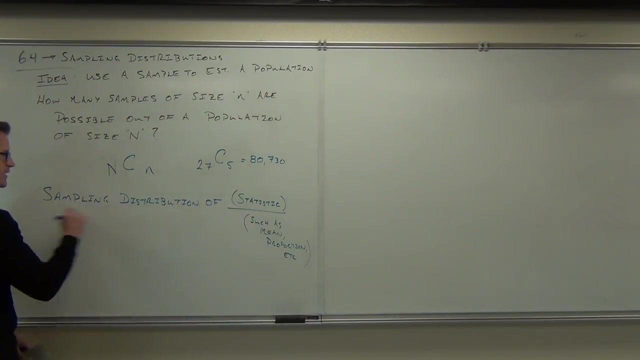 or the variance, So such as: Okay, So sampling distribution of mean proportion, et cetera. and of course et cetera is not a statistic for us, it just means and so on. okay, So, sampling distribution of some sort of statistic. 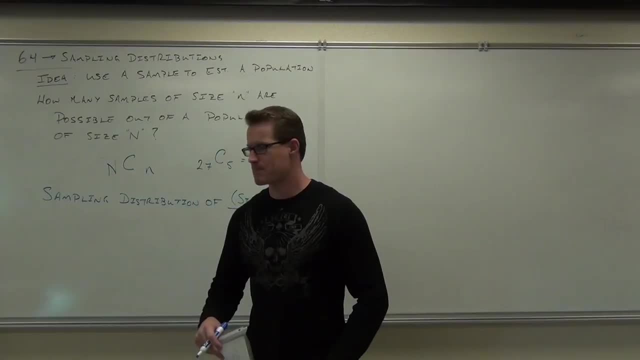 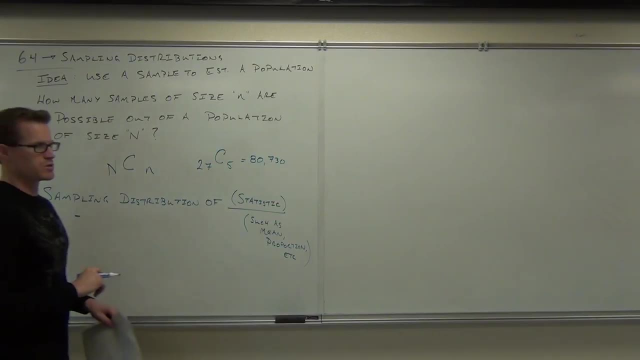 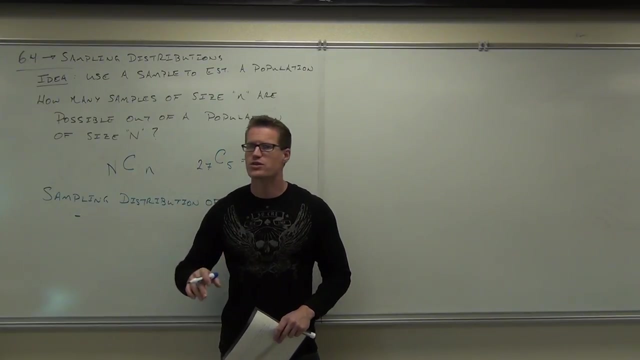 What a sampling distribution says is this: It's kind of an abstract idea because no one ever does this. Here's a sampling distribution. I want you to assume or pretend like you just took all the samples that are possible in a certain size out of a population. 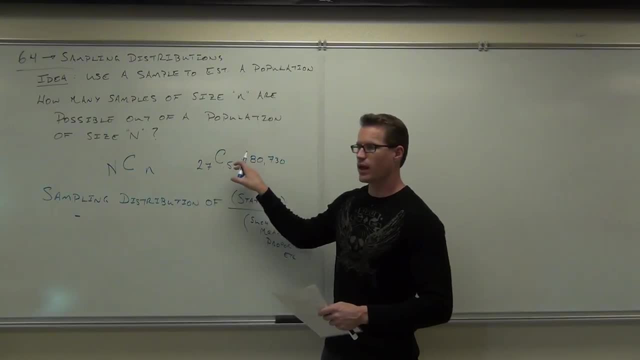 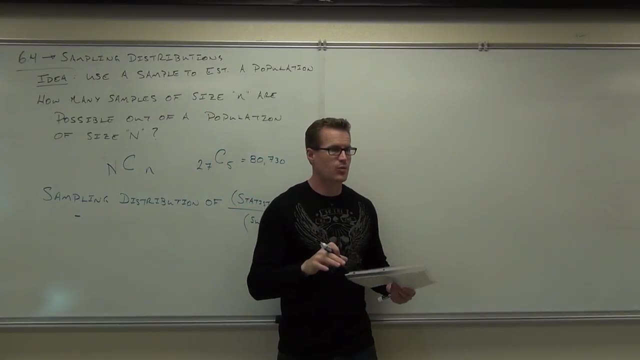 So stick with me on this. So, for our example, you would have taken all 80,730 samples you with me. You would have found out from that sample what the mean was or what the proportion was, What the variance was from those five, five people. 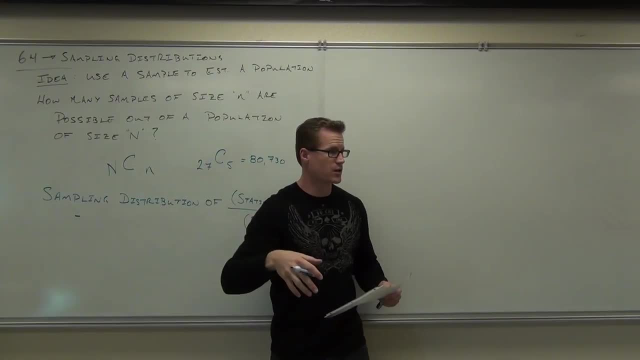 So, like I'd ask you well, like, what's your height? I'd say: what's your height, I'd average it. That's one statistic from that one sample. right, Are you following me along here? You do that 80,730 times. 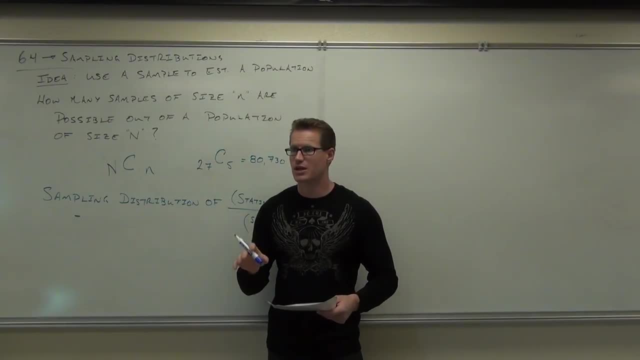 So you'd have 80,730 different samples. That means you're gonna get 80,730 different heights for those groups of five people. You with me on that. You organize all of those into a table and that is a sampling distribution. 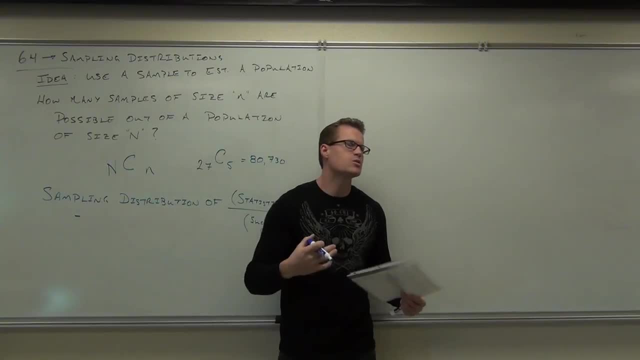 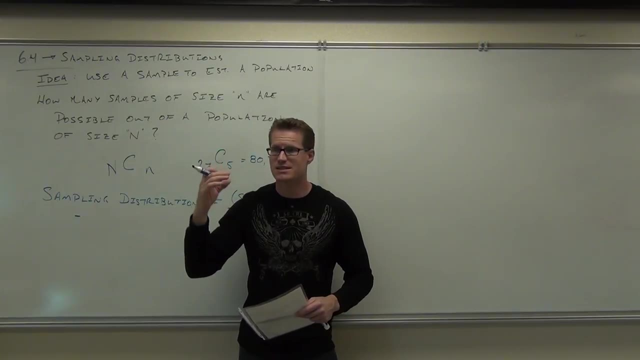 Okay. So what a sampling distribution does is this: takes all the different samples for a certain size out of a population, finds out the key statistic you're looking for for each one of them and it puts them in a table. Do you understand the idea of a sampling distribution? 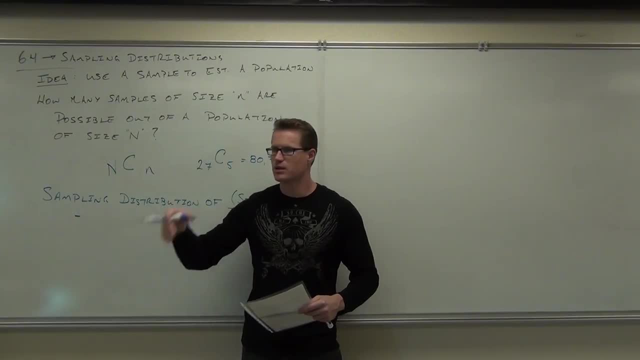 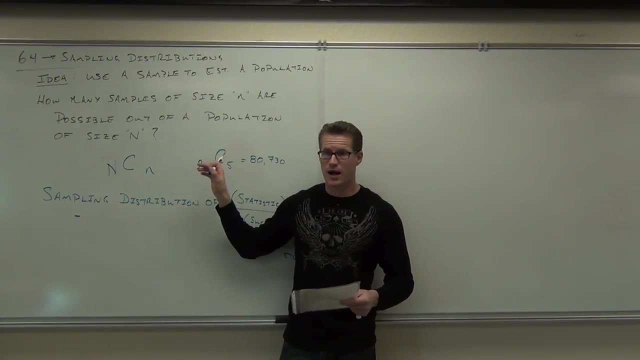 Sampling because you're taking samples. Distribution because you're organizing it. Sampling distribution. Now let me ask you one more question before I go any further. What if I change this to not just groups of five, I want groups of six now. 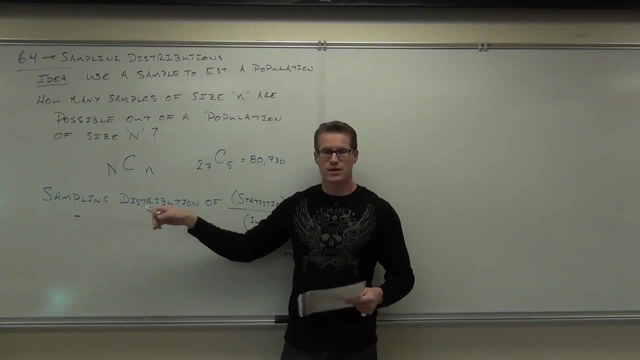 Does this number change? Then this would change. So this is for each particular size of sample that you want. If this number changes, does this number change? Yeah, So this is a very specific thing: Population size versus sample size, Every possible sample of that size. that you organize this as statistics for each one of. 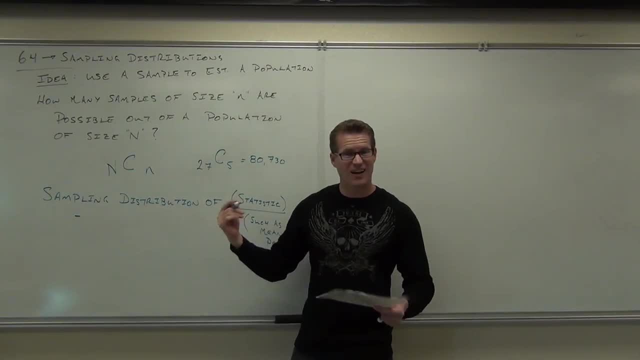 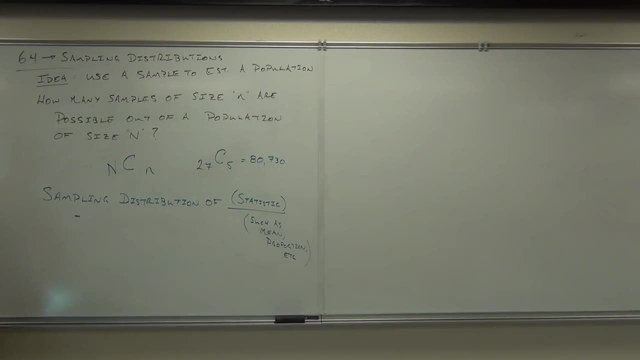 them. Are you ever gonna do that? No one ever does that. That's a lot. We're gonna look at this in a minute. So sampling distribution. I'll write this out in words for you. You're gonna assume that you take all the possible samples of size little n. 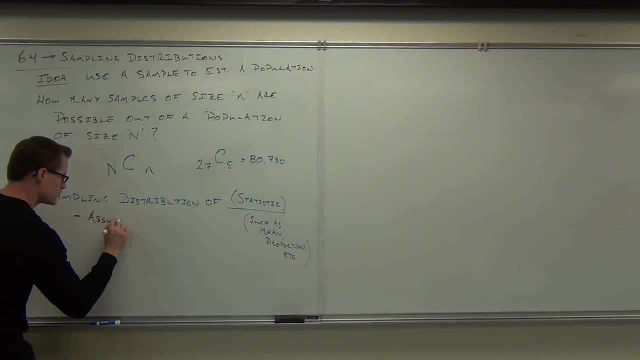 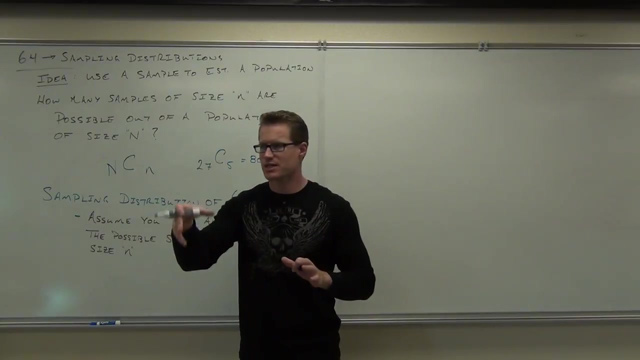 Bless you. Thank you, You too. Assume you take all the possible samples of size N. So again, for us that would be every possible sample of size 5 in this classroom, And you find the certain statistic for each one of them. 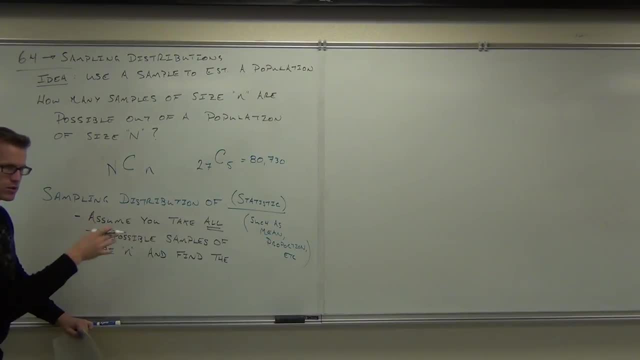 And I'll say: find the, let's say, required statistic, so the one you're looking for For each sample. in our case, that would be all 80,730 of them. We would have 80,730 different means. 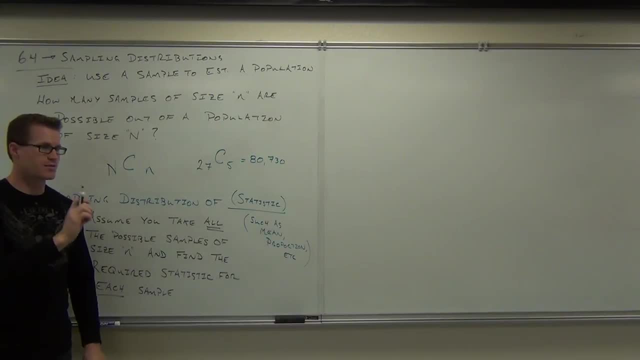 We'd have 80,730 different proportions, 80,730 different variances. Nod your head if you understand that. If you organize all of those in a table or a graph or et cetera, this is called a sampling distribution. 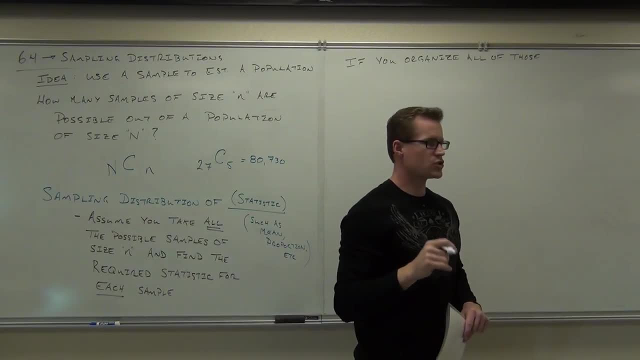 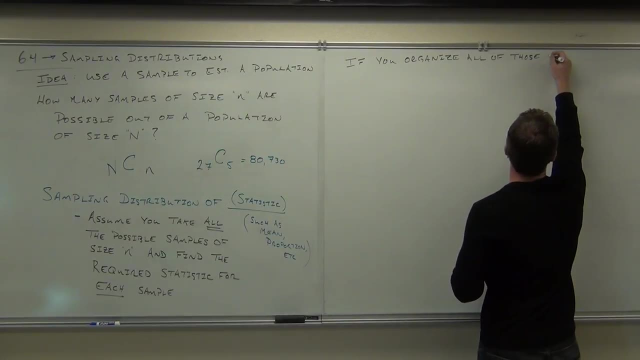 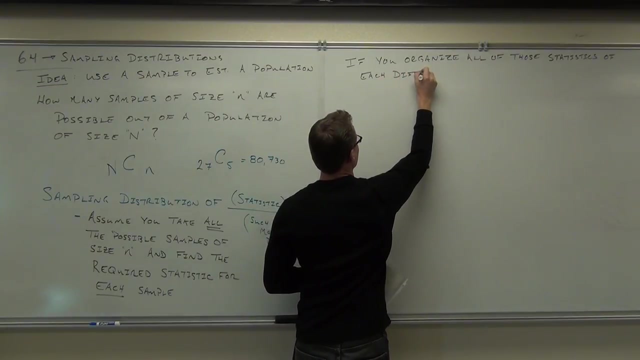 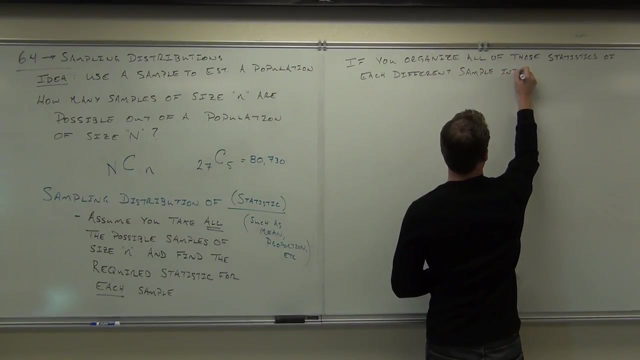 If you organize all of those different statistics for each different sample into a chart, graph, table, you are going to get a sampling distribution. Okay, Okay, We'll just say table, because you can make a chart out of a table and so on. 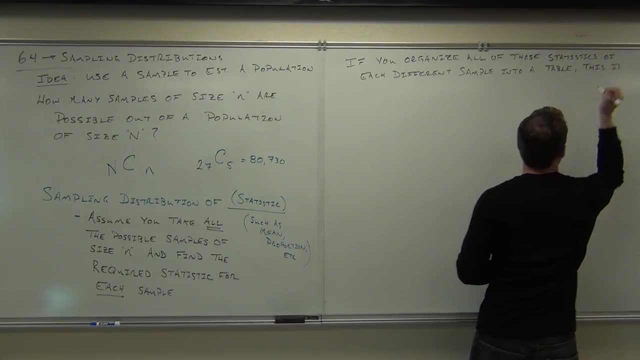 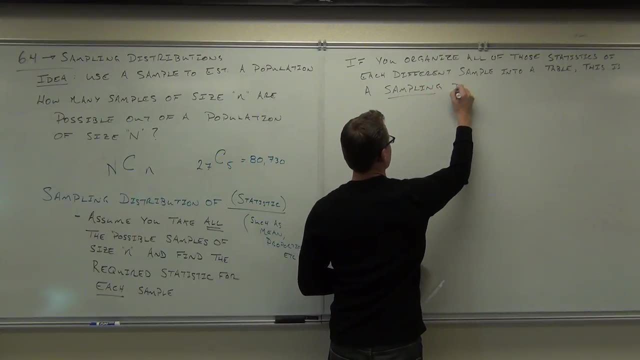 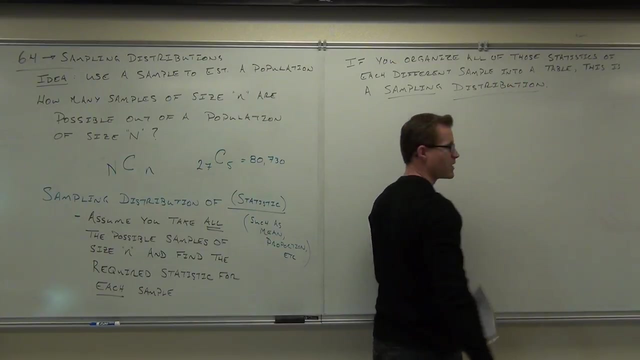 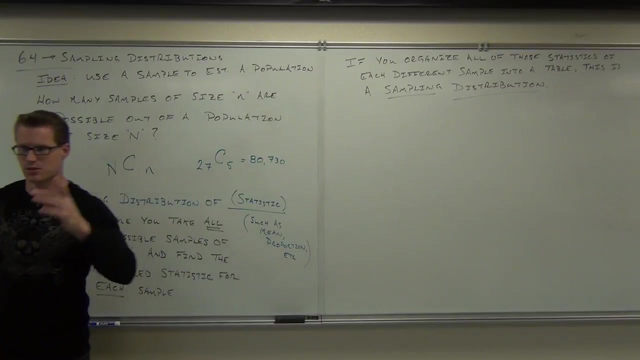 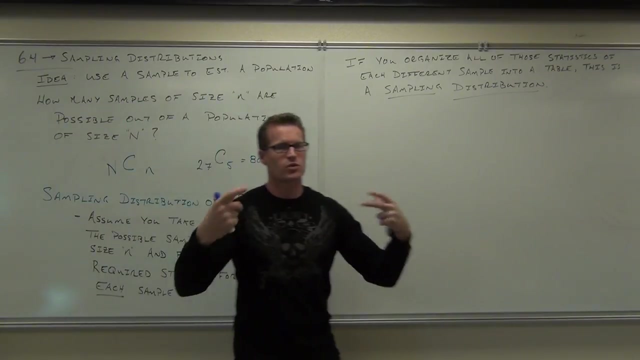 I'm going to kind of recap this one more time as soon as I get a new pen. Every time I miss Okay. so here's the idea: You have this population of a big N size N You're taking. you say: I want samples of size. 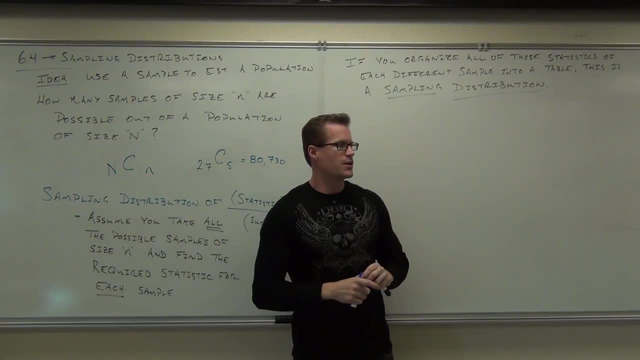 You pick that. so like 10,, 5,, whatever I pick 5.. The number of different samples you can get out of that population for a certain size- remember you're picking that size ahead of time, like I picked 5, can't change that is big N. choose little n. 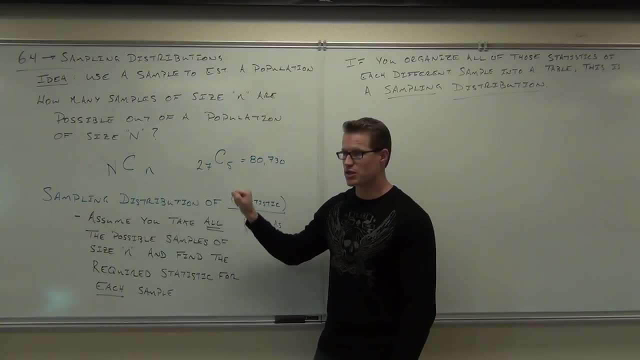 That's how many different samples are possible with any situation of a certain size. We take the statistic for every single one of those samples, all 80,730 in this case. This is a relatively small population right and small sample size. 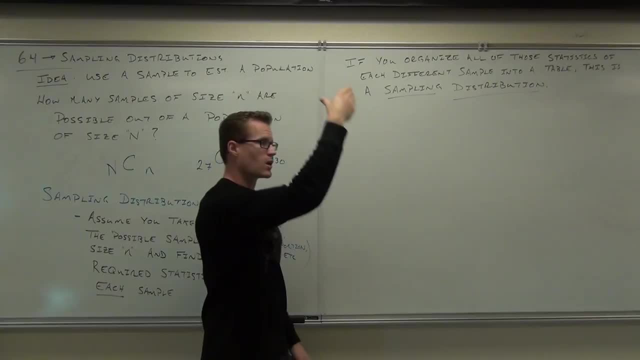 You increase these, you get massive numbers. You organize every one of those statistics with their appropriate, well, the required statistic you've been given, such as the mean or proportion, into a table, a net, And that's called a sampling distribution. 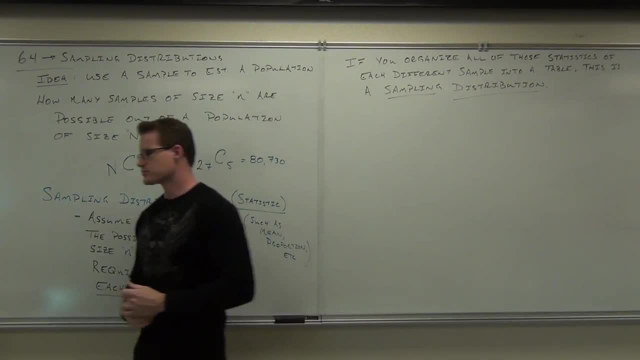 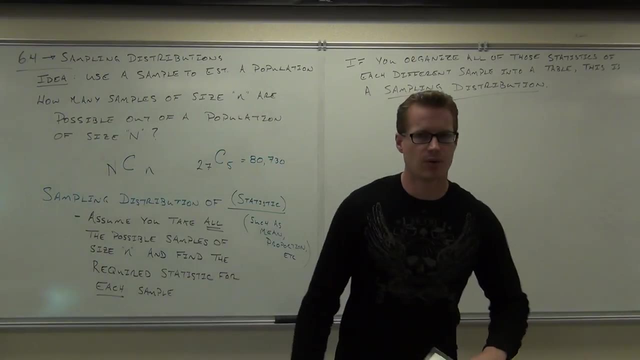 Raise your hand. if you understand the idea of a sampling distribution, Good, okay, Now let's learn about it. Let's learn really what happens here. I'm going to give you a very simple example to illustrate what sampling distributions are going to mean for us. 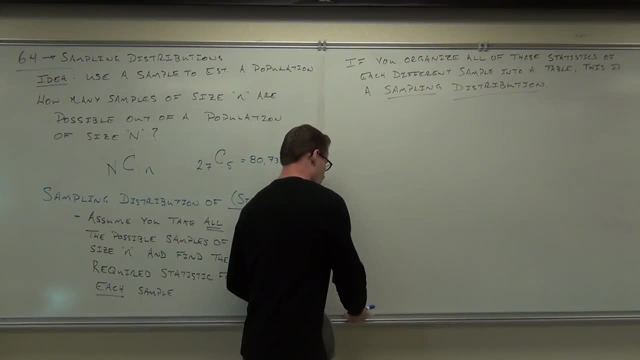 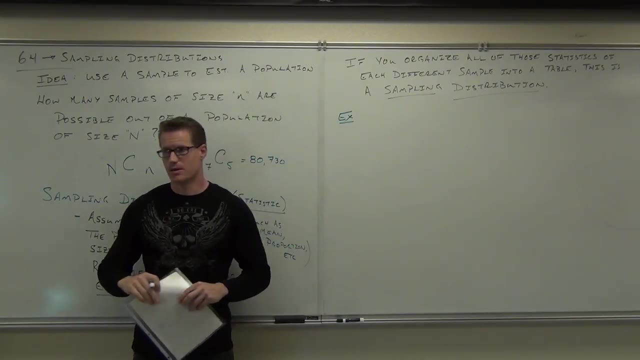 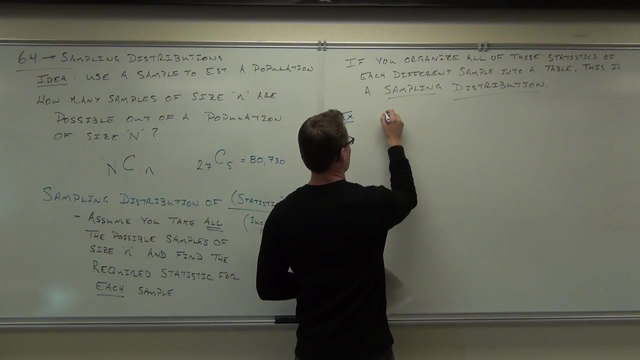 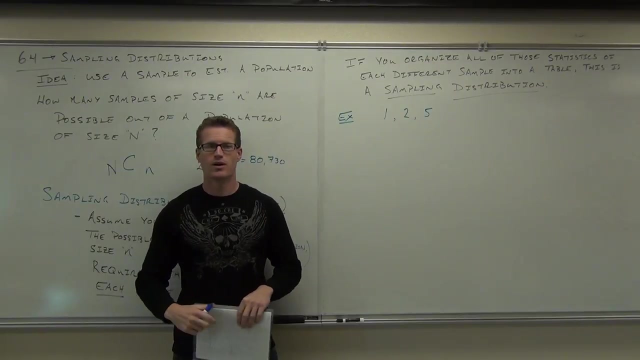 You ready to follow this example? You've got to kind of follow this. We're going to pretend that in the whole world there are only three numbers. The only three numbers you can possibly have are one, two or five. So if you started counting you'd go: I'm one years old, then I'm two years old, then I'm five years old and that's it. Okay, we'd all be five years old. That's it. So there's no other value besides one, two and five. Are you with me? No other numbers exist. It'd be like having a three-sided die, which is literally impossible, but let's pretend it is for this fact. 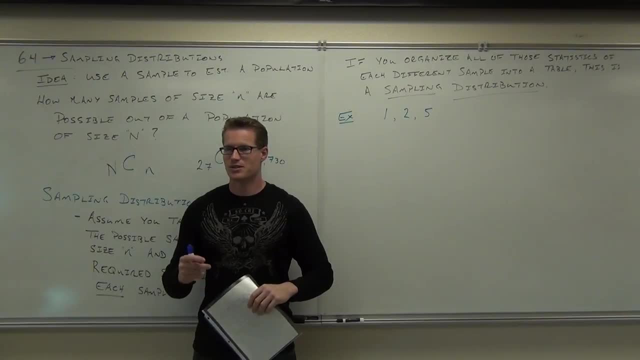 You know you can't get a three-sided die, But if you, let's pretend you had a three-sided die, The only numbers on there would be one, two and five, or are one, two and five and that's it. 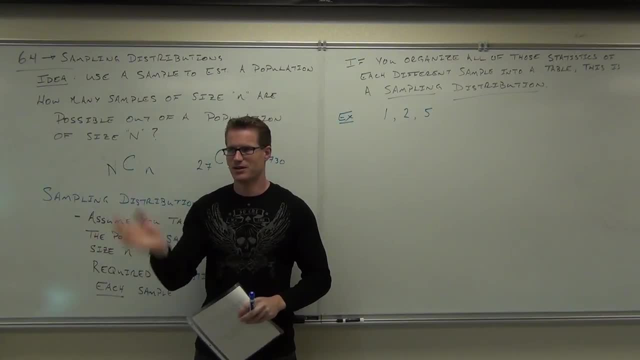 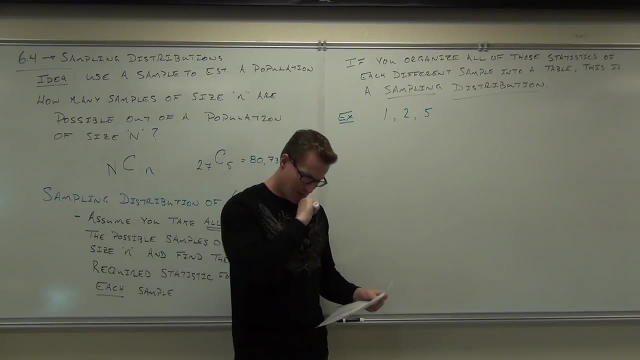 Okay, let's just pretend you label it one, two, five and you get to roll it, You understand. So the only thing you can get out of it is one, two and five. That's another way to think of this. 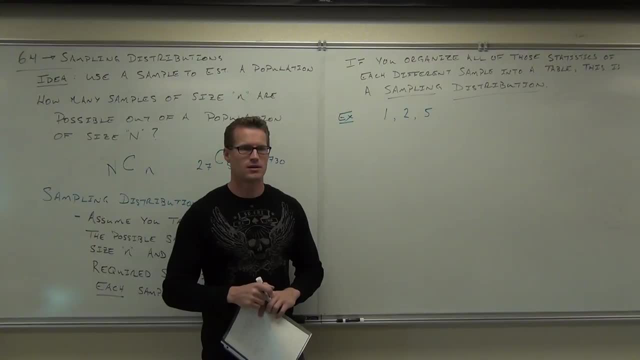 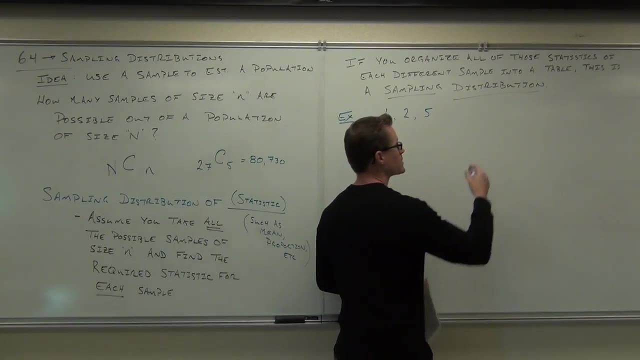 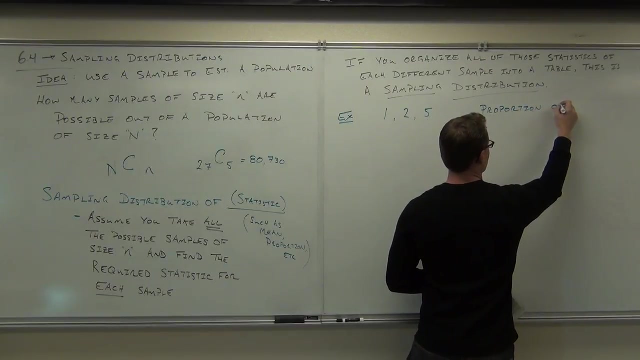 How many odd numbers do you have? How many even numbers do you have? Okay, thankfully we got that. We got that right. So we got two odd numbers, We got one even number. Can you tell me what's the proportion of odd numbers? 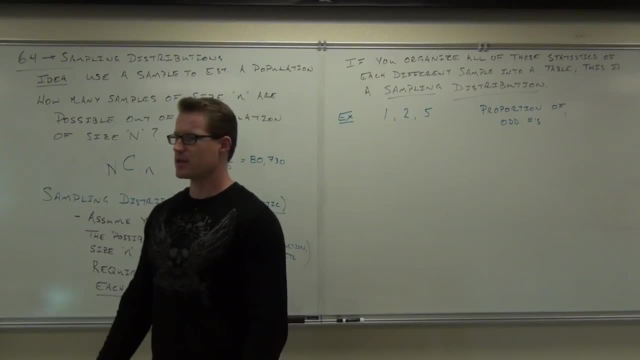 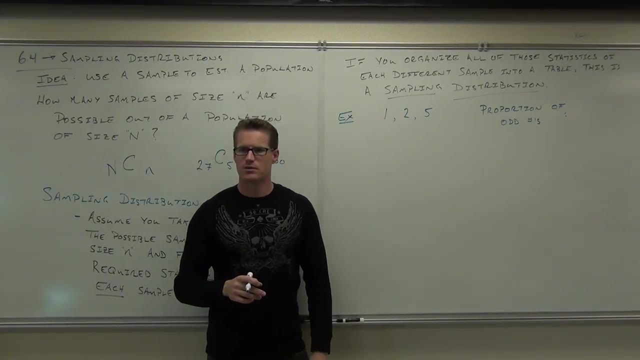 What's the proportion of odd numbers? That means like, not a percentage but a decimal version of percentage. How many odd numbers do we have out of how many numbers total? So our proportion is two-thirds. You'd say two-thirds of these numbers. 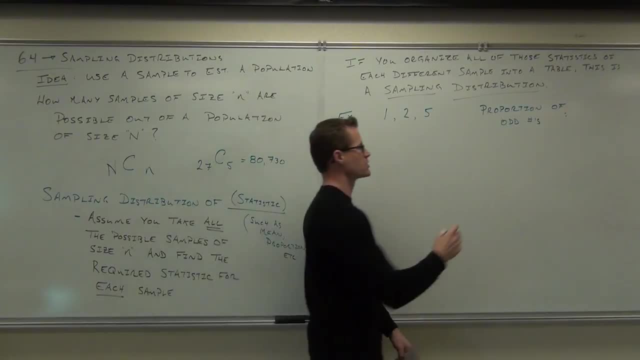 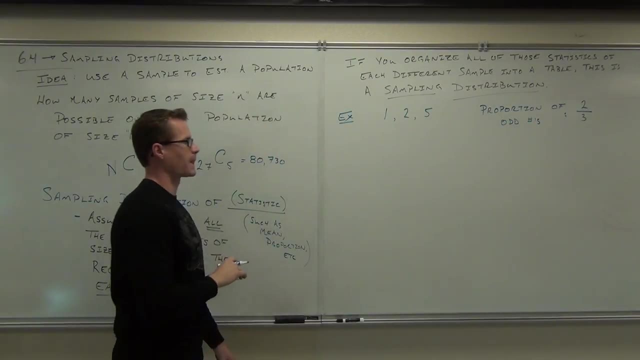 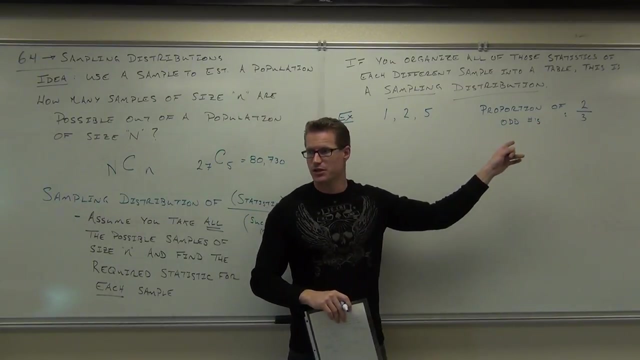 Two-thirds of these numbers are odd. Are you with me on that? Our proportion is two-thirds, Or the proportion of odd numbers is two-thirds. What we're going to do now. this is not a sampling distribution, by the way. This is looking at the entire population. 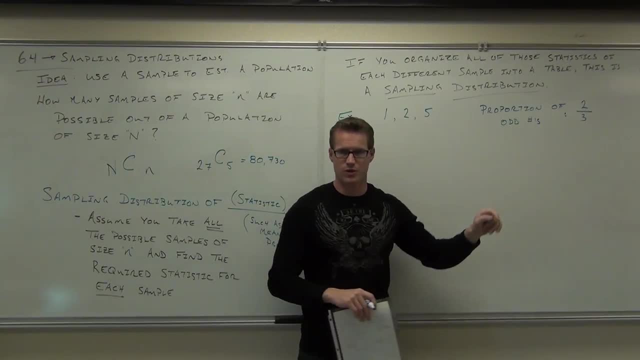 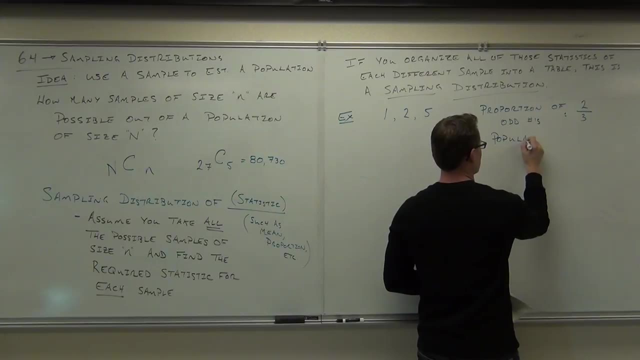 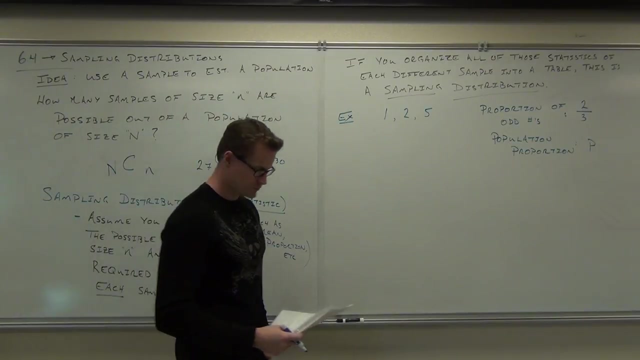 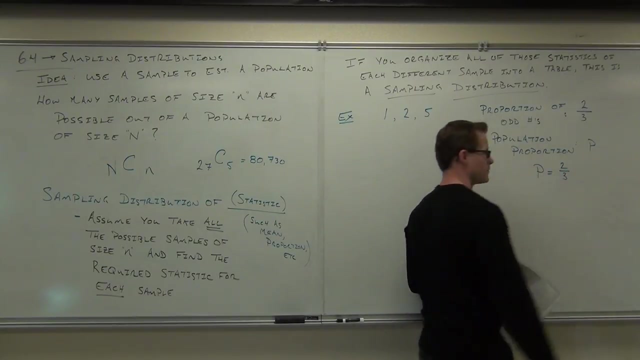 Understand that this is the population proportion. Are you with me? That's the population proportion. Population proportion is a lowercase letter, p. So in our case, p equals two-thirds The population proportion of odd numbers. in our case, because this is our population. 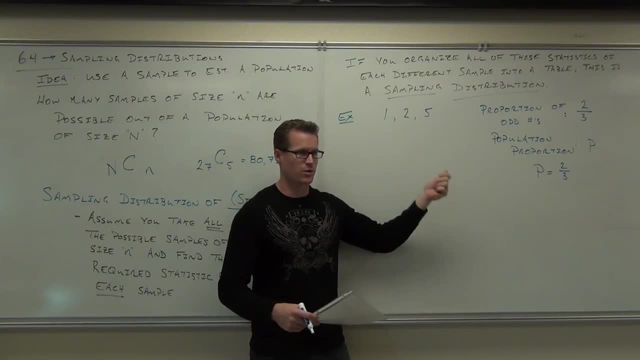 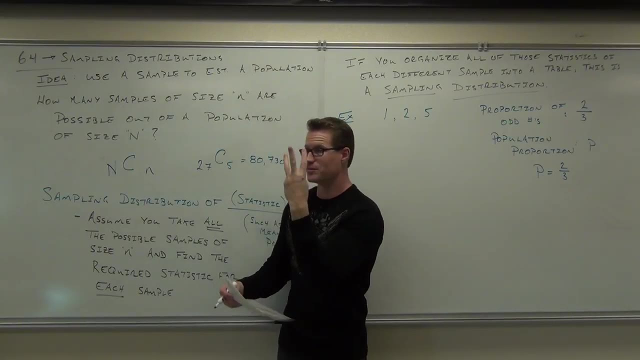 You're following that right. That's it. That's all that's possible is one, two or five. So the population proportion of odd numbers is two-thirds. This is a very, very simplistic example. I only have three items. 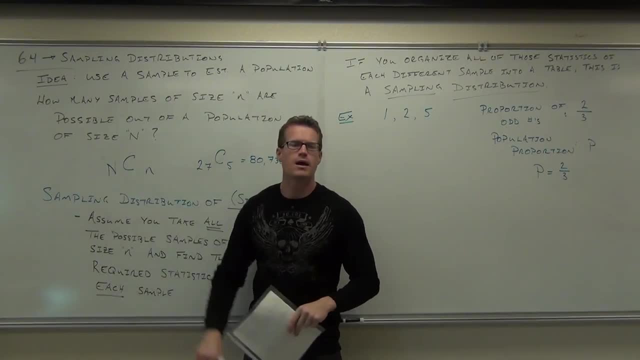 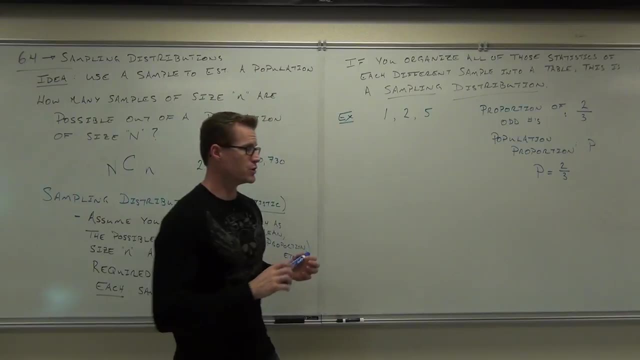 This would be three. Okay, that's it. That's all you can choose from is three. Now, what I'm going to do is I'm going to create for you, with you, a sampling distribution. What we're going to do is we're going to take all the possible samples of size two. 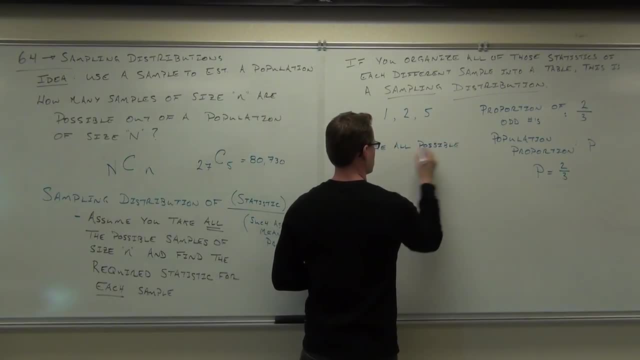 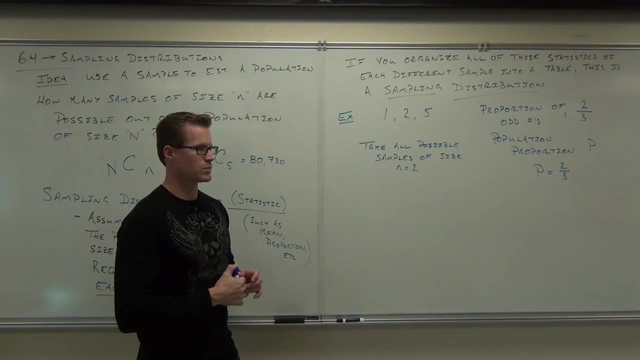 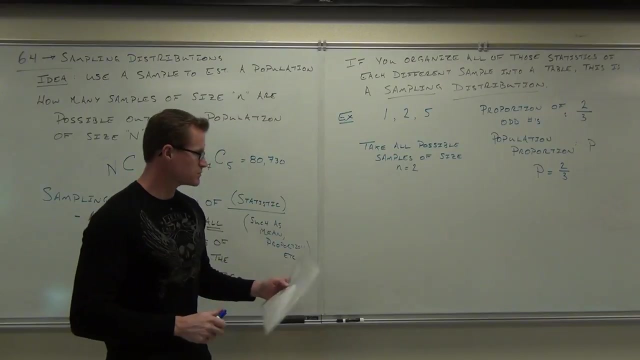 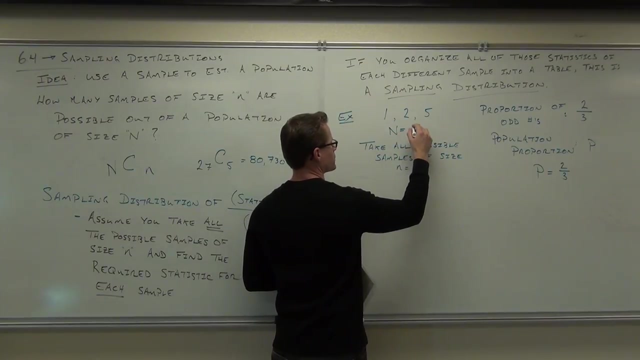 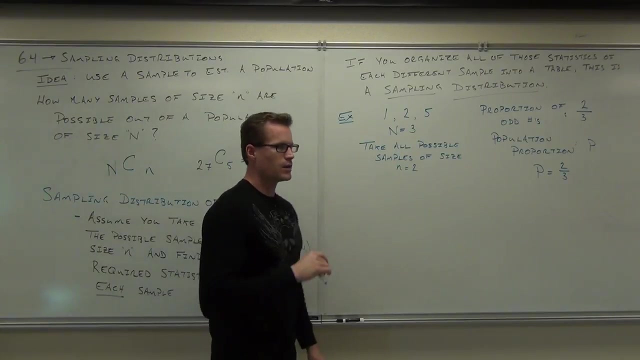 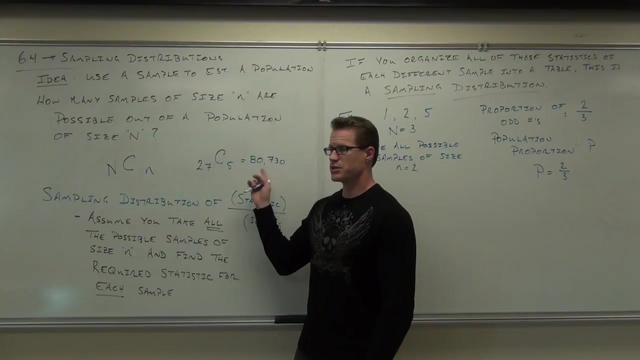 All the possible samples of size two. All the possible samples of size two. So big N equals 3,, little n equals 2.. Now something interesting happens here. I'm going to break the rule just a little bit. These are all the different samples that you can get. 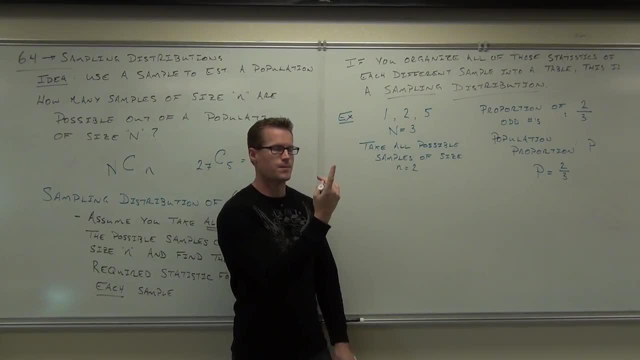 However, I'm going to label the different orders of these as unique samples, just so like the probabilities can come out right, because you have the different order and it raises the probability because you're dealing with two samples, two numbers at a time. 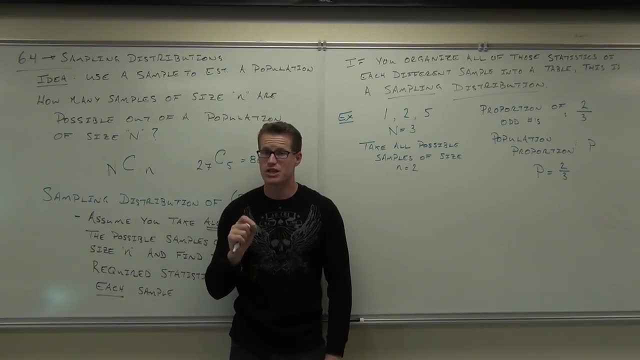 So you'd have to multiply and there's some sort of a probability. So I'm going to cheat just a little bit. We're not going to get the do 3C2 on your calculator real quick. Three, You get three. 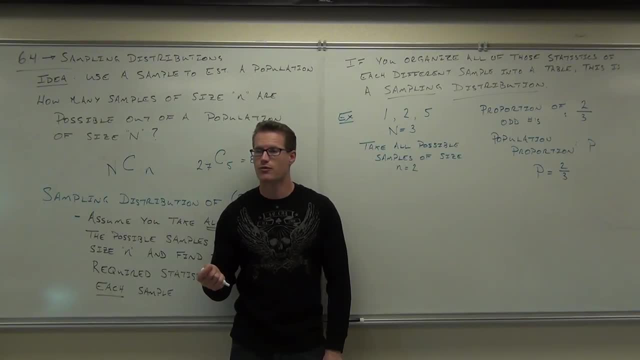 We're going to have three actually unique samples. However, what I'm going to list out is every possible order. I'm going to list out the order of those samples because, out of those three samples, the probability is actually higher for certain ones of them. 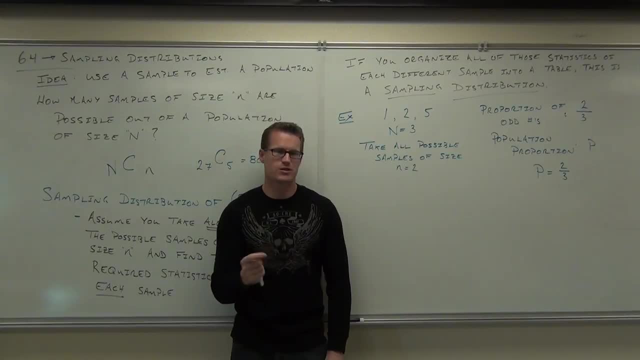 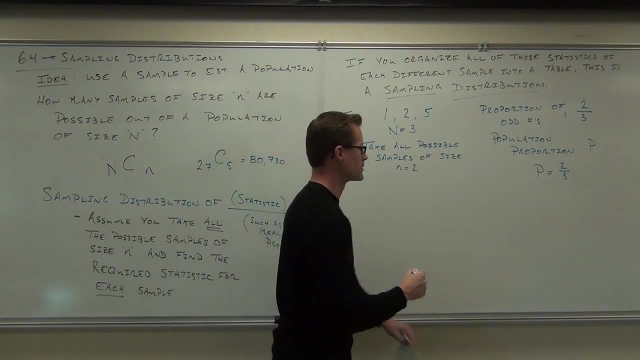 Does that make sense? So we're going to fudge a little bit. There's two ways you can do it. You can change the probability or label out every possible choice, So I'll show that to you when I create this. 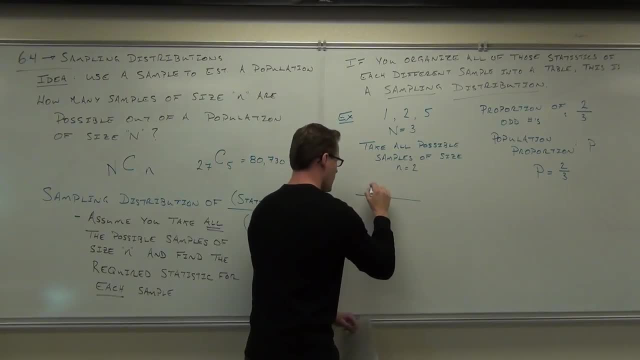 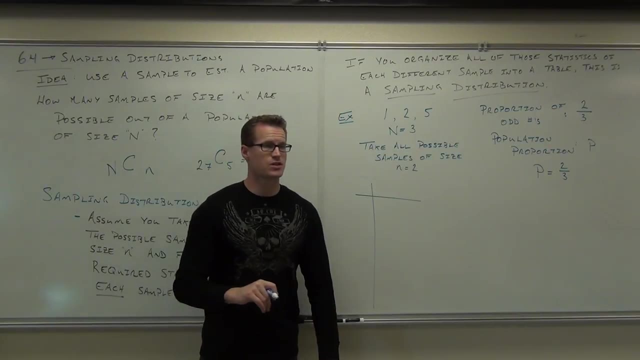 We're going to make a table here. What we're going to do is list out every possible sample on the left and I'll show you what we want to do on the right. Give me the first possible sample. This is with repetition, So with repetition. 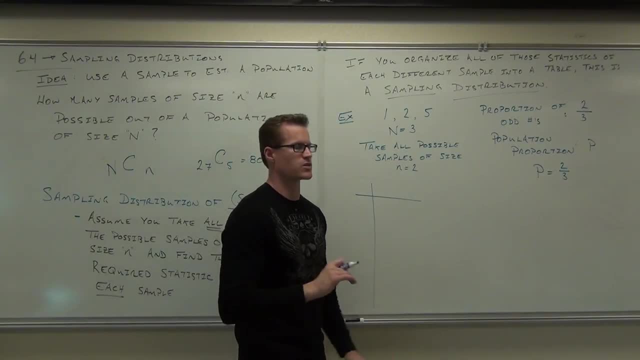 Remember, it's like you're rolling a three-sided die, which literally is impossible, but let's try that. So what could you get for your first sample? It's like you're rolling a die: The numbers you could pick out of or pick. 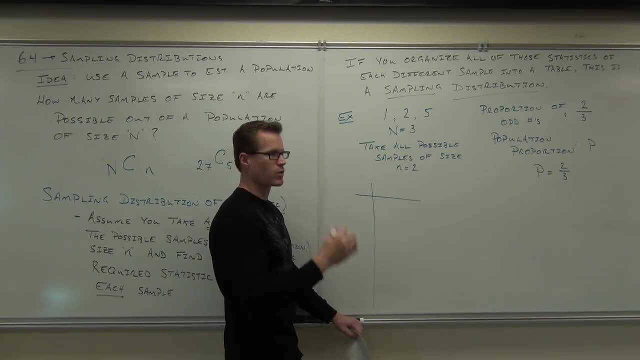 out of a hat with replacement One one. You get one one, Couldn't you? Okay, Then you could get one. two, Do you follow? No, Then you could get one. what One one. I'm going to run out of room. 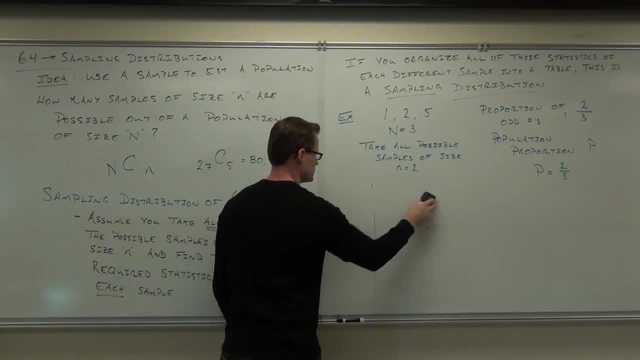 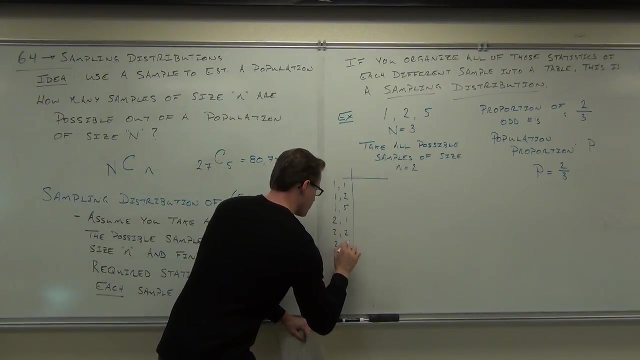 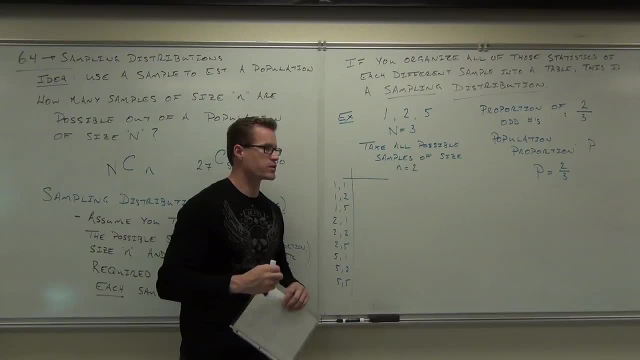 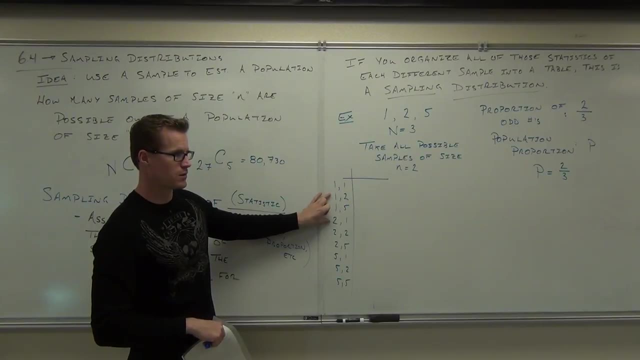 Yes, No, That's it. Now I do need you to know something that, according to the samples, this one and this one are the same. You follow: This one and this one are the same. This one and this one are the same. 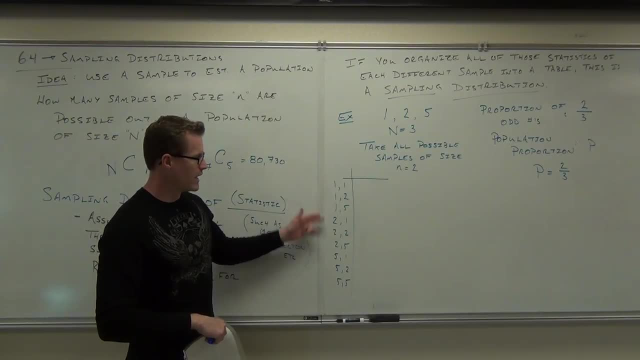 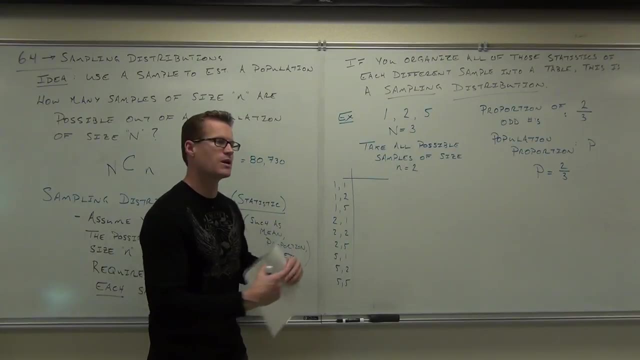 So you have less actual samples than what's listed. However, this is every possible rolling of the die. This is everything that possibly could happen. So if you were to make one sample out of these ones, you'd have to alter the probability of getting those. 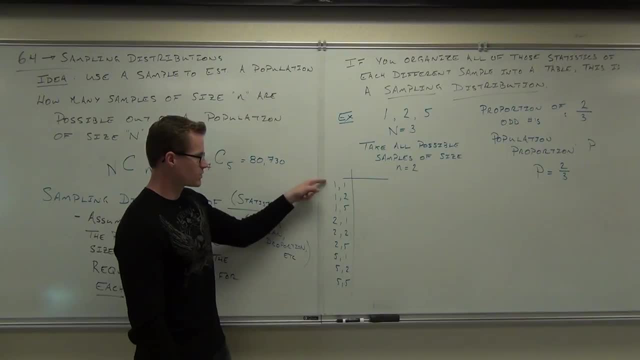 which we're going to do. So I don't want to alter the probability, because this would. this is not. this one sample can only happen one time. This sample can happen two different times, as can this one and this one, but not that one. 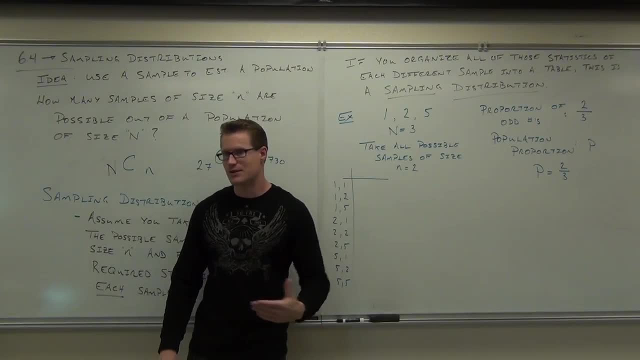 So I don't really want to confuse that idea. So I'm going to keep this listed as different samples. Do you kind of get the picture? So, even though I know these are the same for the probability-wise, I'm going to leave them. 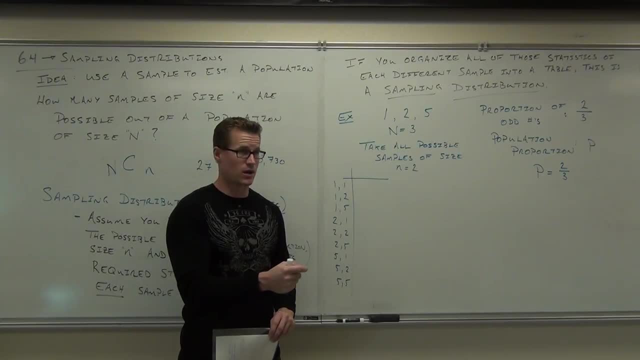 as independent and deal with the probability that way. I'd like to know if you're still okay on that. That's a little confusing topic. I'd love to. I don't really get that. I thought you said that the different order didn't matter. 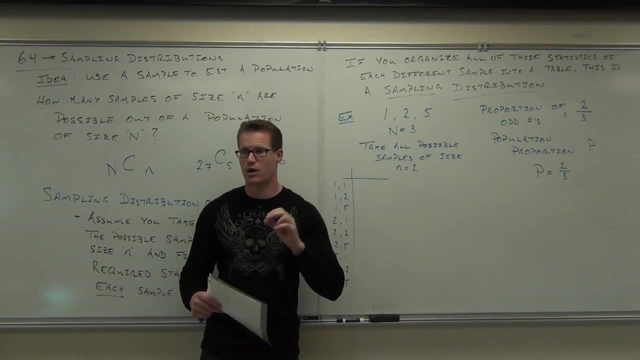 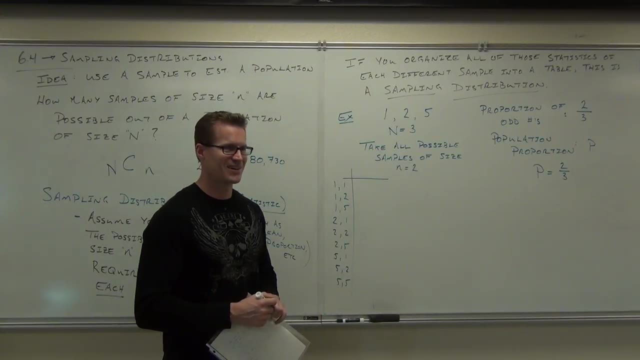 for samples It doesn't, but it does matter for probability and we are combining the idea of different samples with probability right now. Ready, That's a lot of a lot of talk. So this is our, our different n's. 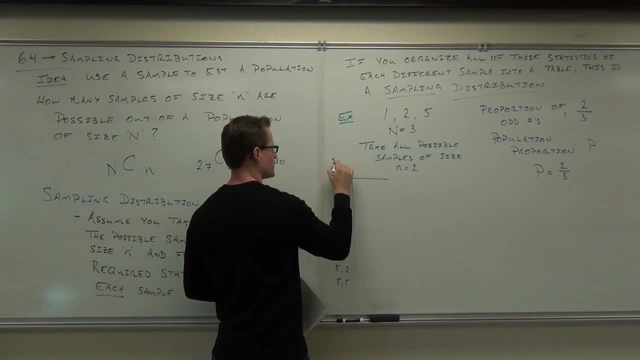 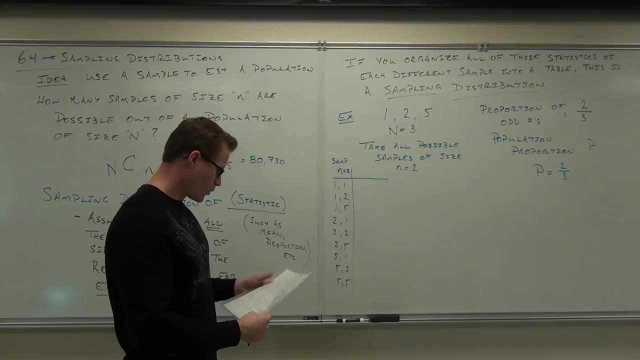 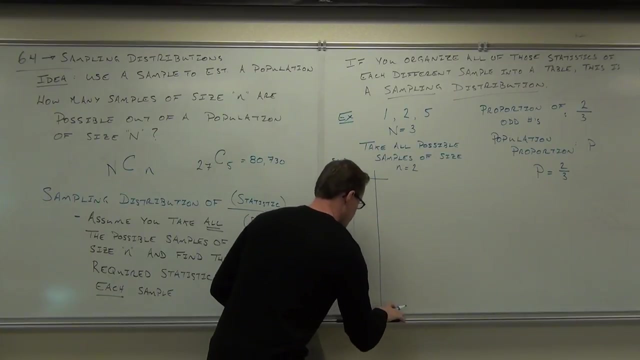 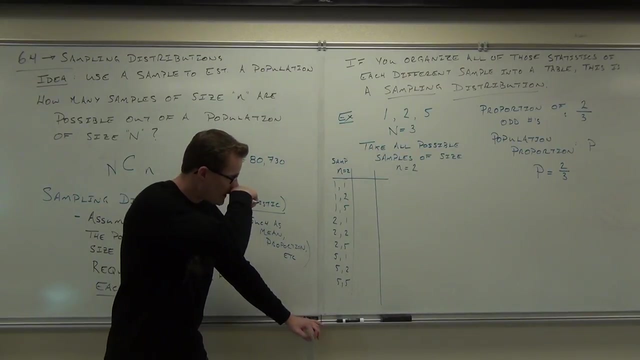 That's our different n's, our samples. Samples of n equals 2.. What I want to do now is I want to figure out the probability that each of these things is going to happen. How many choices do I have? So what's the probability that this one's going to happen? 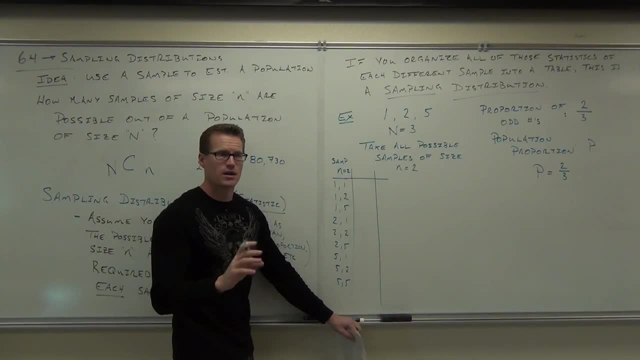 Yeah, we're assuming that the the die, our three-sided die, is not weighted. funny right, It's a normal three-sided die, So this probability would be one-ninth. You okay with that? What's this probability? What's all the probabilities? 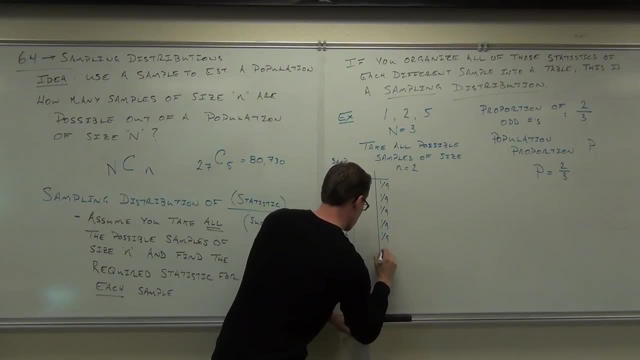 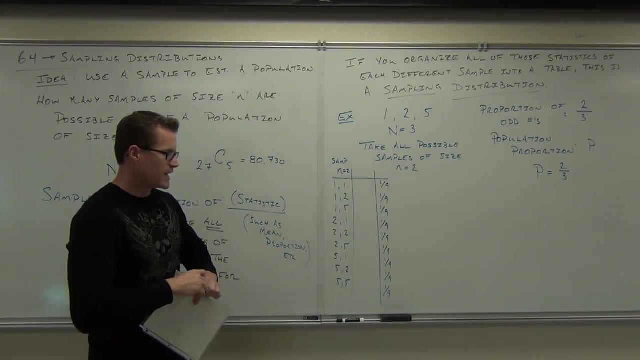 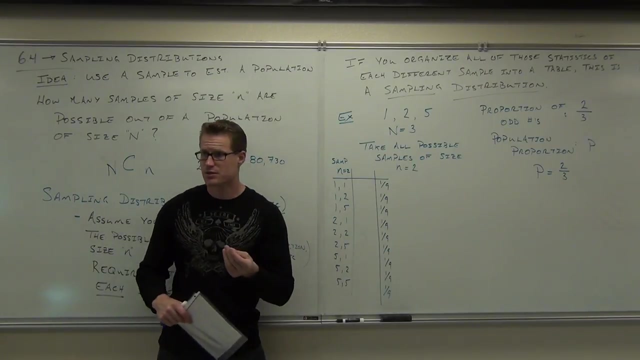 Here's kind of what I was talking about. If you were to combine these samples, like this one and this one, you'd alter the probability to two-ninths. That's the only thing that we'd do, but I needed to show you this. 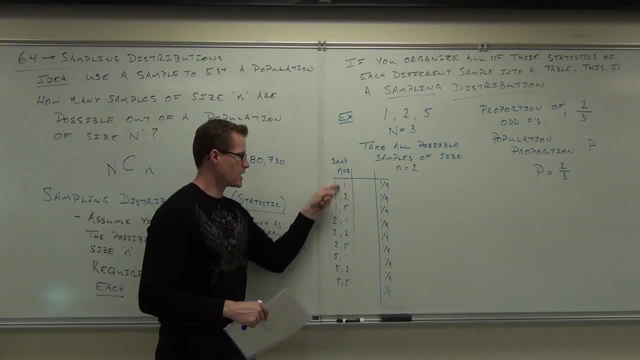 in order to do that. Does that make sense? So the probability for this one to stay one-ninth- there's not another one of those. Probability here would be one-ninth. it would stay. Probability this one. if you combine it would be two-ninths. 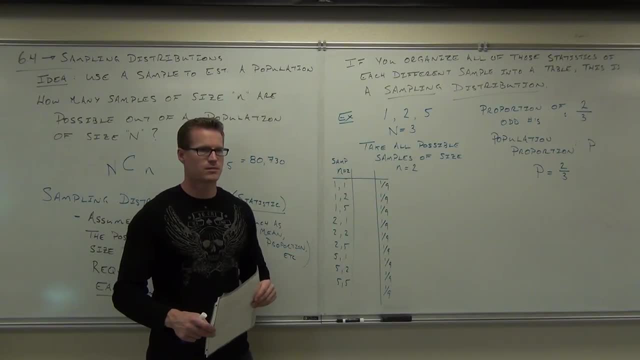 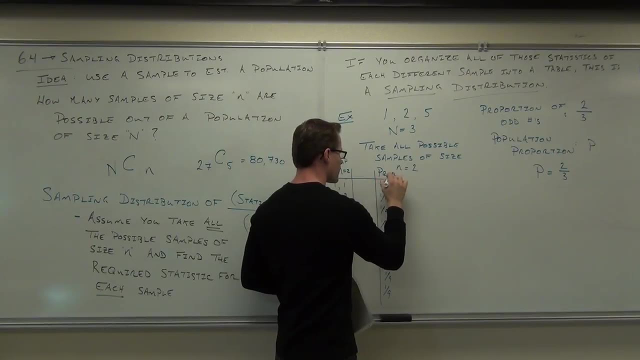 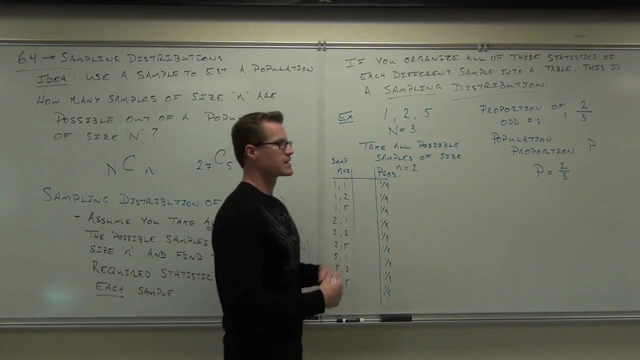 That would be two-ninths. So far, so good. Okay, Now, if this is the probability, the other thing that we're going to talk about is the sample proportion. The population proportion was this lowercase letter P In our case? 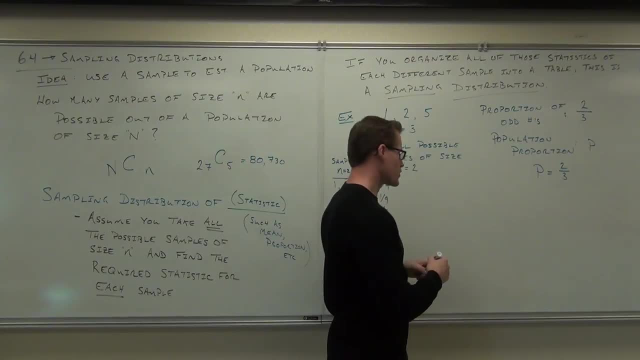 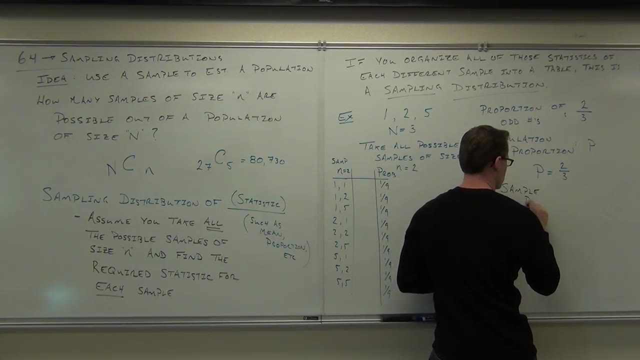 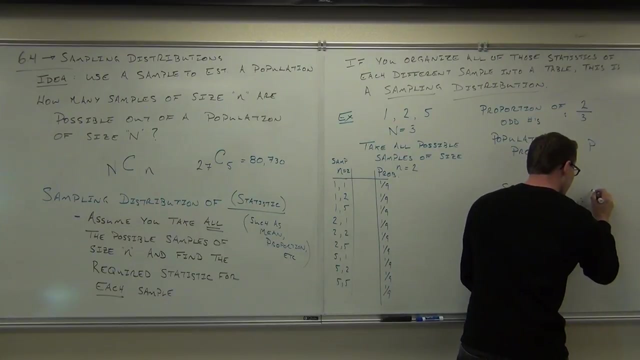 for our population. we had two-thirds of those numbers being odd. There's also another thing we need to talk about, and that's the sample proportion. The population proportion is P. The sample proportion is also P, with a little hat, P hat, I'm not kidding. 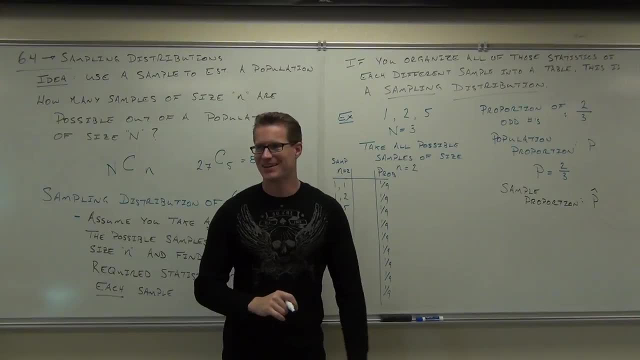 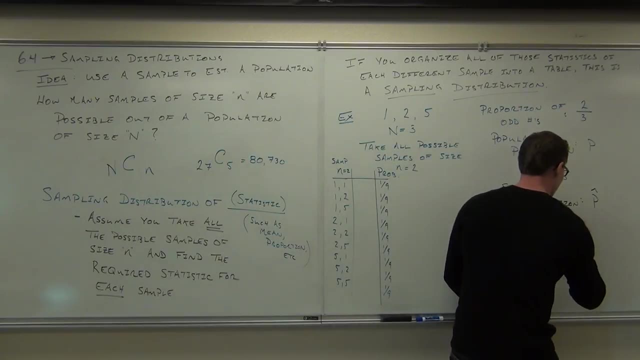 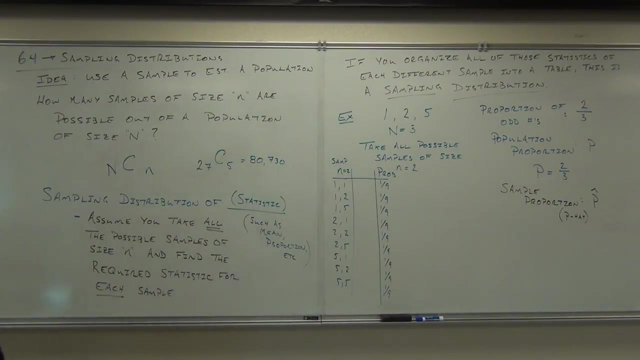 Seriously, I'm not even making that up. It's pronounced P hat. So aren't you glad you don't have a P hat. P hat stands for sample proportion. Usually I make stuff like that up just to mess with you guys. 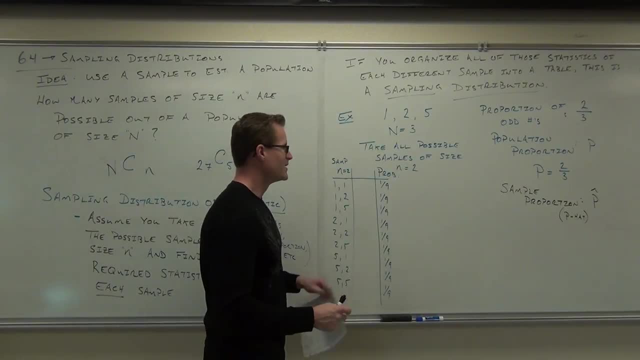 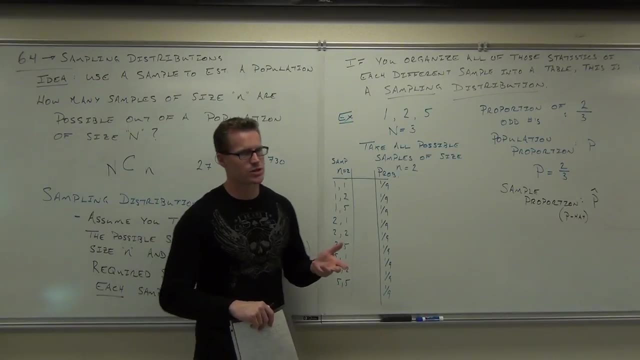 but I'm not making that up. That's honest. That's good enough as it is okay. So, firstly, are you okay that these are all of our samples? Yes, no, With replacement. You might also notice that that I'm doing something with replacement, but in real life. 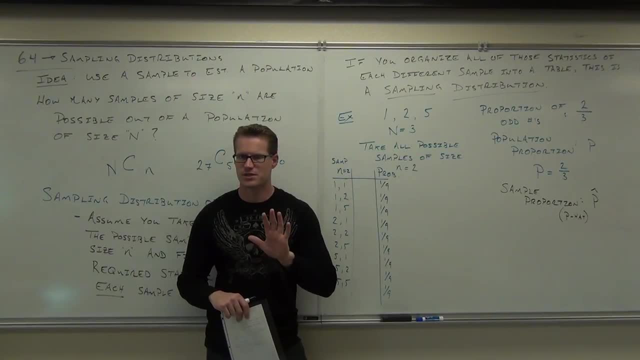 would you ever do that with replacement? If I wanted samples of size five, would I go: oh, okay, let's pick out five people. Kayla, what do you think? Okay, good, Kayla, what do you think? 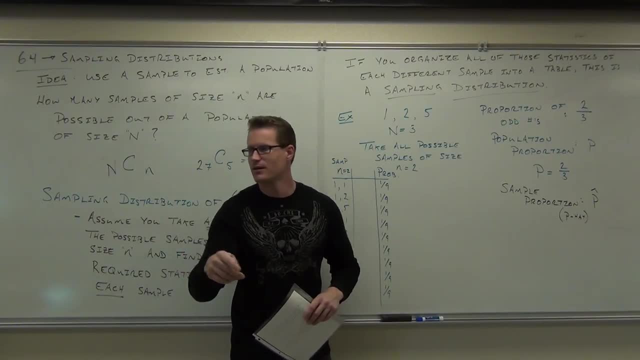 Let's pick someone else. Okay, Kayla, what do you think? Let's go to some Kayla, what do you think? And we need one more? how about Kayla? Kayla, what do you think? Would you ever do that? 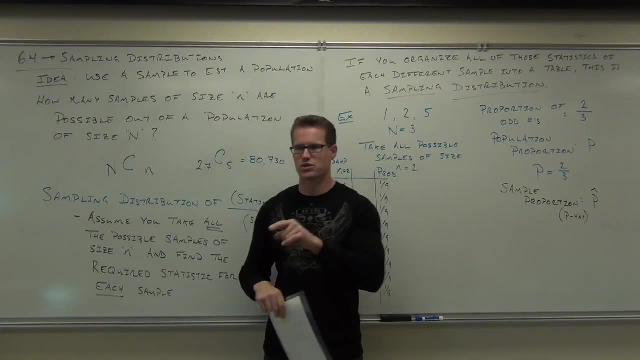 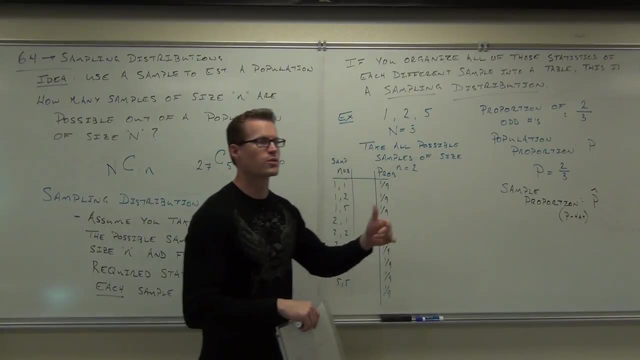 No, you wouldn't. So you're going to read something in that section, so I want you to read that about why we can consider the with replacement in this situation. okay, It explains that in the book pretty well. Read through that- why we are doing this with replacement. 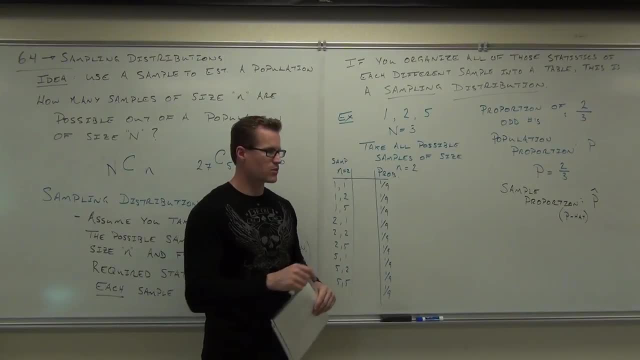 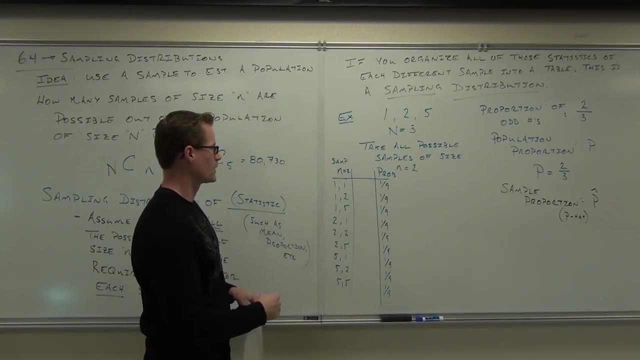 It's a good little little read. I don't remember what page it's on, but read through there. That's going to explain in there why the with replacement versus without replacement. we need the with replacement to do this, So are you okay that all these probabilities are one-ninth? 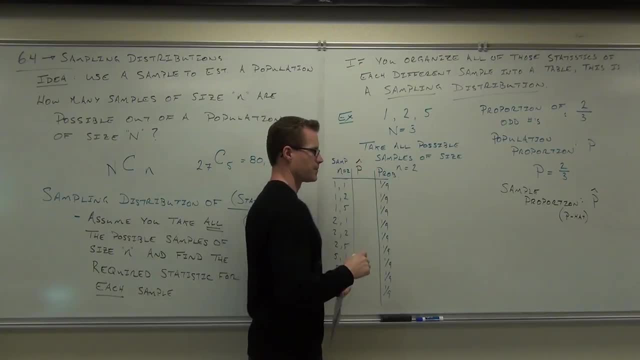 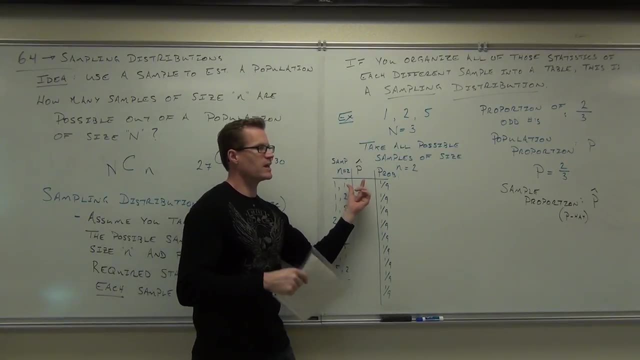 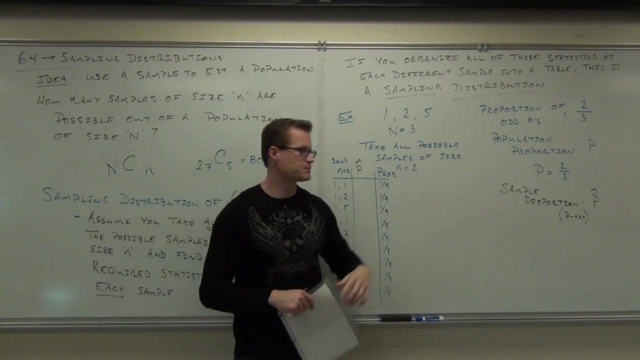 We also want to find out the p-hat. We're going to learn something right now that's going to going to tell us a relationship between p-hat and p, our sample proportions and our population proportion. What is the what's the p stand for? again, 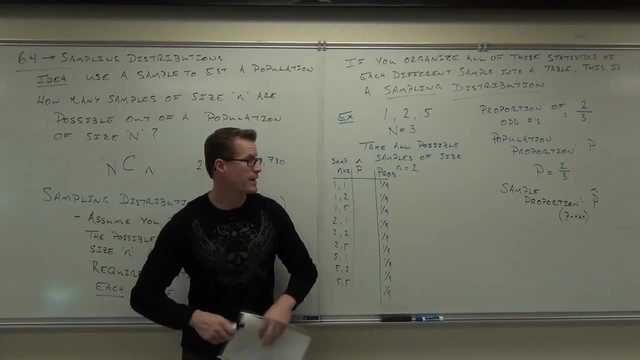 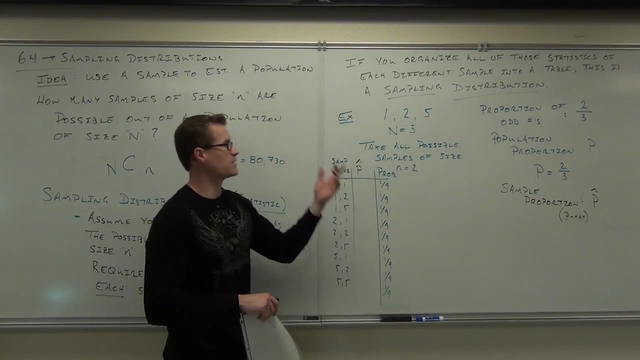 The p in this case. what are we looking for? Okay, yeah, this would be population proportion, This would be sample proportion of what. What specifically? look at our problem. What specifically are we? are we looking at The proportion of what? 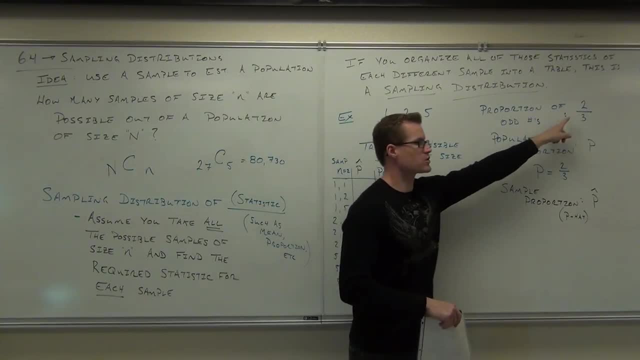 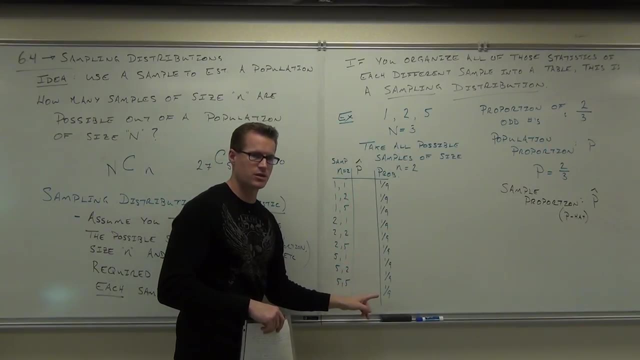 Odd numbers, Odd numbers, odd numbers. So two-thirds of these were odd numbers. We're going to go down the list right here and figure out the proportion for each of these, for each of these as far as odd numbers goes. So question: how many numbers do I have here? 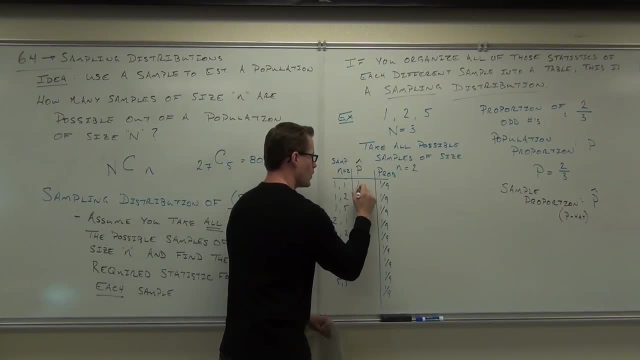 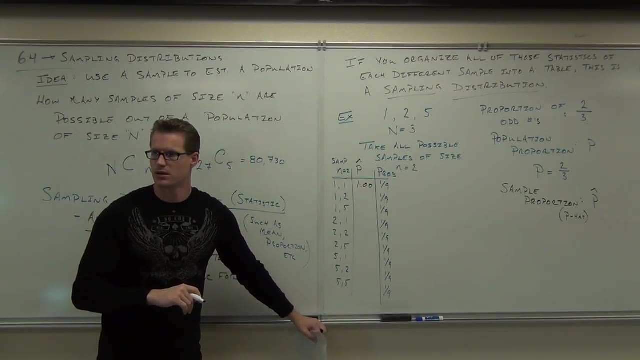 And how many of them are odd. So 100% of them 1.00, are odd numbers 1.0.. Do you follow that? What's the proportion? All of them? What's the proportion for odd numbers in this case? 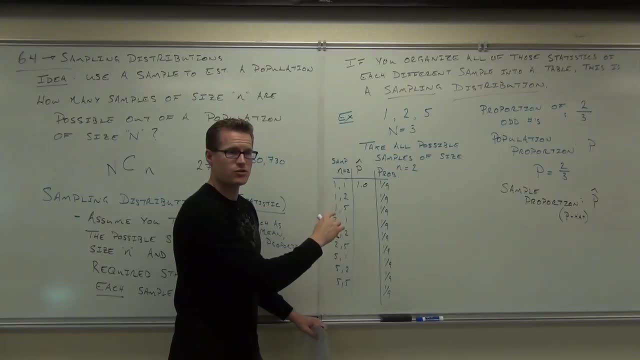 One, How much? .5.. .5,, sure, half of them. What's the proportion for this case? How about this case? How about the two? two, How many? how many odd numbers do I have there? 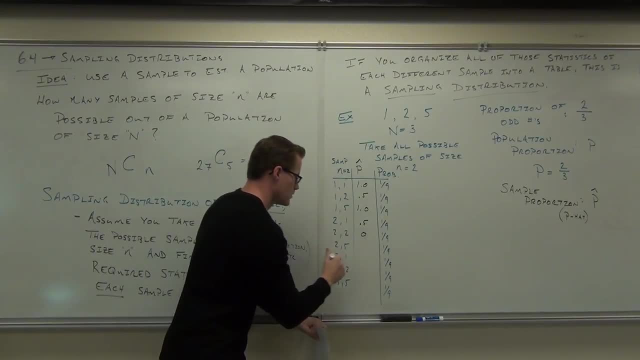 Zero, Zero. How about here? Zero, How about here? How about here Here? 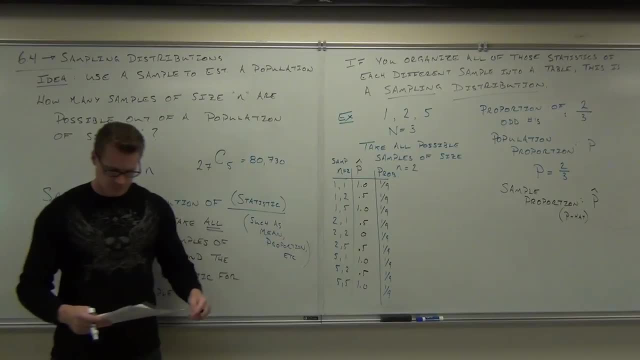 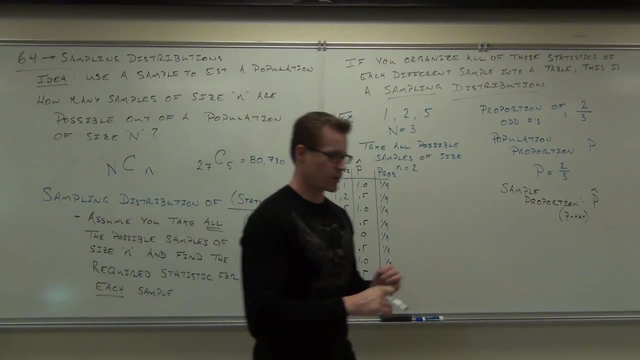 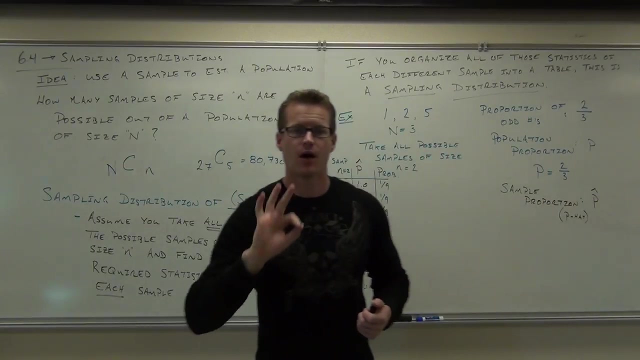 And lastly, we have 1.0.. Okay, we're going to recap for about ten seconds on what we've been doing. We have a population that has only three items in it: One, two and five. The proportion of odd numbers in that population is two-thirds. 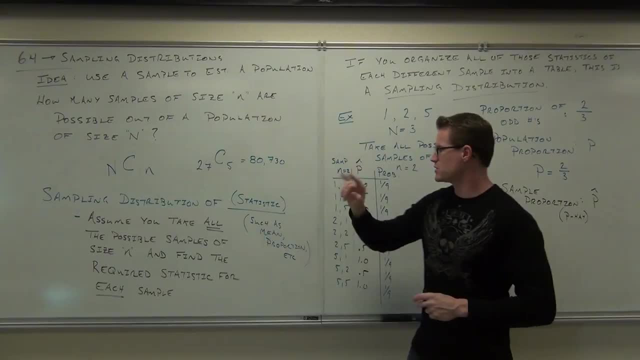 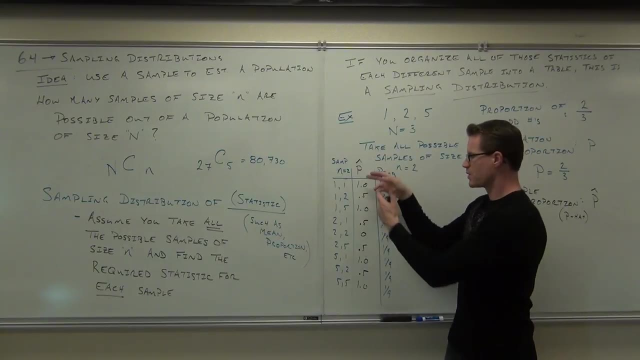 We now took samples of size two. For every sample of size two we listed it out with replacement. The probability of getting any of those samples is one-ninth. The proportion of odd numbers is what we listed out for each sample right here. 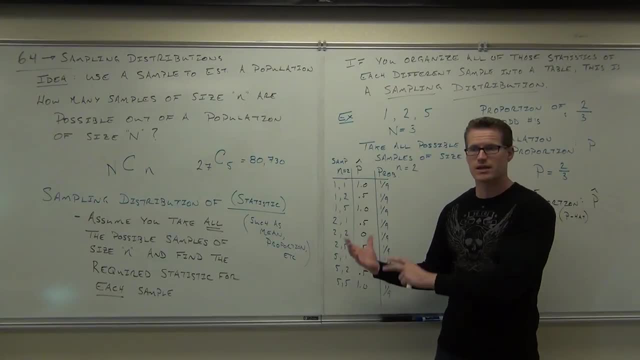 Do you feel okay with what this is? Do you understand that this is a sampling distribution? This is every possible sample of a certain size. That size is two. This is what we're looking for. the proportion of each of those- So that's our statistic in this case- is the proportion. 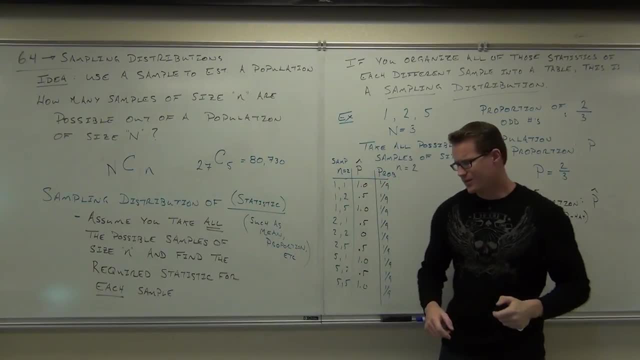 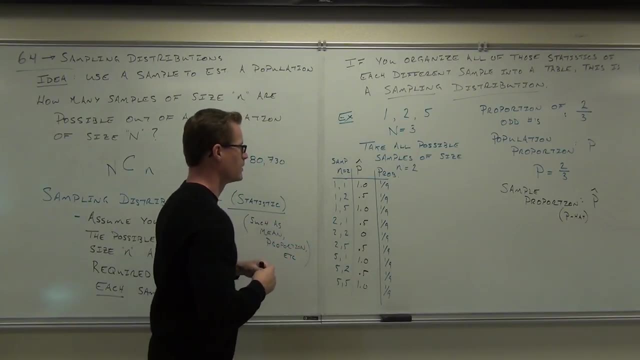 The proportion. right, there is the statistic. Are you with me? Now the question is, as I accidentally erased my two, do my p hats equal my p? Do my p hats equal my p? It's a hard question. Don't mess up the p, I'll get really pissed off. 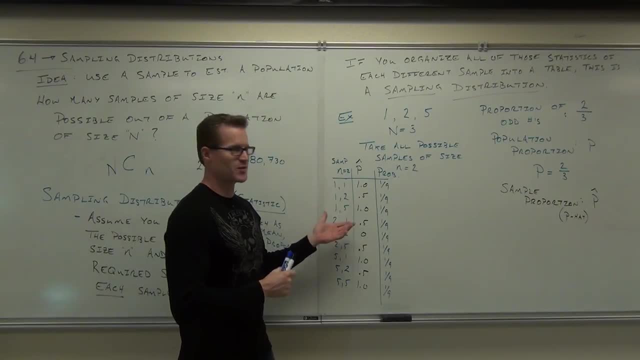 Get it Okay. Okay, That was funny. You can laugh. I heard you laugh. Do my p hats equal my p? Does this p hat equal my p? This is 1.0.. The p is two-thirds. Is this the same? 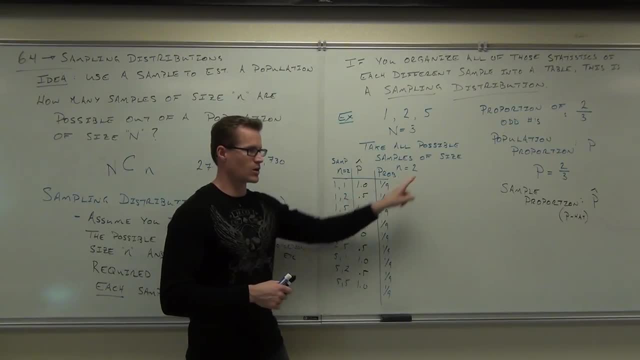 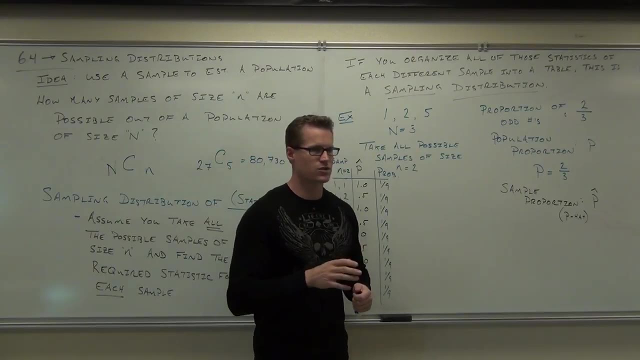 Is this the same? Is this the same? Are any of these the same as our p two-thirds? No, not one of them. Not one of them. However, something really really interesting. This is the key point here for the whole day. 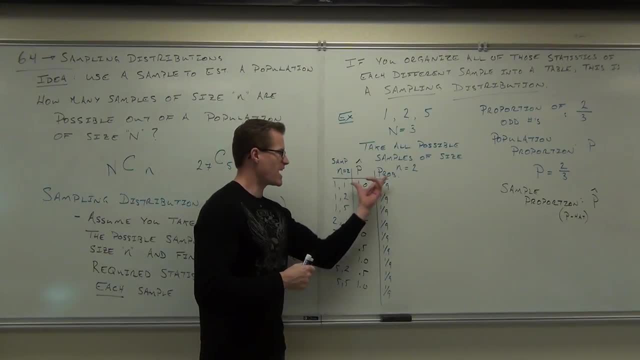 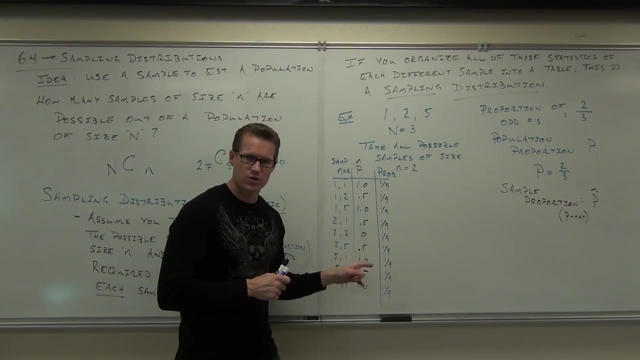 The key point here is that something really interesting is going to happen. if I add this, I'm going to find the average of this situation. I'm going to find the average of this. So, while none of these equals two-thirds, what I want to do is find the average. 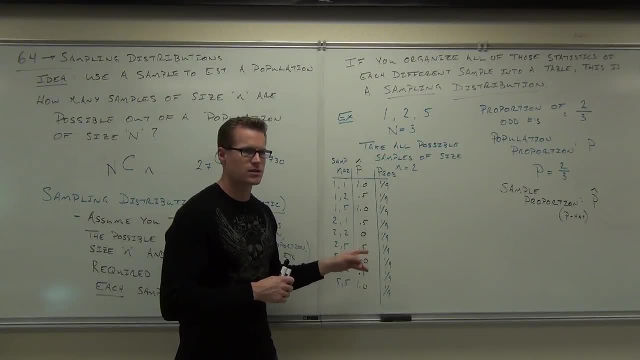 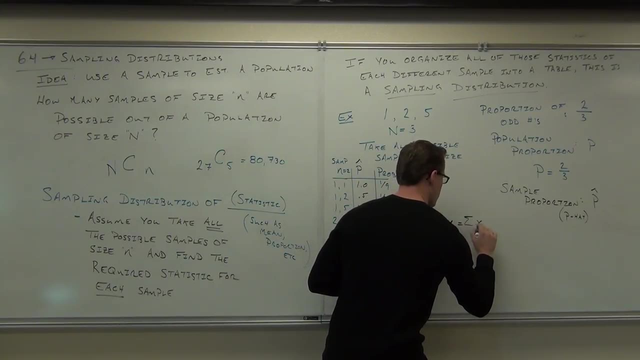 Now, if you don't remember how to do an average of a distribution like this, what you do is you add up the x times the p of x. We're going to treat this as our x, So in our case it's going to be the p hat times the p of x. 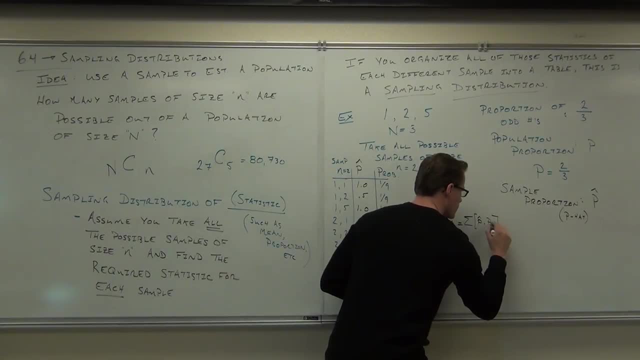 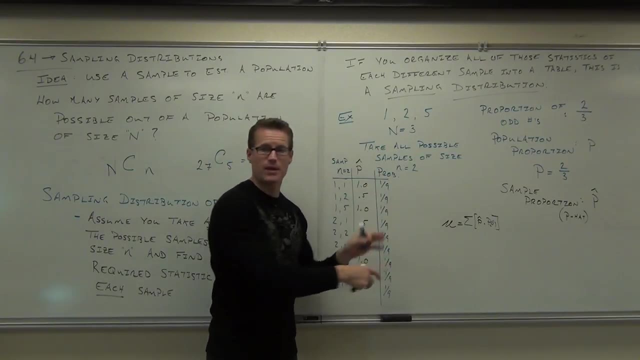 Or the p of p hat. We're going to multiply these things and add that column. That's how you- if you- hopefully you- remember about our frequency distribution. That's how you found. or probability distribution: That's how you found the mean. 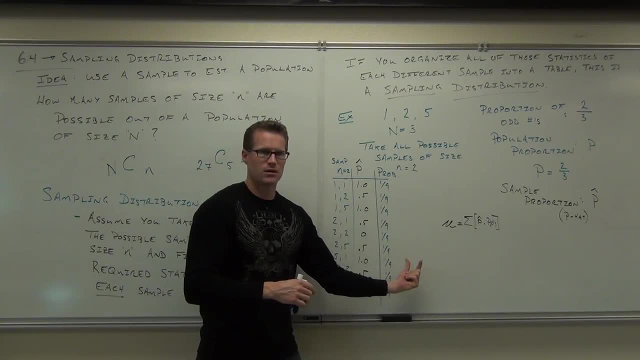 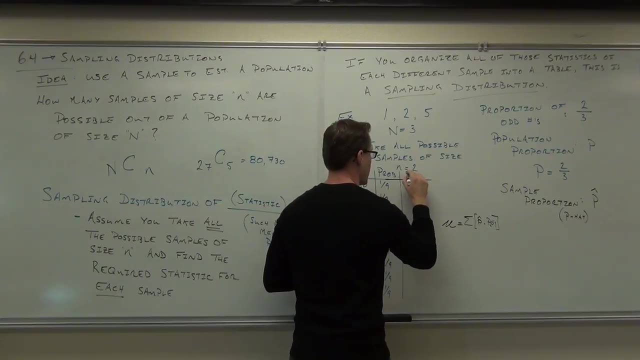 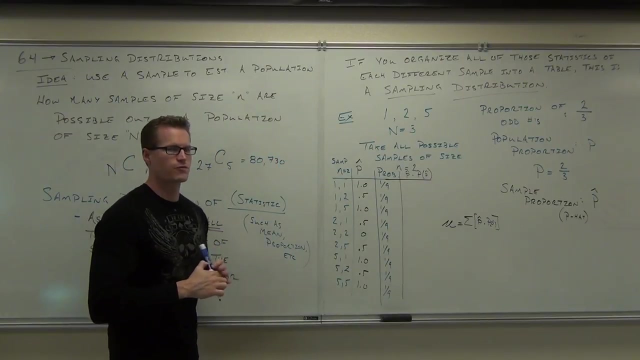 You multiplied these two things and you added that column. Do you remember that? I hope that you do So right here when I extend my column. I'm going to have p hat times, p of p hat. We're going to do some fancy fraction stuff. 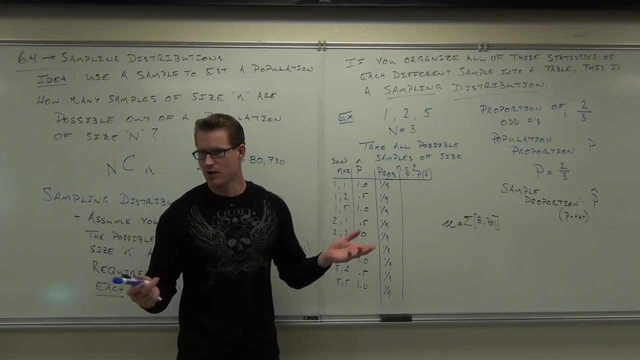 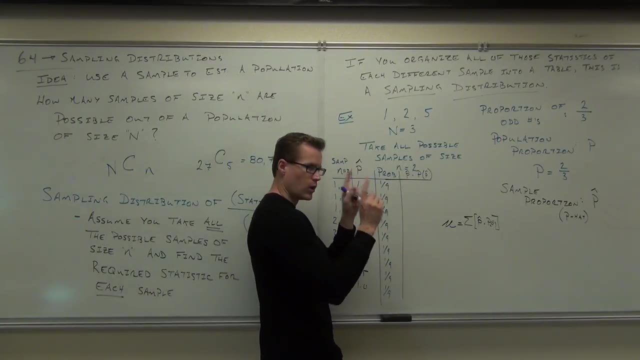 There's only three numbers we need to work with: Zero, I'll take care of the zeros for you. One, I'll take care of the ones for you. And .5, that's the only tough one. One times one, 1.01 times one-ninth, gives you one-ninth. 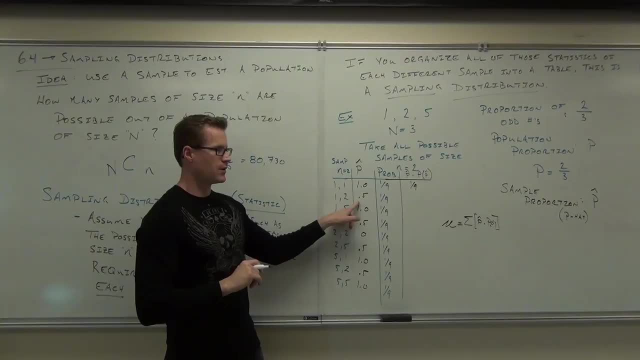 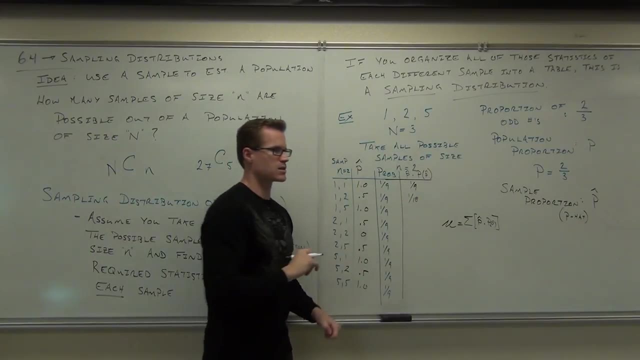 Do you follow Half of one-ninth? you could have left that one-half. One-half of one-ninth is one-eighteenth. You see where the one-eighteenth is coming from. Yes, no, One-ninth divided by two is one-eighteenth. 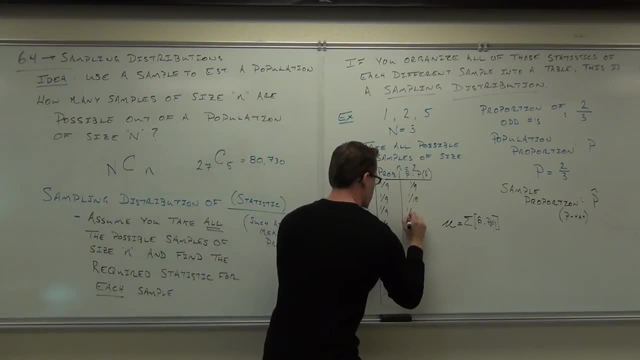 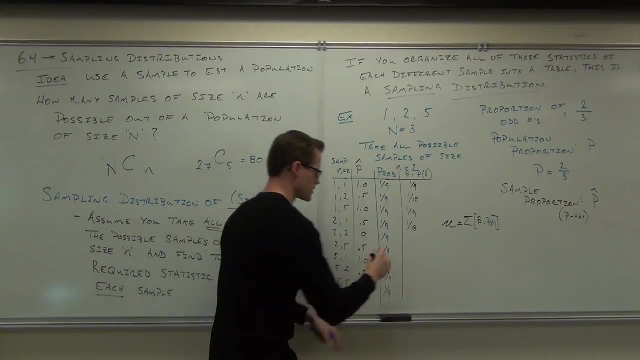 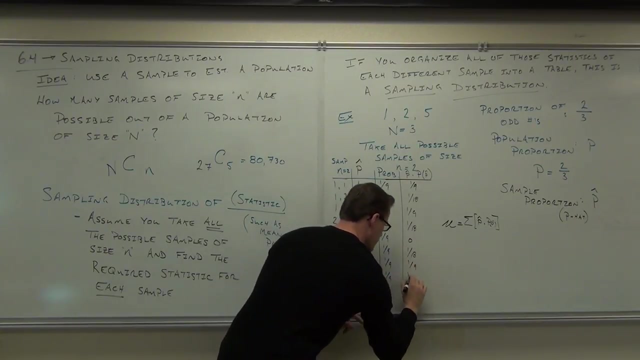 Half of one-ninth is one-eighteenth, This is one-ninth, This is one-eighteenth. This is how much is this? Zero, This is one-eighteenth, This is one-ninth, This is one-eighteenth And this is one-ninth. 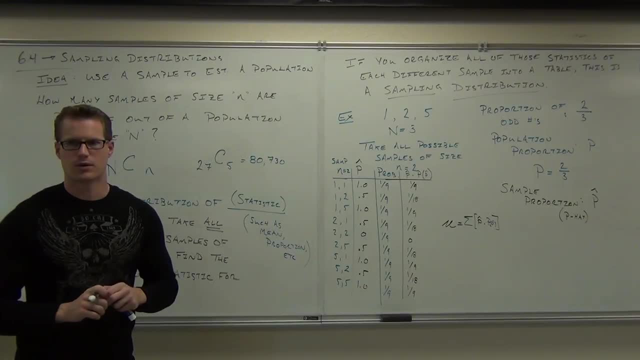 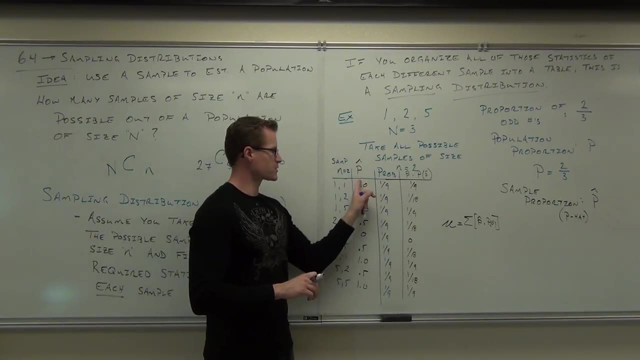 Are you okay with that so far, Are you sure? So we've multiplied this column this one times this one. We've got p-hat times p of x. If I add up this column right here, I'm going to get the average. 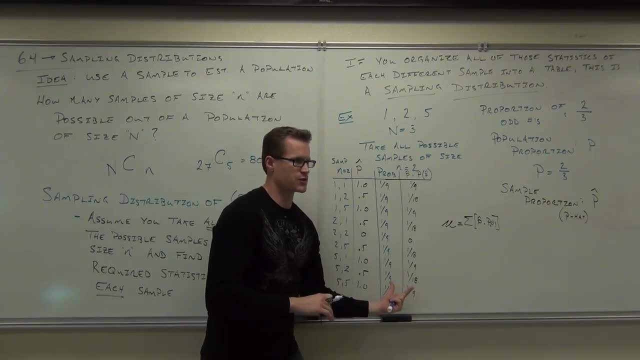 Not sure. if you're all right. Are you sure It's confusing for some people? If you're confused, I need to know. Do you know where these numbers are coming from? One-ninth and one-eighteenth: Do you know that if I add them, I will get the mean? 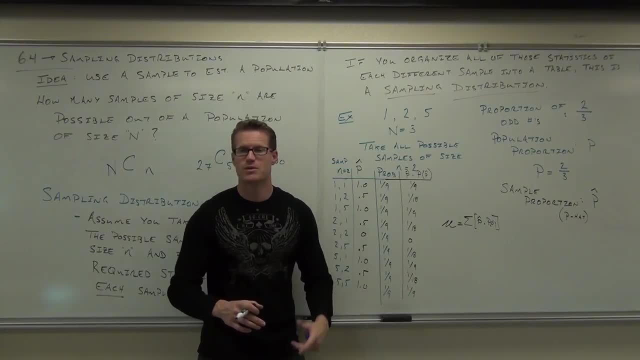 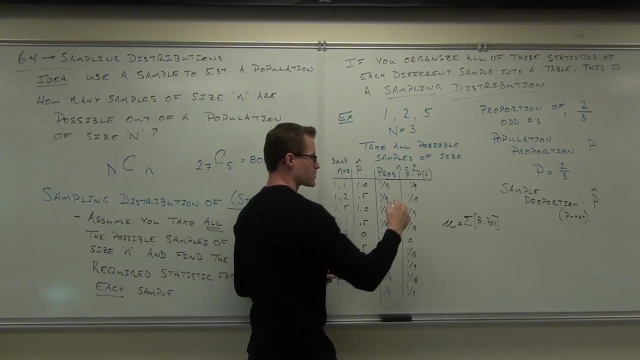 Yes, Just like you did. Yes, Just like any other probability distribution. it's still the same thing, which happens to also be a sampling distribution. If I add this column, let's look at what happens here. This one and this one actually give you another one-ninth. 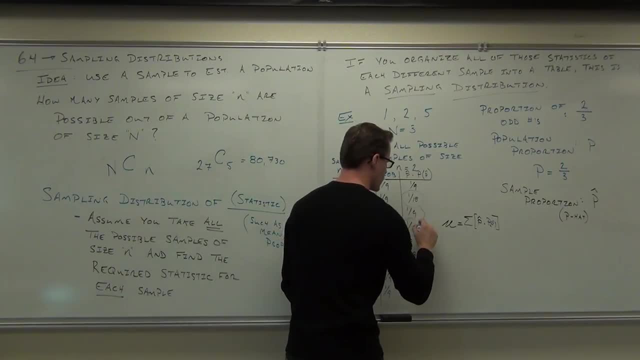 because you'd have two-eighteenths, right, That's going to give you one-ninth. Let's cross that out. This one and this one also give you one-ninth. Let's cross that out, Just to make it easier. here's why. 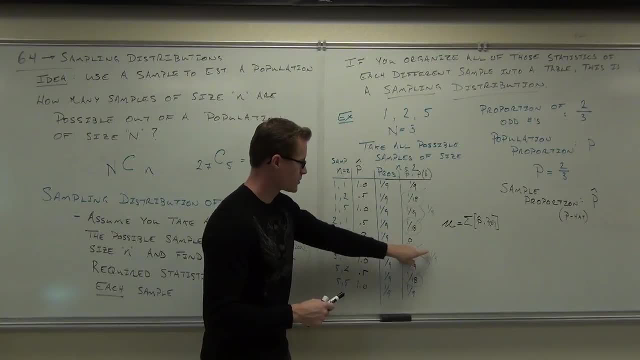 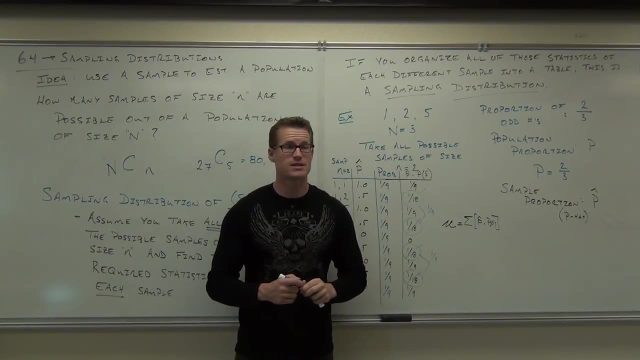 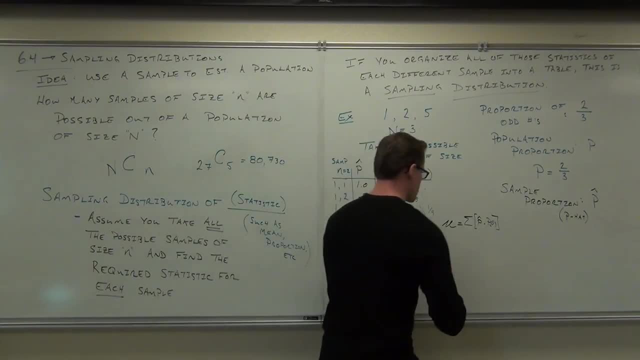 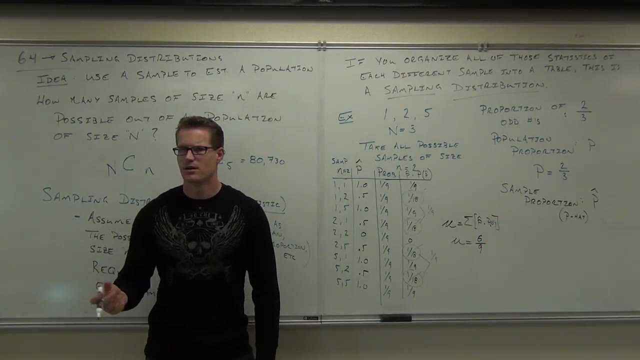 If you don't just add all these up on a calculator, You're going to get six-ninths. So the mean equals six. wait a minute. six, how much is six-ninths? What the heck? I'm Harry Potter and this is my math magic wand, right there. 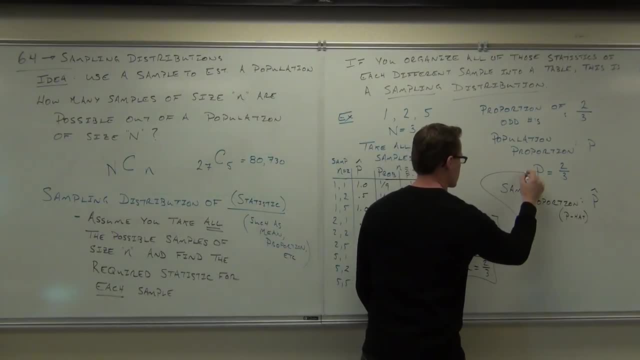 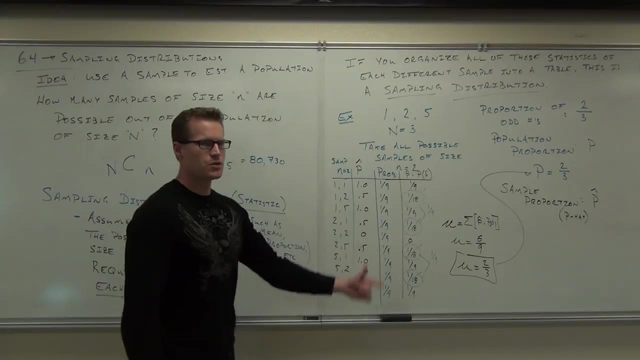 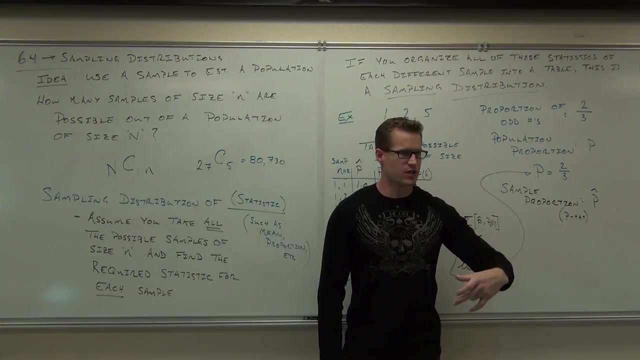 I knew it. Wait. none of these were two-thirds. not one of them. not one of our samples, sample portions had two-thirds, yet when I average them, it equals exactly two-thirds. Is that magic? No, it's actually expected. 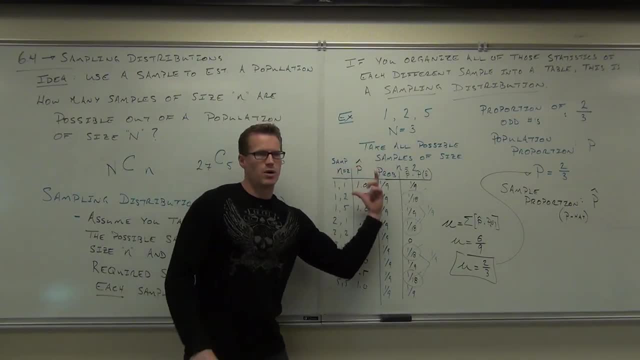 Think about what you're doing. You're taking every single possible sample right, every single one, So sure you're going to get some that are higher, some that are lower, some that are higher, some that are lower. Some of them are way lower, lower, higher, lower, higher, but you're averaging them. 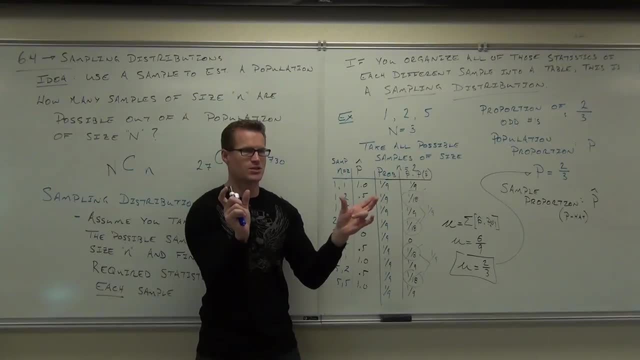 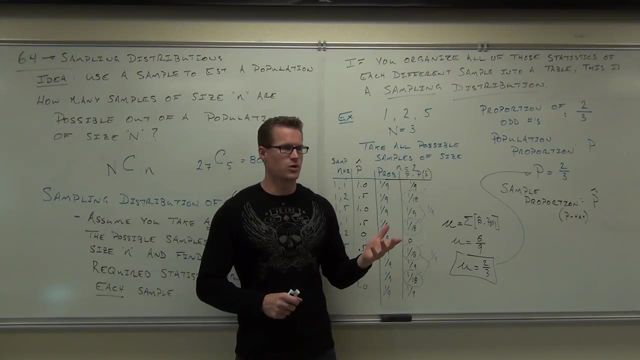 If you add up all the possible samples and you average them, you're going to get exactly what your population originally gave you- exactly it. Now, this might not seem like such a big deal for you, but in our populations we don't just have three things, do we? 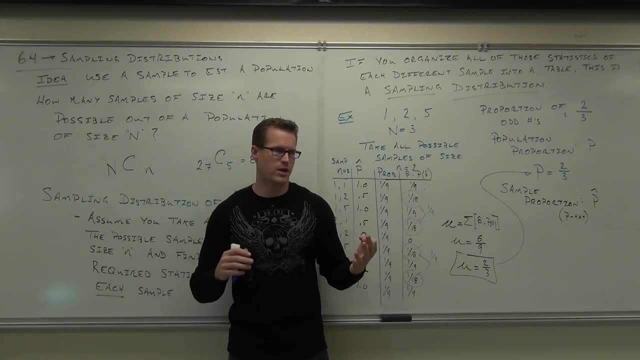 We have like 27 things or we have like a million things, or we have 370 million things, Like in America. that's how many people we pretty much have. It's a lot of people. We can't do this all the time. 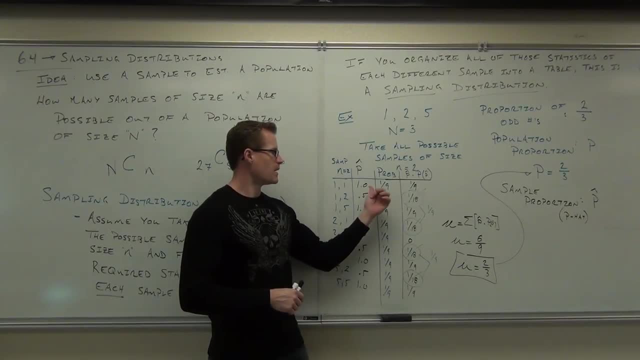 Right, But what this says is, while every sample does not give you the population proportion, the average of all the sample proportions will give you the population proportion. In other words, sample proportion targets. that's a key word for us: targets, population proportion. 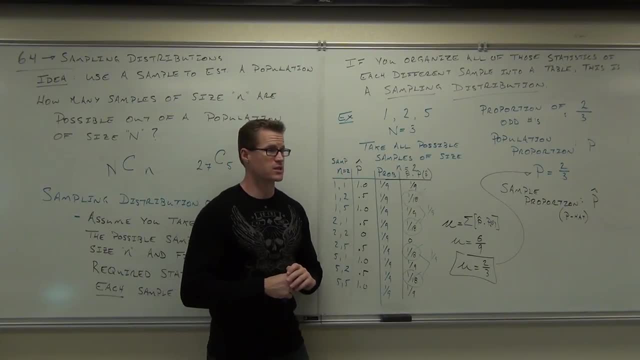 It doesn't systematically overestimate it or underestimate it. It will be around it. Now, with a sample size of three, yeah, we're going to be way off, But with a sample size of more than 30, we're pretty much right on the money. 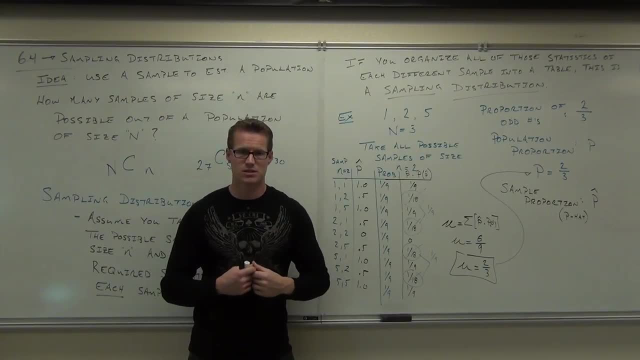 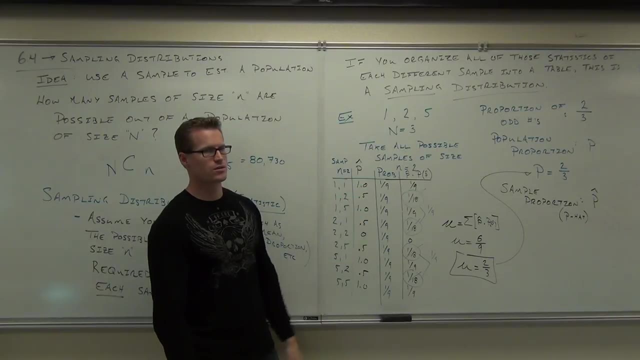 Or we're really, really, really close. So as our sample size increases, our ability to target the population proportion is increased as well. So, while this one's over, this one's under. While this one's over the two-thirds, this one's under. 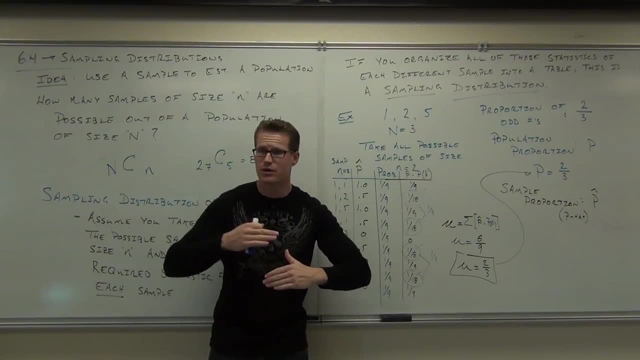 It's not doing all over. it's not doing all under. Some are over, some are under. It's not systematically doing any one thing. We call that targeting. If I take the average of them, it is exactly the same thing. 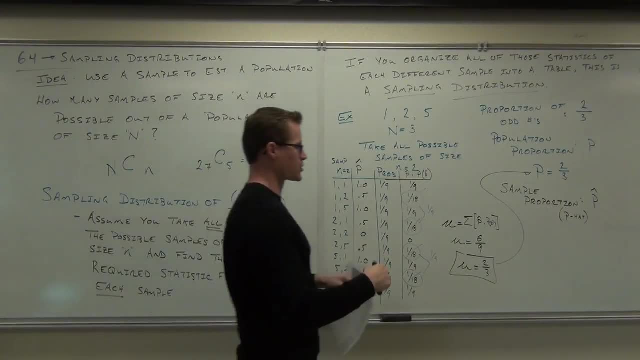 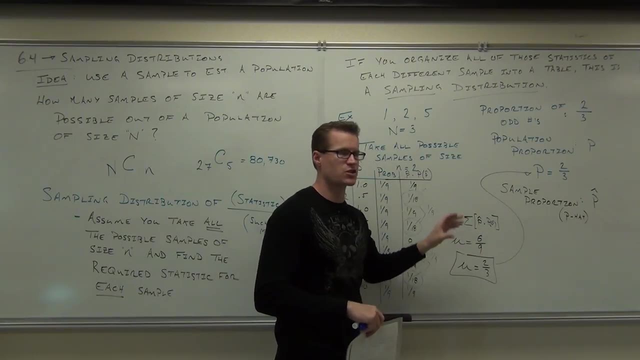 So what we would say is that this shows us that we're going to be able to target the population proportion, Is that this shows that sample proportions- the average of our sample proportions, equals our population proportion. That means that our sample proportions target our population proportion. 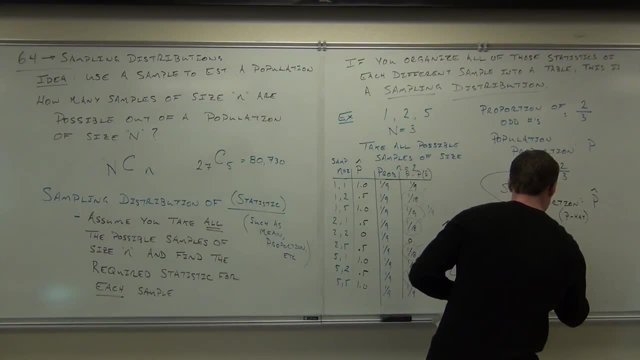 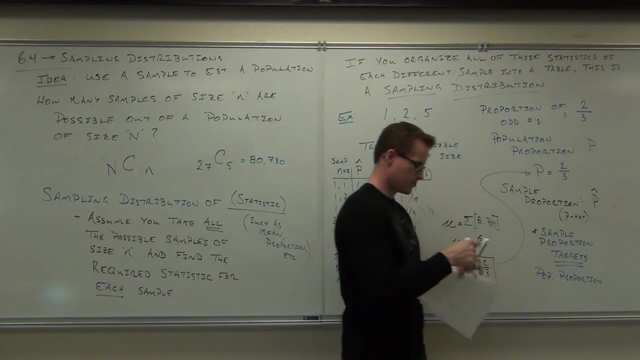 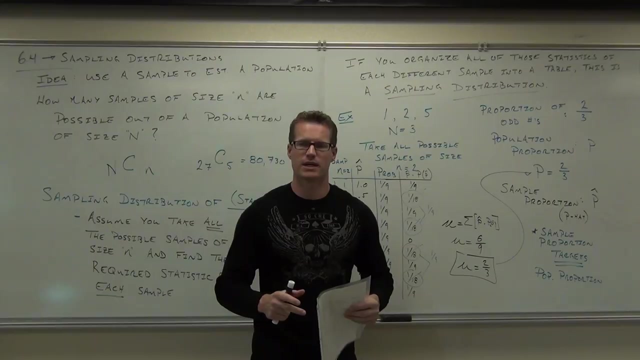 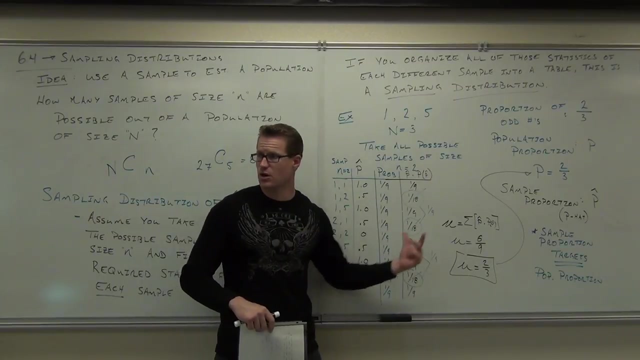 Right there. If you're still not quite getting why this is important, we've just proven- you do follow me- that this is targeting it right. Find the average. I mean it's giving you the same thing. It's not systematically over or underestimated. 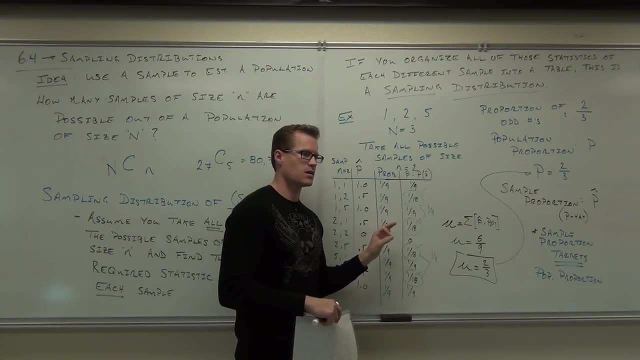 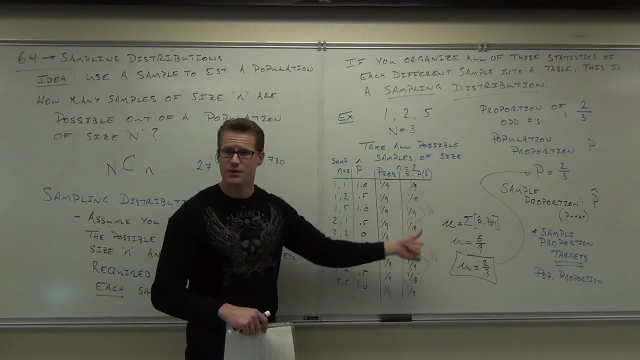 That's what target means. If we have a statistic that targets a parameter, or in other words, something about our sample that targets something about our population, this says that the sample statistic is a good estimator for the population proportion. This is showing that, while this is not right on the money, it's going to be close enough if our sample size is big enough. 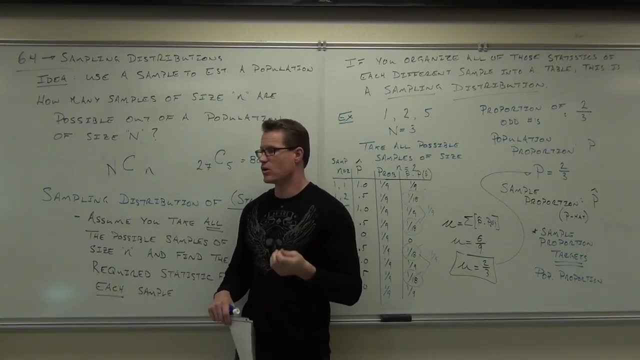 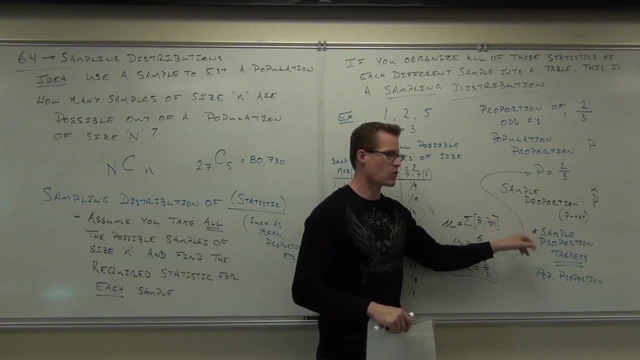 While this is not exactly accurate, it's going to be a good estimator overall. So what this says, the sample portion targets population proportion, or in other words, we can use a sample proportion as an estimator for population proportion. So targets and estimates pretty much synonymous in this case. 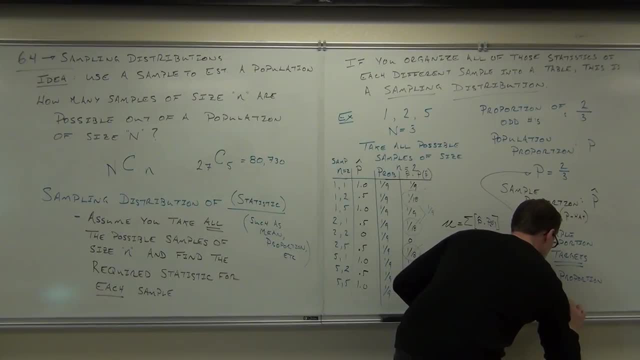 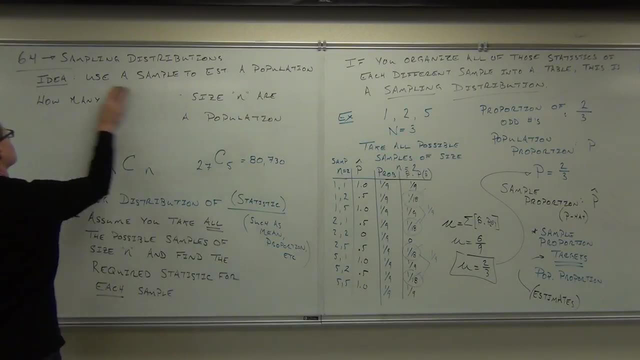 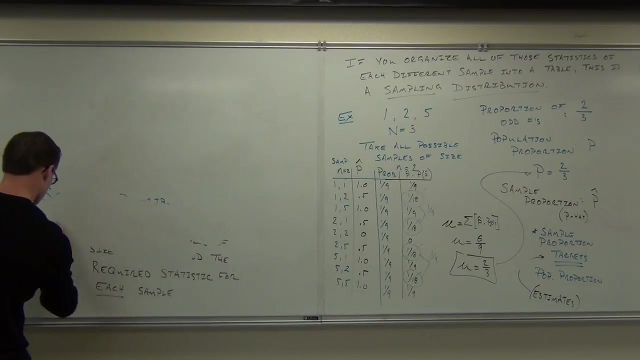 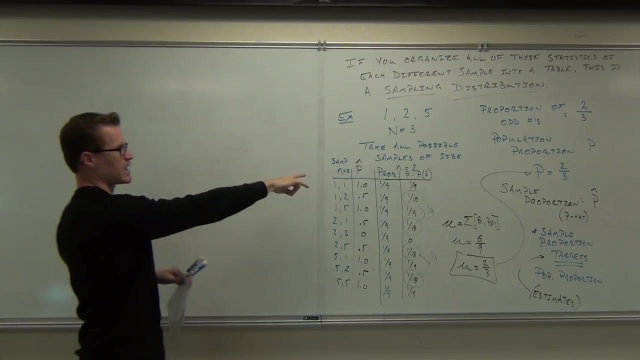 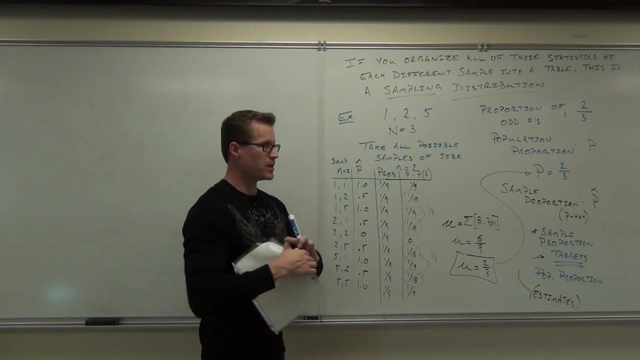 So this right here is a sampling distribution of the proportion. That's what that is: sampling distribution of the proportion. What we're going to do right now is construct another one for the mean. I'll show you that, and then it'll be all our day. 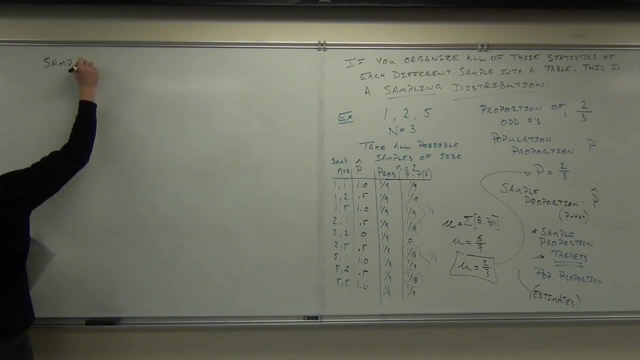 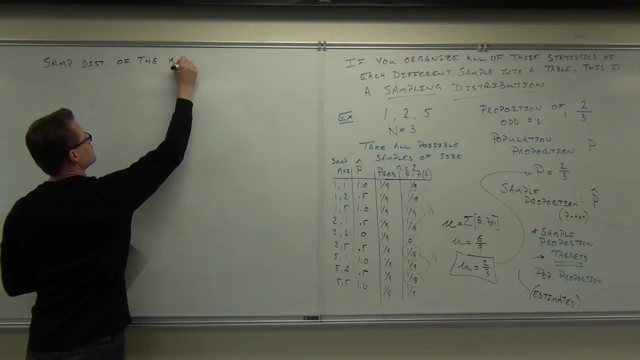 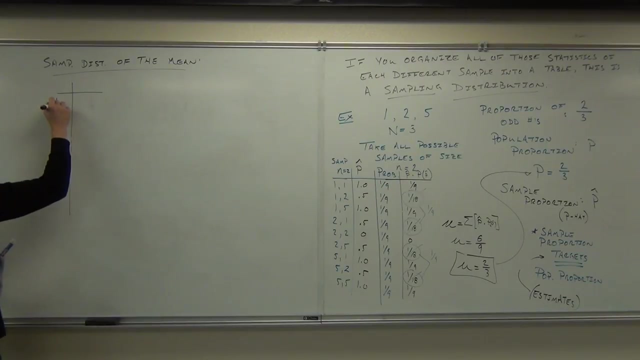 So let's do a sampling distribution of the mean Same idea: 1, 1.. Let's do that: 1, 2. 1, 5.. 2, 1., 2, 2., 2, 5.. 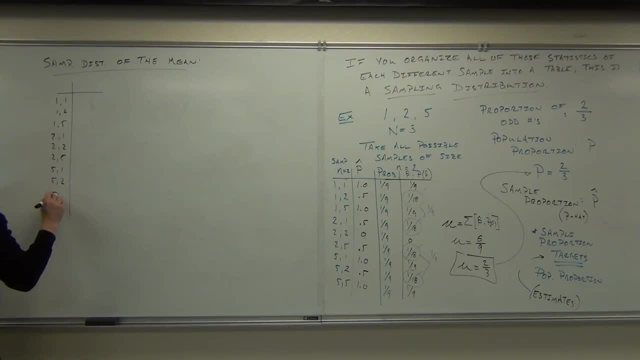 5, 1.. 5,, 2., 5, 5.. These are our samples of size n equals 2.. This is my probability. They're all going to be 1 ninth, 1. 1. Uh-oh. 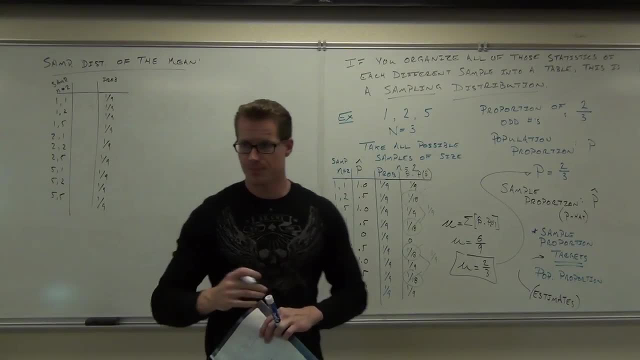 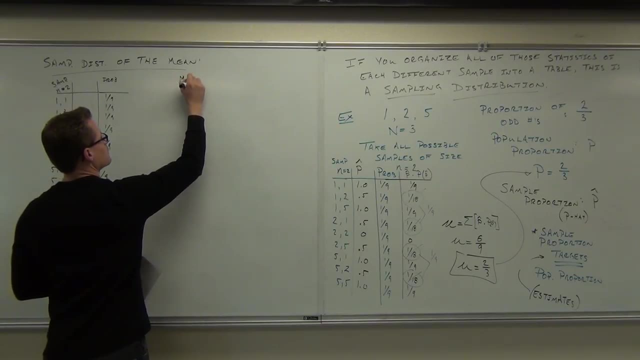 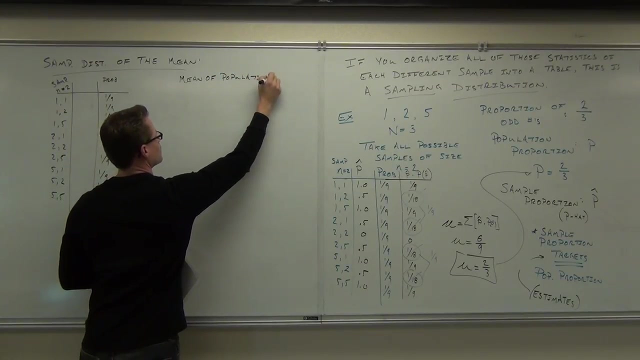 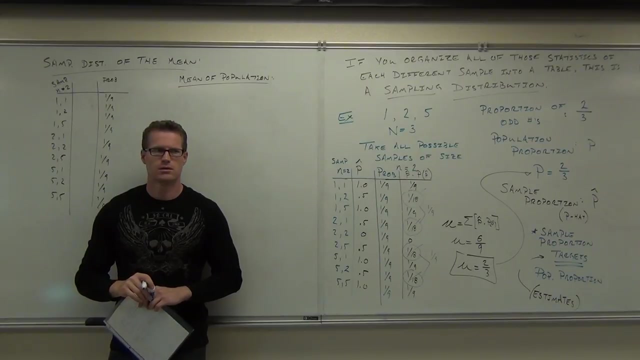 But now, instead of dealing with the proportion, I want to look at the mean. Oh, by the way, what's our population? again, What was that? No 3. Population is 3?? Yeah, That must be the population's size. 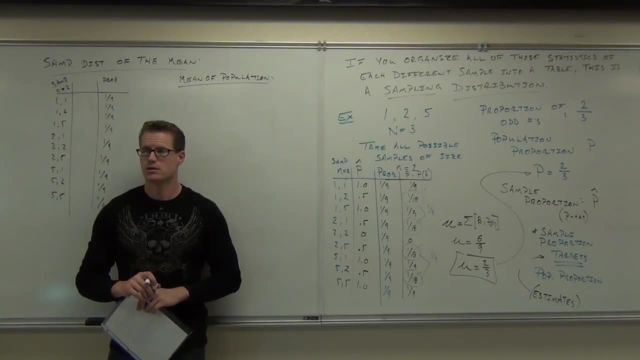 Yeah, What is the population? What is it? Two-thirds, Two-thirds, Two-thirds- that would be the population proportion. What's the population? What are the things we're dealing with? folks, What are the only three numbers in the world? 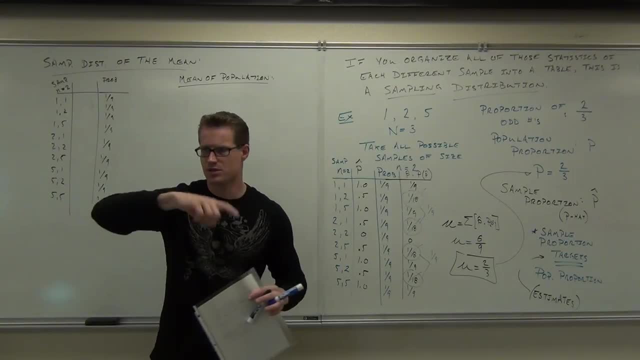 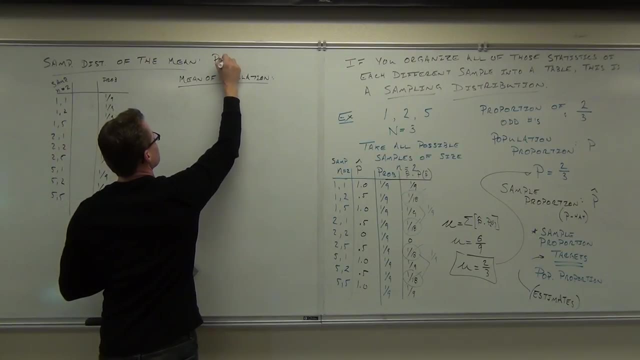 That's your population. The population of this class is the people who are in this class. The population we're dealing with is one, two and five. Population is one, two, five. that's it. There are three items in our population. 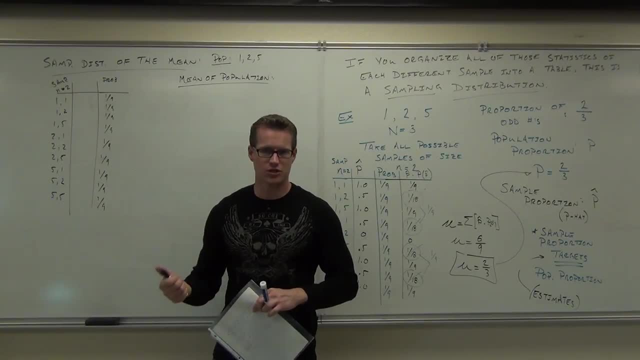 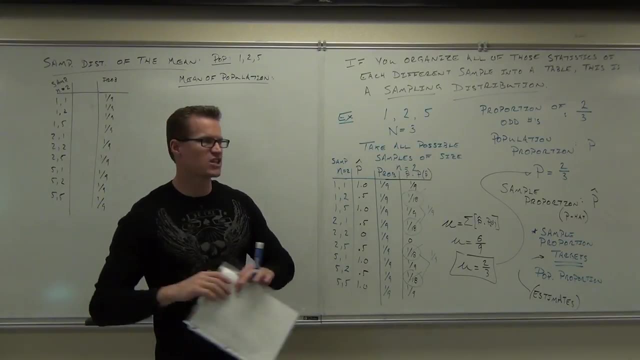 The proportion of odd numbers is two-thirds, but our population is one, two and five. It's one, two and five. You with me? Yes, Now what I want to do is forget about the proportion right now. This was one example. 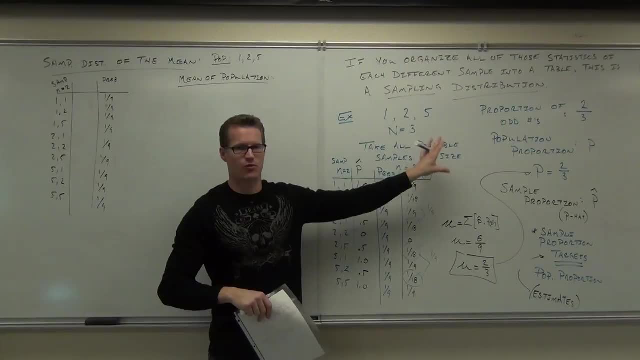 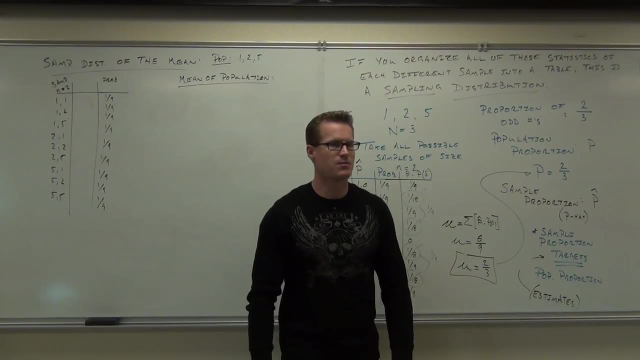 This is a different example. This is not related to this one in any way. shape or form You okay with that New example? We're now talking about the mean. What I want you to do is find the mean of your population. 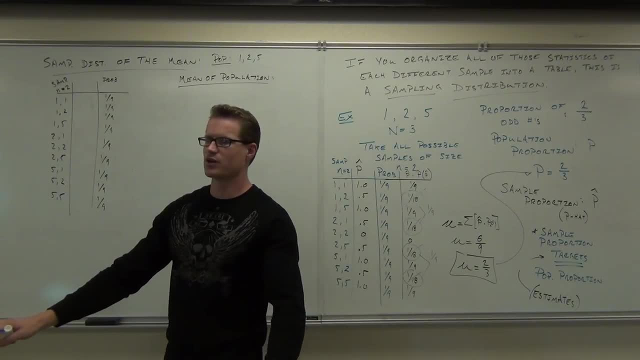 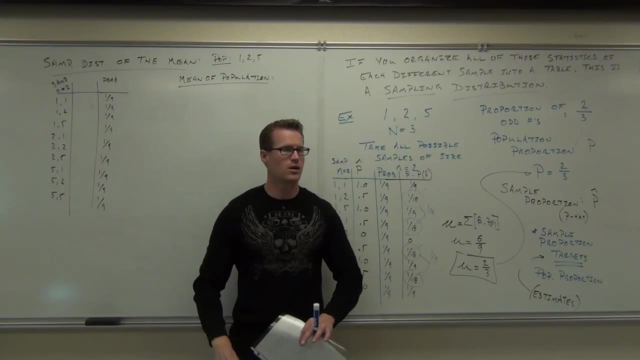 Find the mean. It's only three numbers. You all look at me like I'm crazy or something and you're confused. How do you find the mean? Add them all up, Cool. Add them all up. Divide by the number you added. 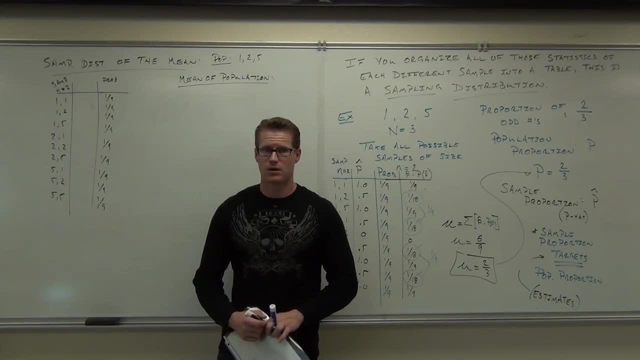 What do you get when you add them all up? No, you don't. You get eight, You get eight. And what are you going to divide by Eight? Eight, Eight, Three, Three. You're going to divide by three. 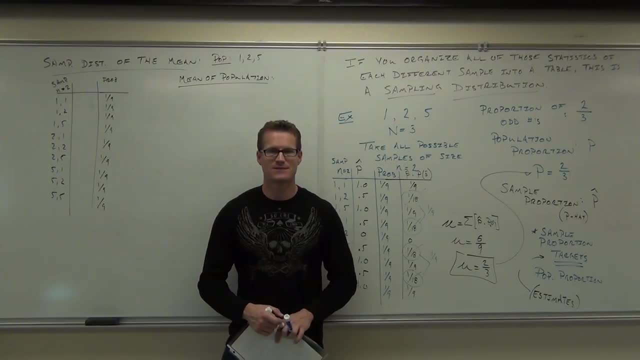 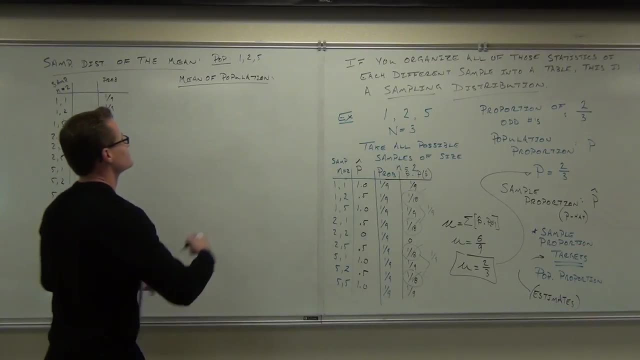 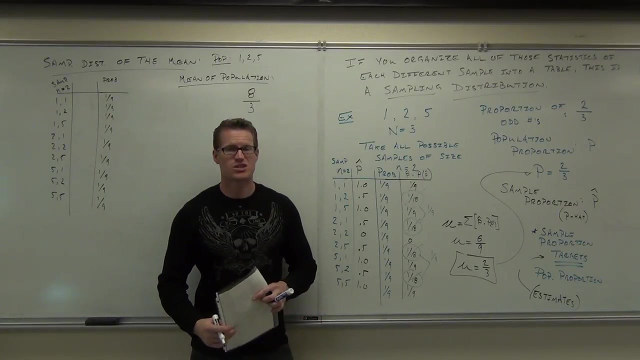 What's the symbol for population mean that you're going to use? Wow, All right. Do you agree that your mean is going to be eight-thirds? What's the symbol for the mean? This is not a confusing question. This is something you've been doing since the first day of class. 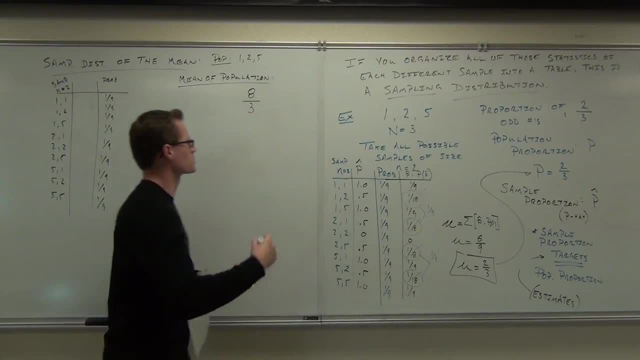 What is the symbol you use for the mean of a population? New, Yeah, That's a good question. The mean for the population here our mean is eight-thirds. You add them all up, You divide by the number you added. 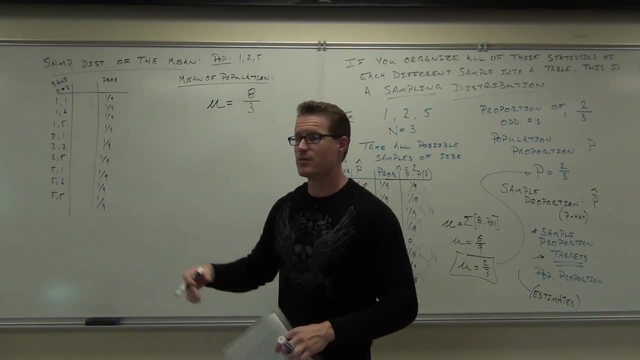 You okay that our mu is equal to eight-thirds? Remember, you are not dealing with P anymore. Ignore this example. We're learning something new, A whole new game, A whole new ball game. We're talking about the mean. now You find the mean, which. you know how to do that. 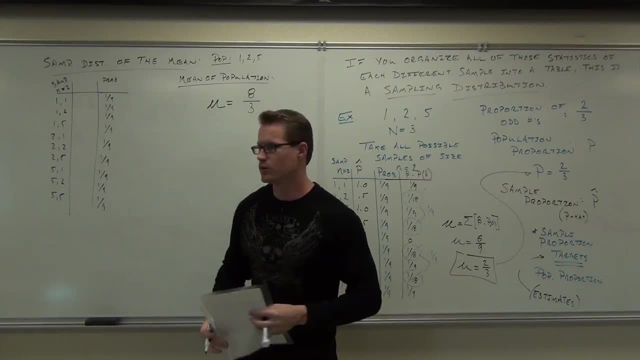 It was on your very first test. The mean for the population is labeled mu. We get eight over three. We added them all up. We divided by the number you added, You get eight-thirds. What we're going to do now is, for every sample, we're going to divide by the number you added. 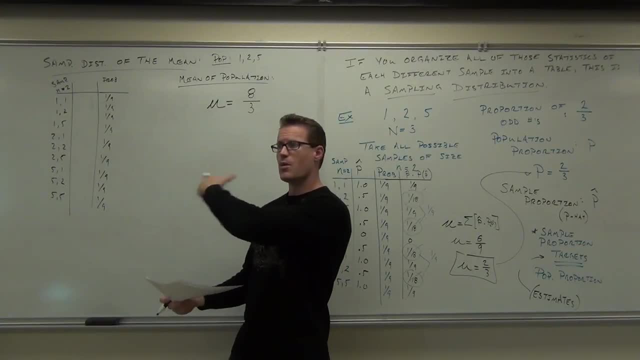 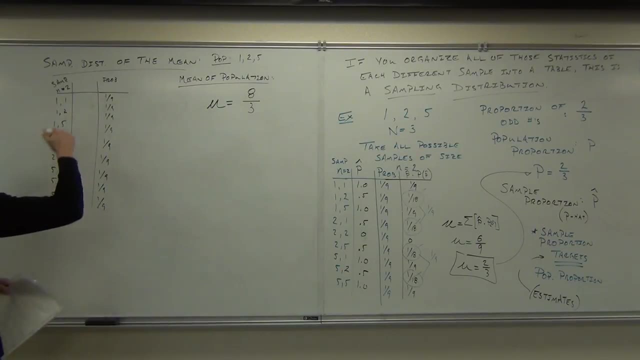 We're going to divide by the number you added, You get eight-thirds. The mean for the population is labeled mu. We get eight over three. We added them all up. We divided by the number you added, You get eight-thirds. What we're going to do now is for every sample we're going to find the mean. 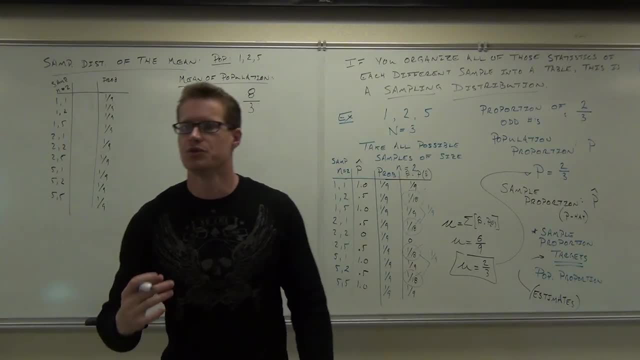 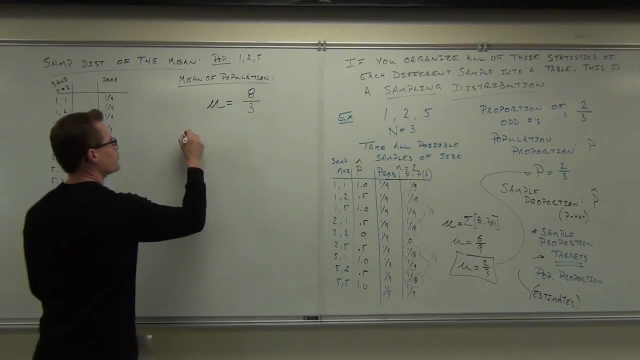 Now, what symbol do you use to represent the mean of a sample? It's not mu, Mu is for population. What do you use to represent the sample mean? X-bar, Say that again. X-bar, X-bar, Remember X-bar. 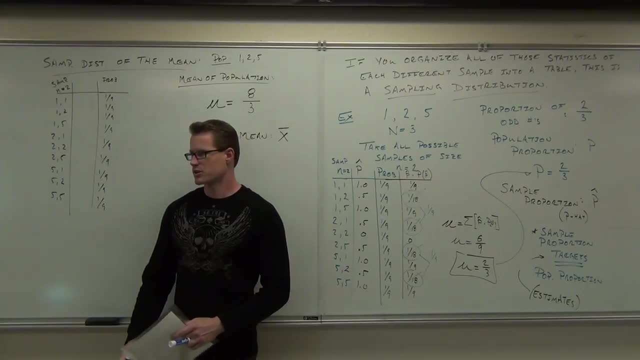 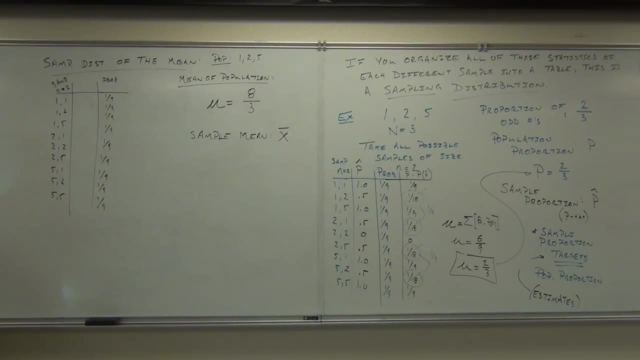 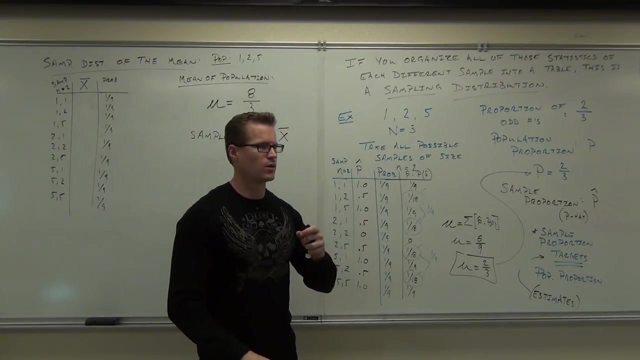 X-bar. We've rarely used X-bar because we've been dealing with populations so much, But X-bar is going to come back at us. What we're going to do is calculate X-bar Again. what does X-bar stand for? The mean? 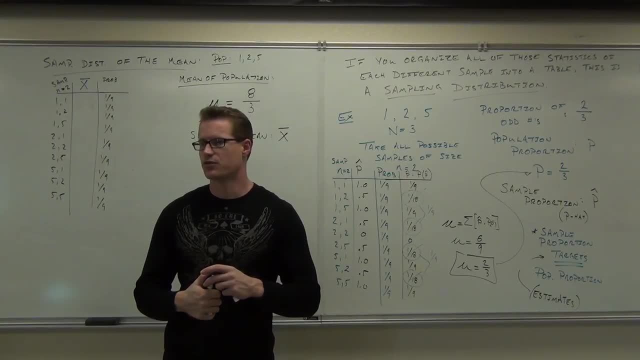 Don't just say the mean. You've got to be specific. The mean Good, What's mu stand for? Population- Are they different? Yes, One deals with a little sample. One deals with a thing. The population mean for ages in this classroom is going to be one thing. 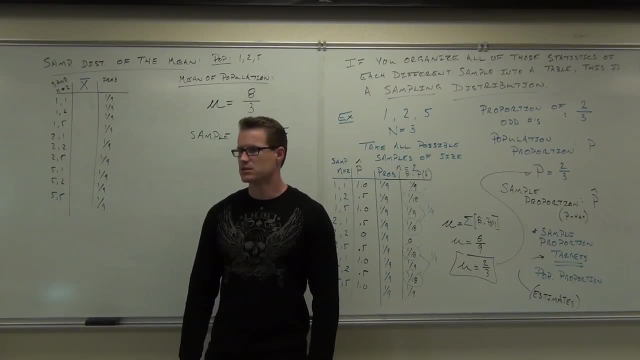 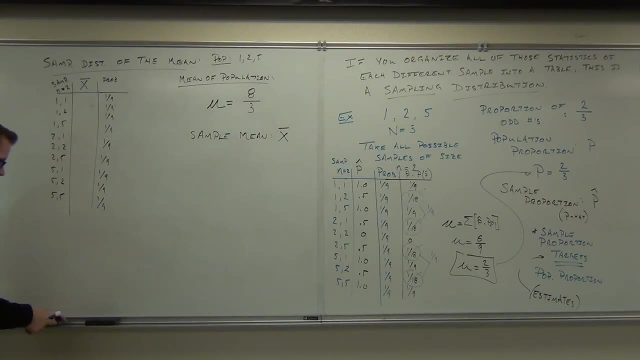 The sample age of these five people is going to be a different thing, right? Generally it's going to be different. Let's find out the mean for each of these. for each of these samples, The mean is: you just add them and you divide by the number you added. 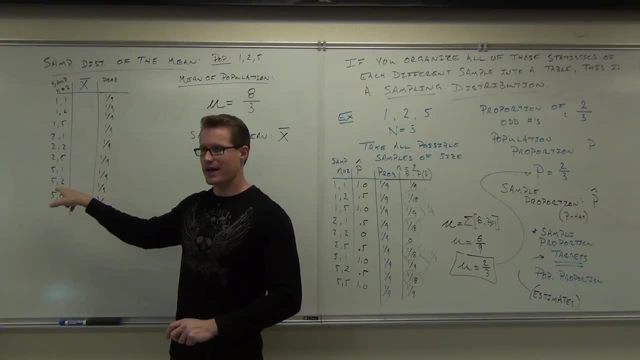 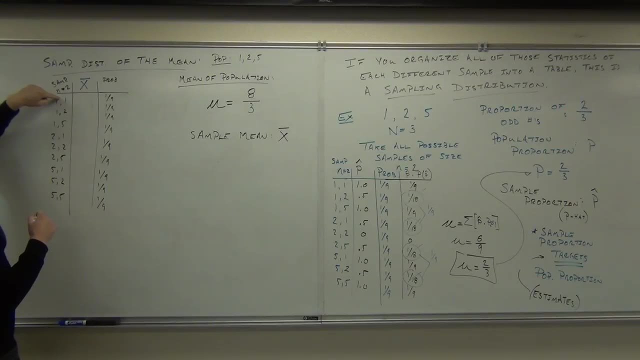 How many are we adding? in every case? Two. So we're going to be dividing by two. So we have what's the mean of one and one, Two, Two. How much is it? It's one, It's one. 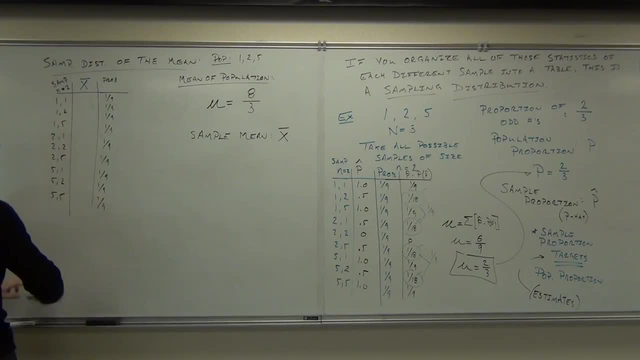 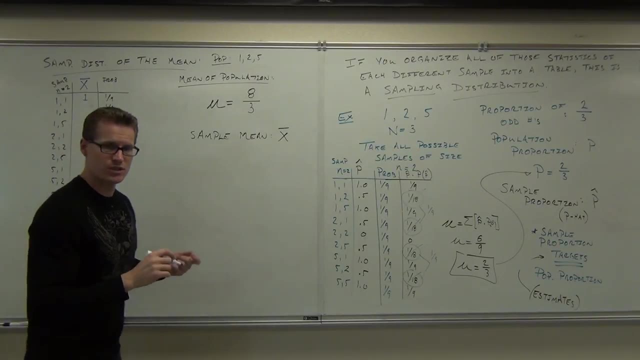 Sure, You add them up, You divide by two, You get One. What's the average of one and two? Three over two, Which is Five. What's the average of one and five? Six over two, Six over two. 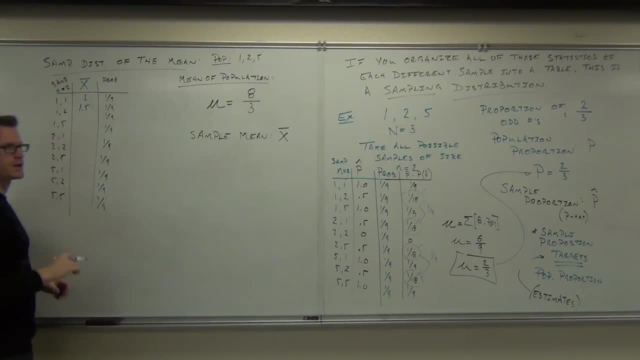 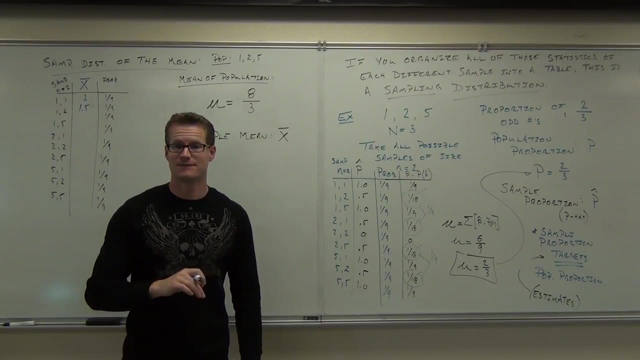 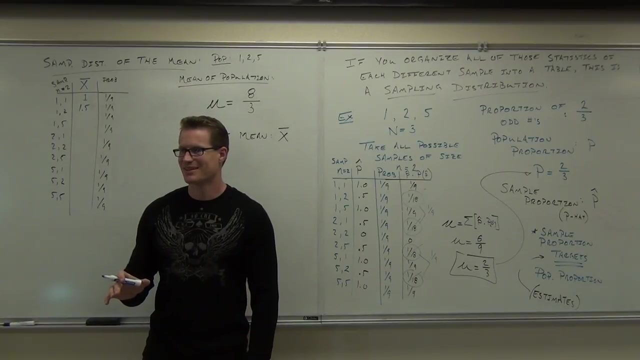 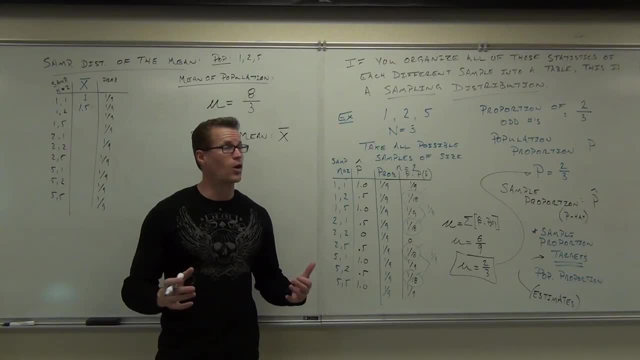 Let's just get it. I'm getting eight out of ten Great. Are you sure I gotta to have you here? I gotta have you with it. If not, you need to let me know. I can go back and cover this again. 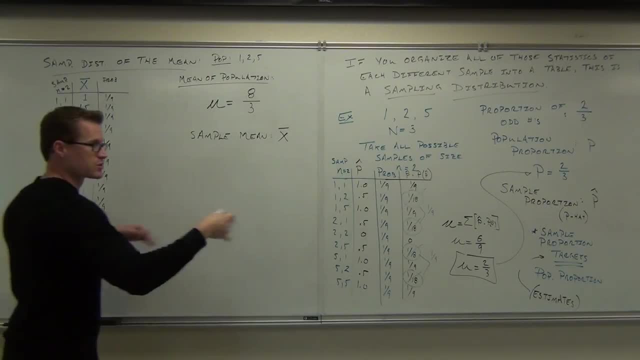 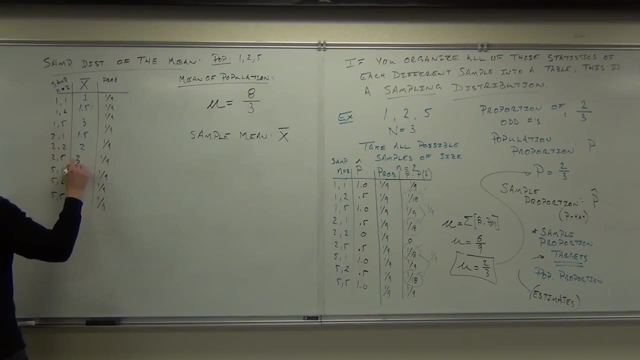 Are you understanding where the one and the 1.5 are coming from? Yes, You're just averaging these things. So averages means, sample means in this case, but so means Three: one point five. Two, three point five. 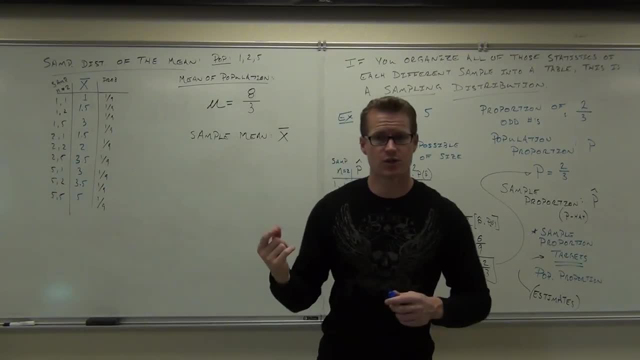 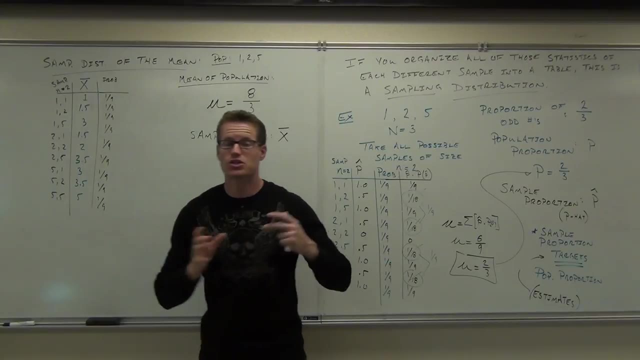 Three, three point five. I didn't make them up. I've averaged each of those numbers and added them all and divided by two in my head. How many of you feel okay with getting that far? Good, alright, Now, just like we did over here, this is going to be a little different. 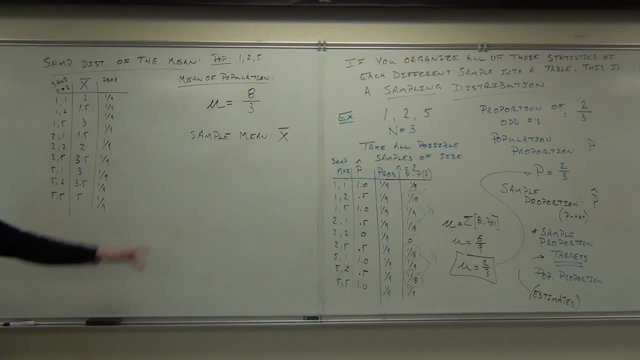 We are going to find the average of these things because I want you to notice something. Eight thirds is 2.66666 forever. Are any of these averages 2.66666 forever? No, But look at them. Some of these are below 2.66, below, below. some are above, above, below, below, above. 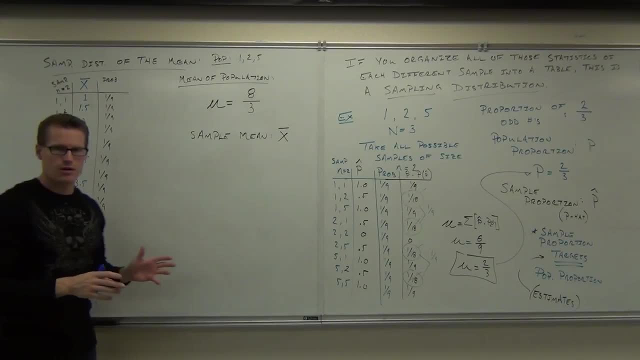 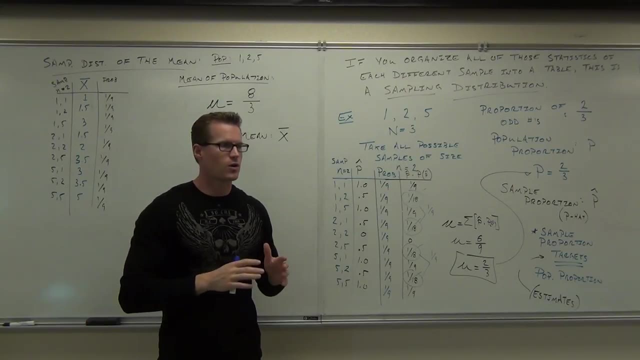 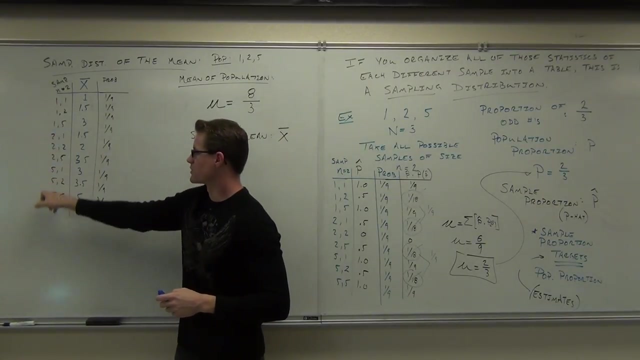 above, above, above, some are below, some are above. It's not systematically above, It's not systematically below. Some are above and some are below. We're going to go ahead and average these averages. So again our idea for sampling distribution. do you agree? this is every possible different. 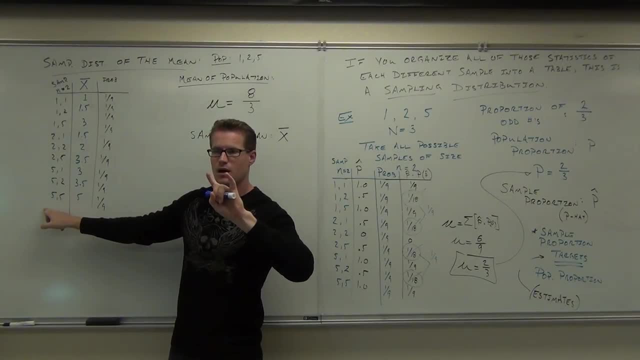 sample of size two. We found the mean of every different possible sample. Simple sample size two. we've put it in a table. This is a sampling distribution. It's a distribution of all the sample means. You guys with me, That's what it is. 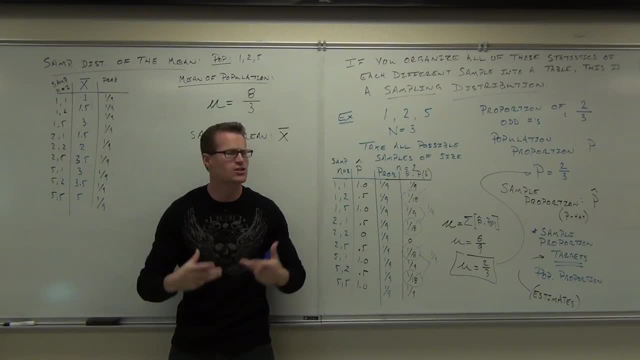 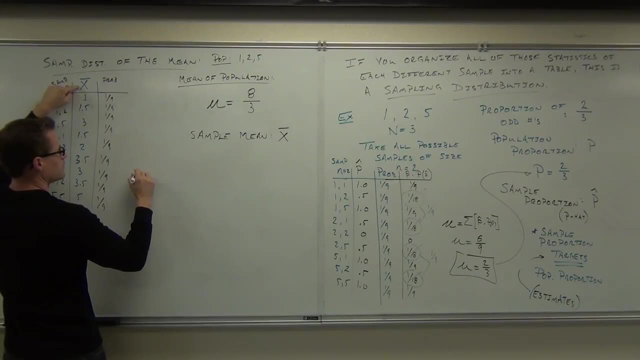 We're now going to average. these means We're going to average the averages- How you average averages in this case, by the way, I'm cheating on the symbol. we'll talk about that in a while. We're going to do that. 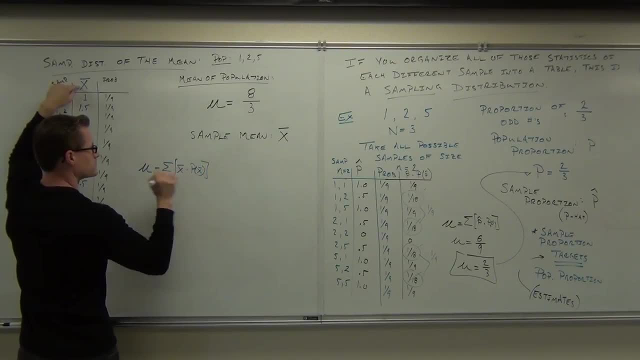 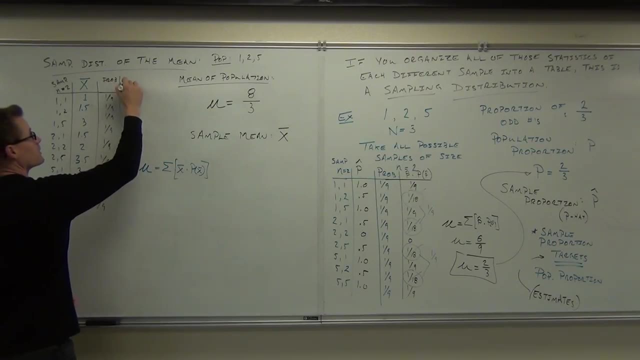 We're going to go ahead and we're going to calculate x-bar times, p of x-bar, Or in other words, sorry, p of x for our sample, x-bar times, the probability of each sample occurring. Oh, we get one-ninth. 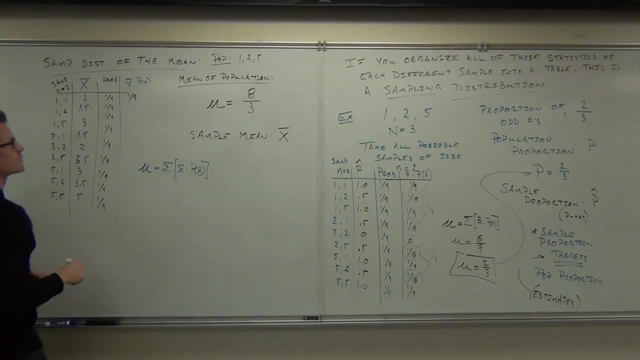 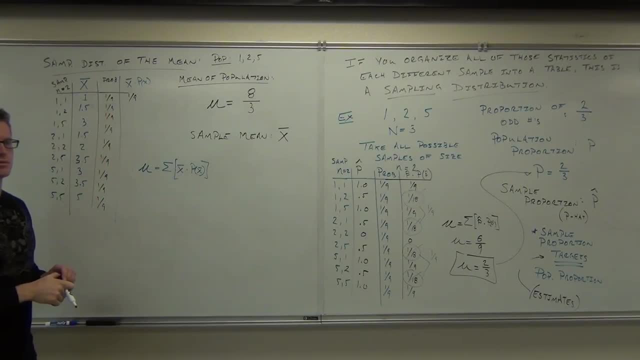 Where am I lying? Am I right? 3 eighteenths. So yeah, we're multiplying Here. you're going to need 3 ninths, 3 eighteenths, again 2 ninths. Let's see. 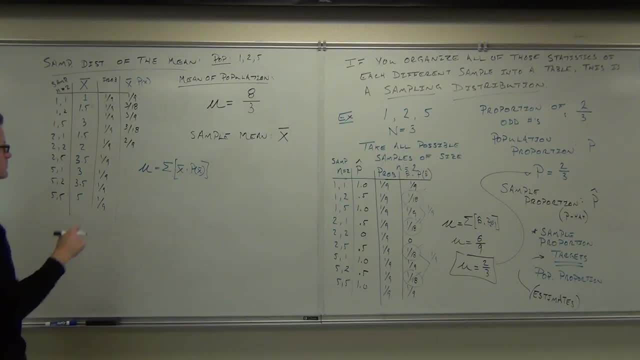 That's 7.. Come on Eight-eighths, three-ninths, seven-eighteenths and five-ninths. Might have been a little bit easier to leave those as fractions, but that's okay. Do you see where the fractions are coming from? 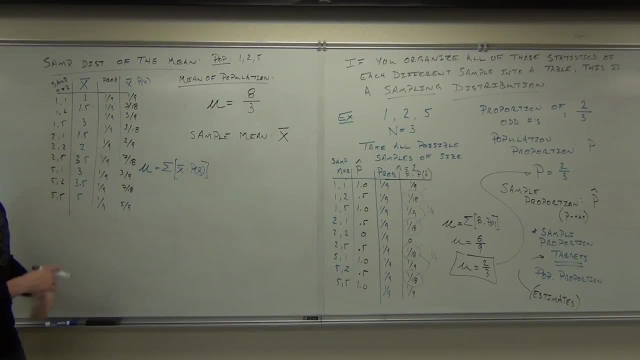 I'm simply gonna find these two numbers together to get those. If I add all those up, maybe do a little bit of conversion here. change all these into eight-eighths, if you'd really like to, This would be two-eighteenths. 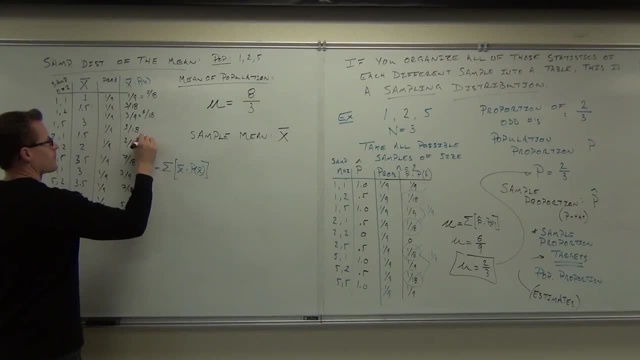 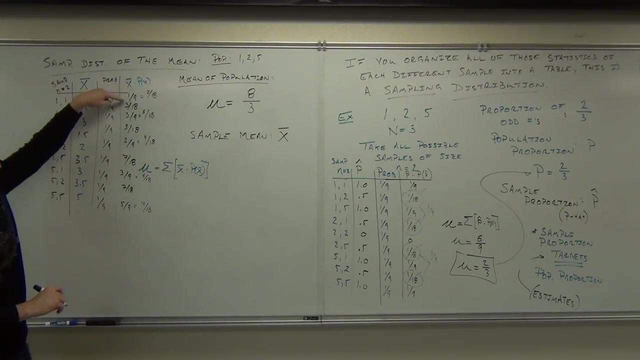 This would be six-eighteenths. If I add these, I get two plus three, that's five. Then I get 11,, 12,, 15,, 14,, 18,, 25,, 31,, 38,. 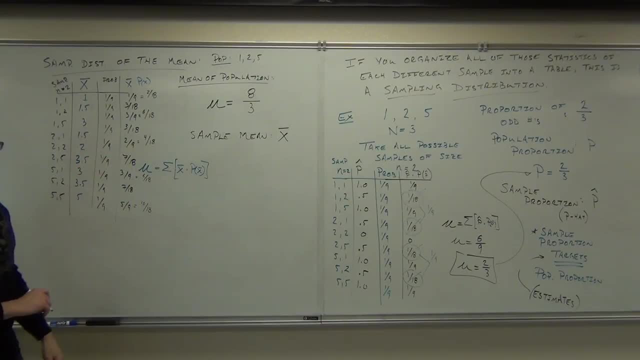 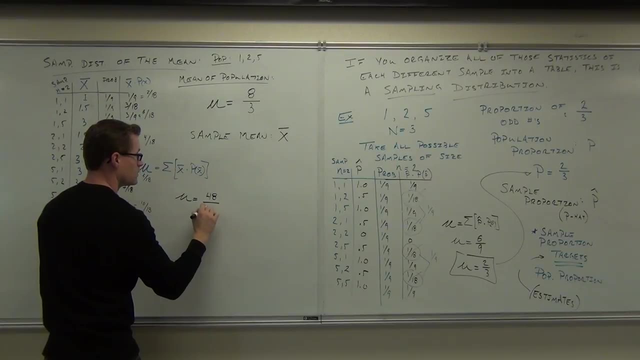 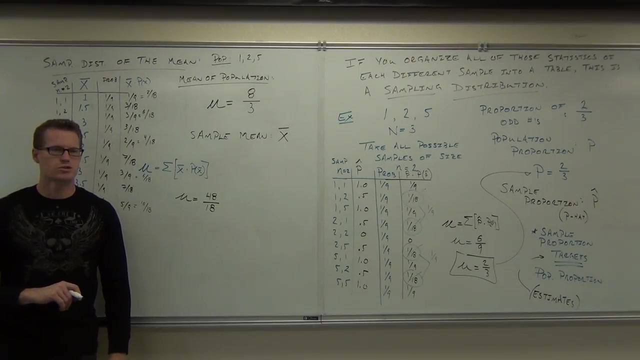 48, so if I add them all up, I get 48 over 18.. Can you reduce 48 over 18?? What goes into both numbers? Six goes in. This gives you eight over 18.. If you add up this column of numbers, 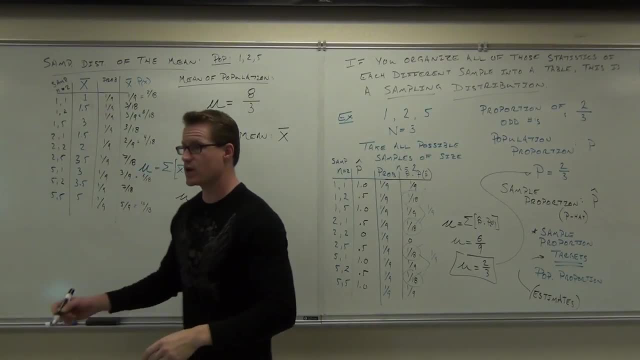 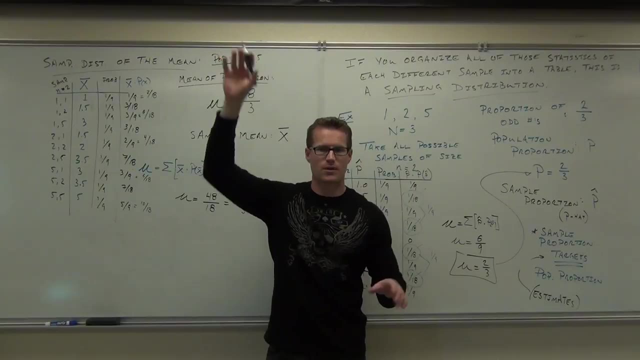 use a calculator if you're not very good at fractions- which hopefully you are good at fractions- but if you're not, add up all those numbers, reduce it, you're gonna get eight-thirds or 2.66666 forever, which I don't feel okay with that so far. 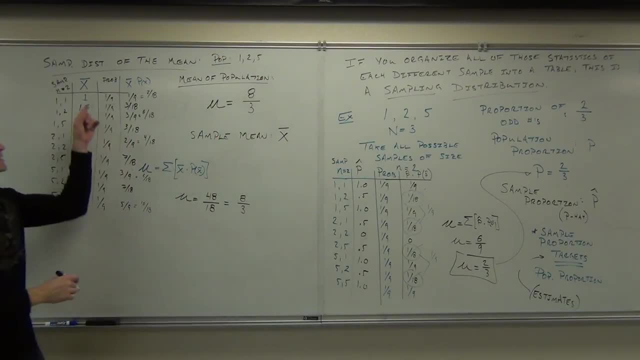 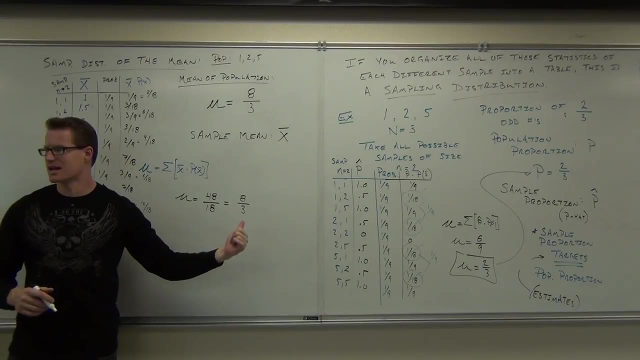 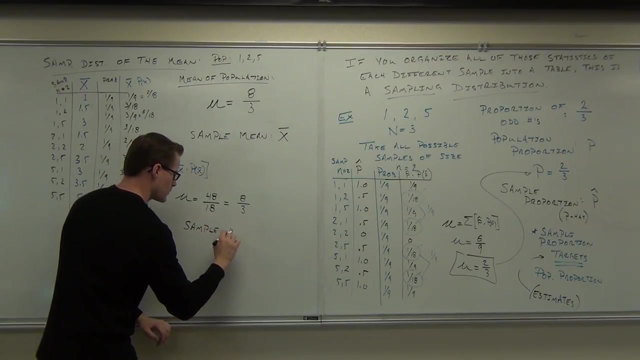 So what happened, Were each of these sample means the same as our population mean? No, but when I averaged them, yeah, it's exactly the same. What this says for us is that sample mean targets, or in other words, estimates, population. 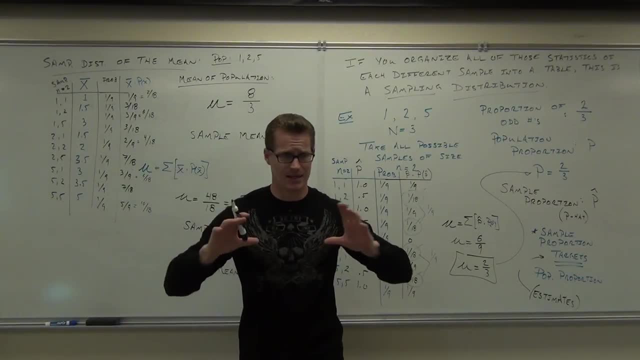 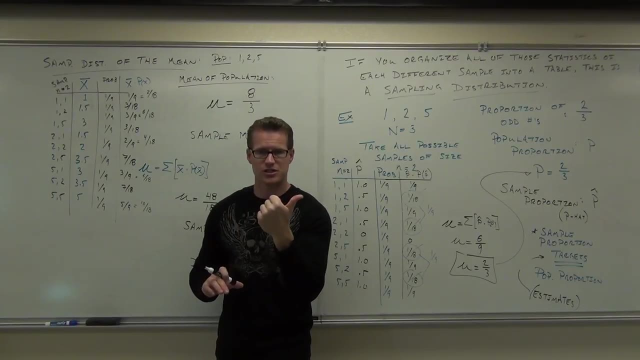 So so far we know two things. We know that here's basically the underlying concept for this section is this: Proportion, sample proportion will be a good estimator for population proportion. Sample mean will be a good estimator for population mean. That's all this whole section says. 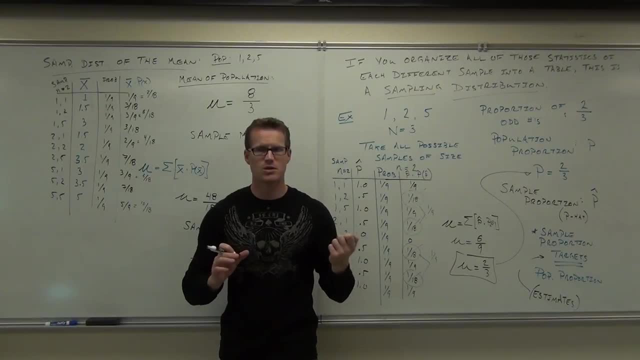 There's one more: Sample variance will ultimately be a good estimator for population variance. The problem is standard deviation, which we need. Standard deviation is actually not a great estimator for population standard deviation. It systematically underestimates it, And so we're gonna have to fix that. 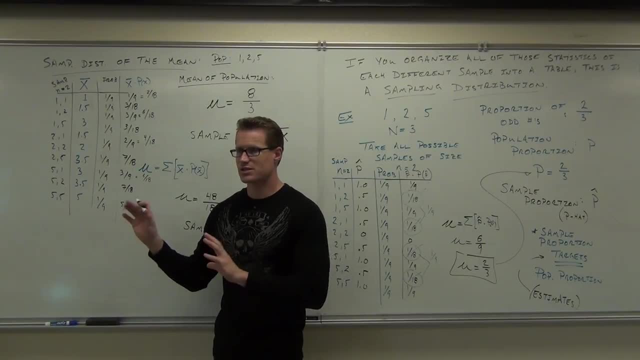 but it's gonna be close enough for us, Do you understand? So our section about sampling distributions was simply: you should know what a sampling distribution is. It's this concept, And then if we average them, we're gonna have to fix it. 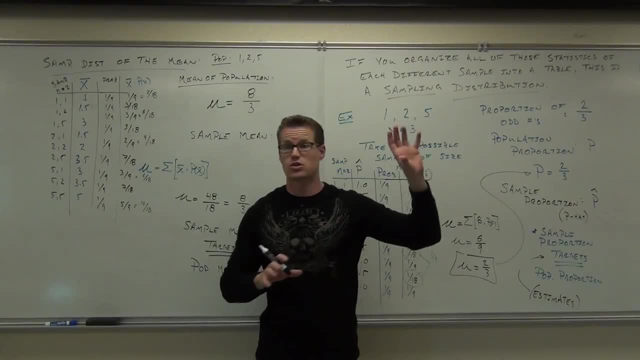 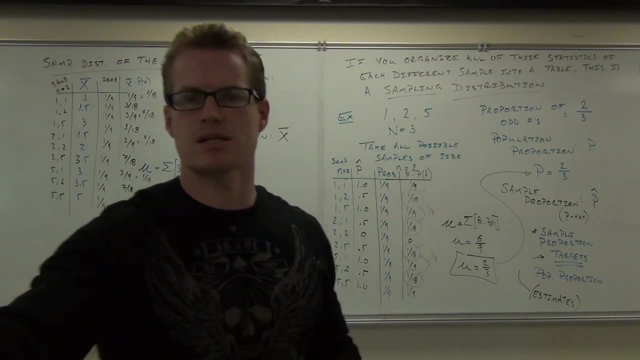 But if we average them together, the average of those statistics will give us or target or estimate the population parameter. I mean, we feel okay about our section here. Good, we'll wrap this up next time.